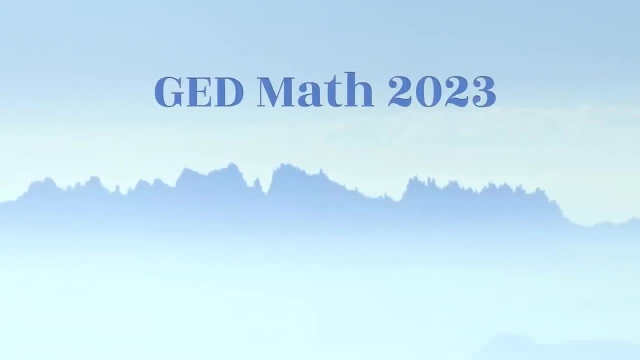 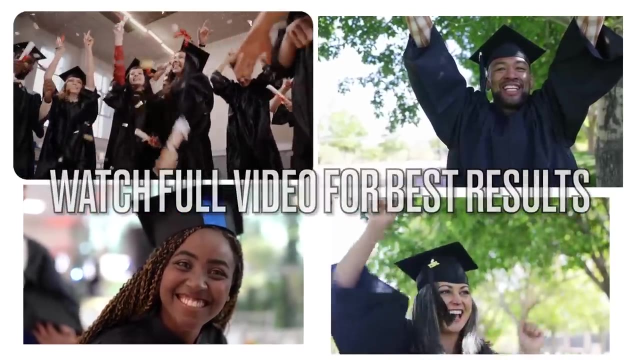 Welcome to the GED Math 2023 Test Preparation video from UltimateGEDcom. We are so excited to help you pass your GED this year. In this video, we'll be looking at how to easily solve 100 of the most important GED math questions. 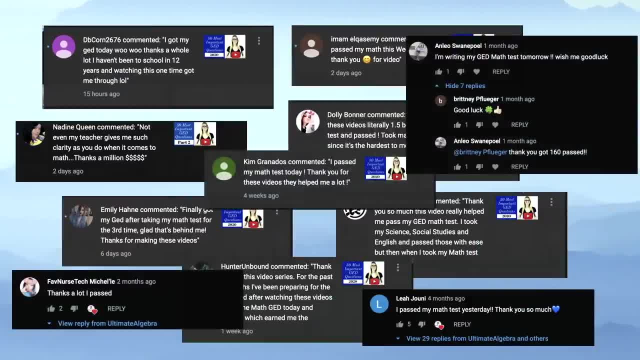 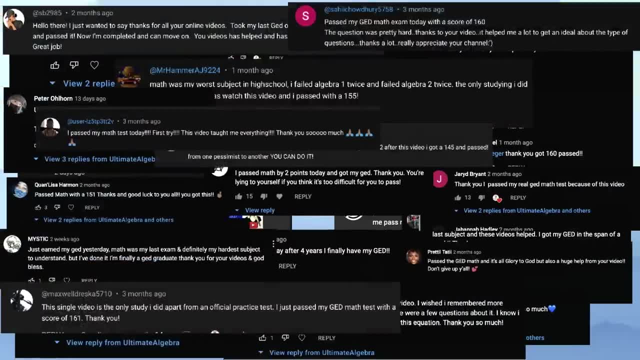 From experience of helping thousands of test takers to pass the GED with ease, we've noticed that the best way, by a far margin, to prepare for the GED is to use standard GED test questions. so let's dive right in Question 1. 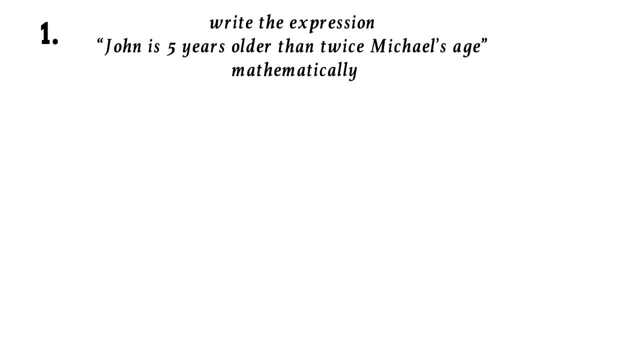 We are writing the expression. John is 5 years older than twice Michael's age mathematically. Let's write the expression here so we can easily work with it. Translation of expression is very common on the GED. We will just solve this question and add a link in the description. 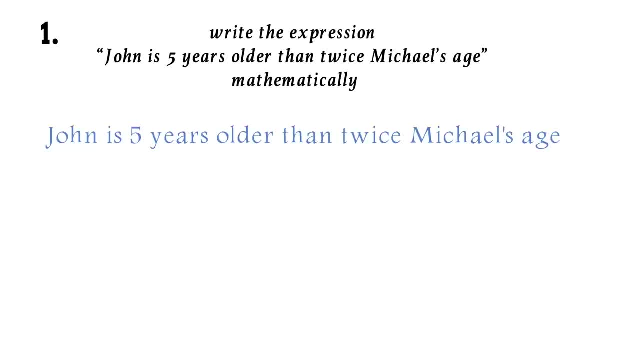 where you can get more information to master it. Please check it out. We can represent John with J and Michael with M. J and M is in mathematics means equal to 5 years older than is the same as 5+. When you see words like bigger than, faster than, more than, and so on, they mean addition. 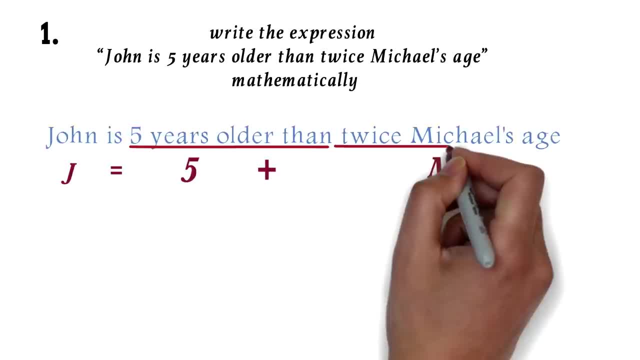 We know that twice means 2 times. Therefore, twice Michael's age is the same as 2 times M. 2 times M can be simply written as 2M, So we have J equals 5 plus 2M as our answer. 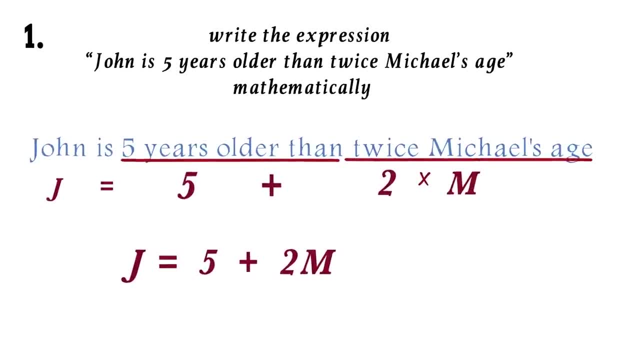 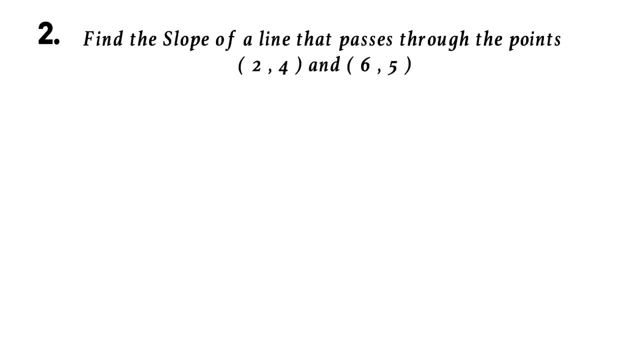 This is pretty straightforward forward. Let's look at our next question, Question 2.. Find the slope of a line that passes through the points 2, 4 and 6, 5. Finding slopes is another important topic on the GED. 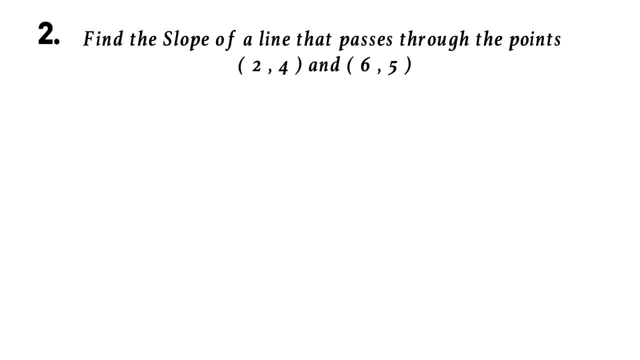 Here we will learn how to find the slope given two points. To find the slope of a line given two points, we will use the slope. formula n equals y2-y1 over x2-x1.. Formulas are given on the GED, so don't worry too much about it. Of course, memorizing it can save you some time. 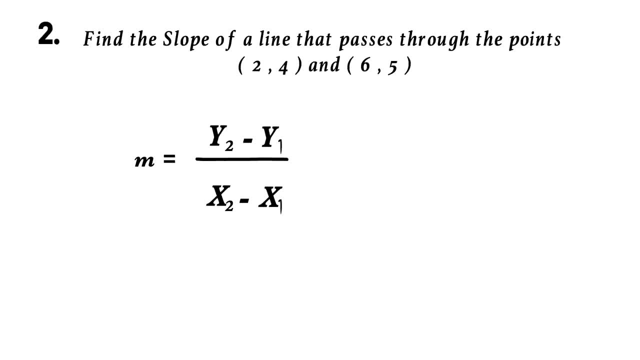 on the test. Please note that you can call any of the point 1 or 2.. I'm choosing this as point 1 and this as point 2.. We know that when you have a point, the first value is your x and the second. 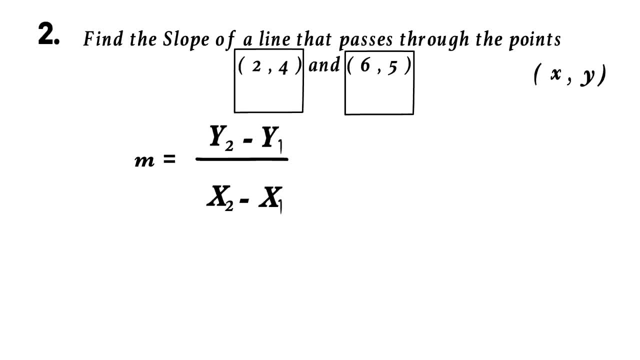 value is your 0. y. Since we are calling this point 1, we will have x1, y1 here. Same thing for this. Since we are calling this our point 2, we can call this x2, y2.. We just put the values into the. 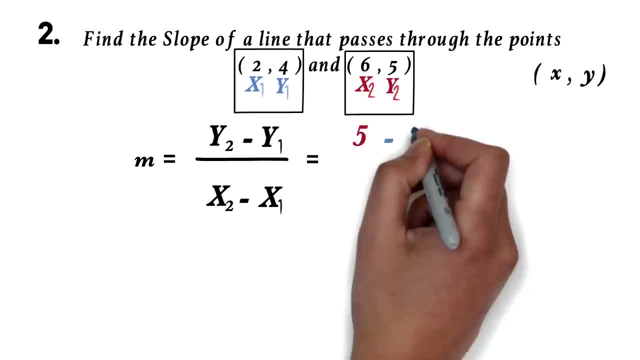 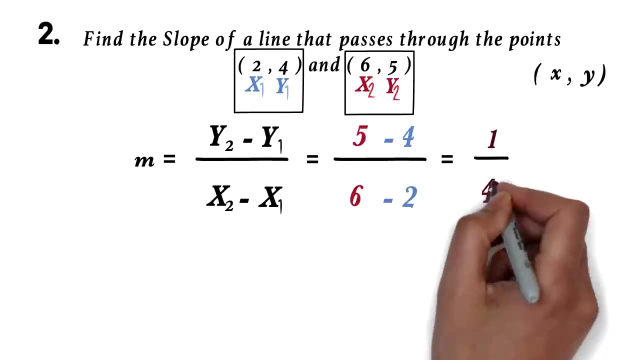 formula: We have 5, which is y2, minus 4, which is y1, divided by 6, which is x2 minus 2, which is x1.. We simplify: 5 minus 4 is 1, over 6 minus 2, which is 4.. So the slope is 1 over. 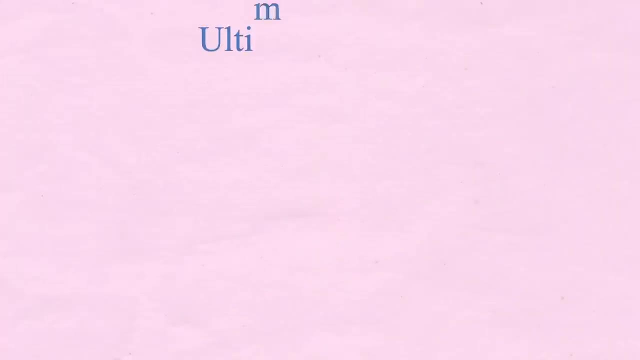 4.. Before we look at our next question, we want you to know that we have a lot of resources at ultimategedcom to help you pass the GED. We have more free videos, A complete GED math course. This is a step-by-step course from the absolute beginning to advanced. 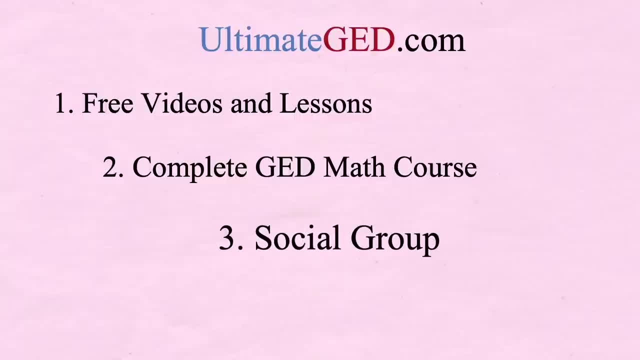 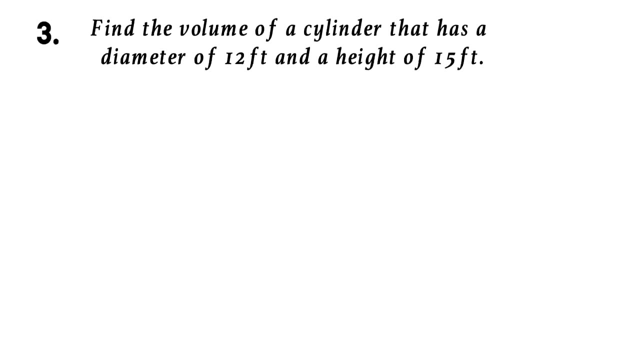 We have a social group. You can talk to people that have taken the GED or are working on taking the GED. Get more at ultimategedcom and pass the GED with ease. Question 3. Find the volume of a cylinder that has a diameter of 12 feet and a height of 15 feet- A lot of the GED geometry. 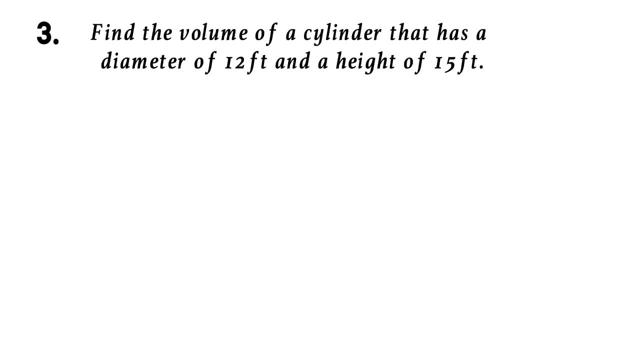 questions are just formula work. All the formulas will be given to you on the GED formula sheet, So no need to memorize it. It is good to be familiar with them, however, because they can increase your speed. The formula for finding the volume of a cylinder is pi r squared h. 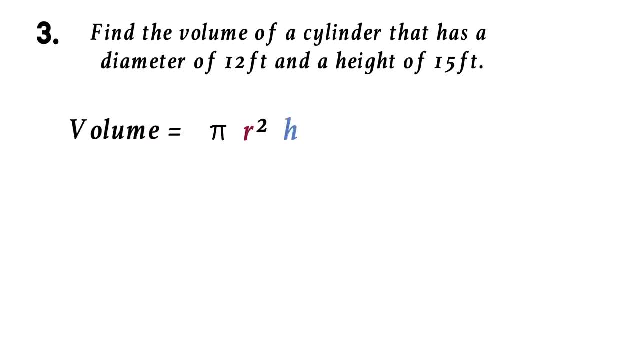 where r is the radius and h is the height. To solve this question, we need to know the value of pi, which is given to us on the GED formula sheet as 3.14.. We need to know the value of height, h, which has been given to us as 15.. Then, finally, we need to know the. 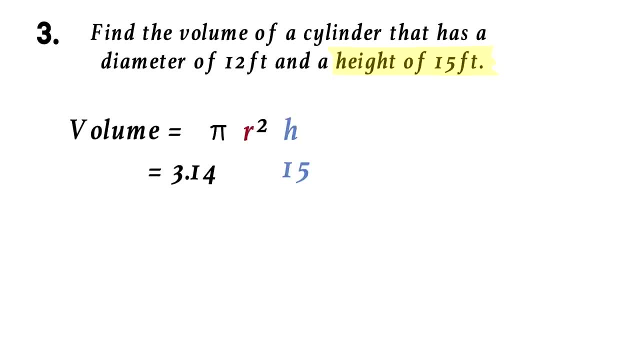 value of radius r, which has not been given to us. We were given the diameter, but we know that the radius is diameter divided by 2.. So we divide 12 by 2 to get 6 as our radius. So we have the volume to be pi, which is 3.14 times 6, squared times 15.. We input this into: 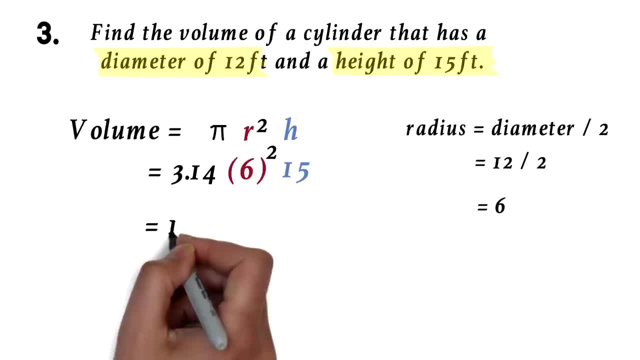 our calculator and get the volume of the cylinder to be 1695.6 feet cubed. So we have the volume to be pi, which is 3.14 times 6 squared times 15.. We input this into our calculator and get the volume of the cylinder to be 1695.6 feet cubed. 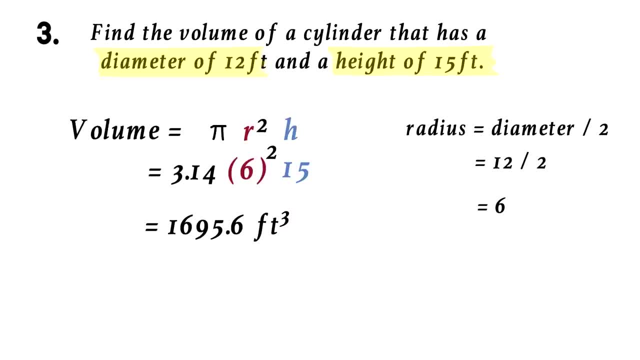 So we have the volume to be pi, which is 3.14 times 6, squared times 15.. We input this into our calculator and get the volume of the cylinder to be 1695.6 feet. cubed feet- cute sometimes. ged geometry questions are not that straightforward. this same question could. 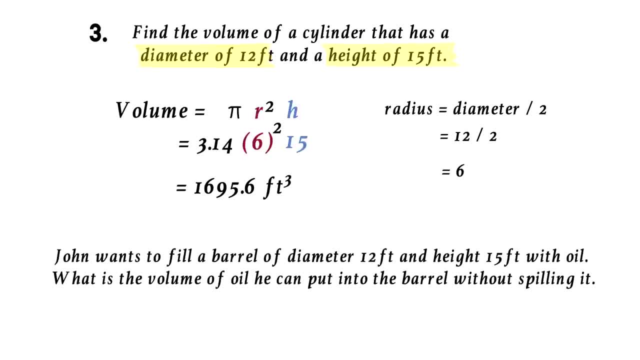 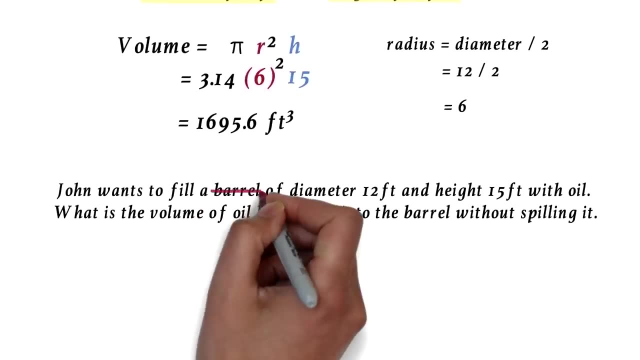 have been worded this way: john wants to fill a barrel of diameter 12 feet and height 15 feet with oil. what is the volume of oil he can put into the barrel without spilling it? this is exactly the same question. first, you have to know that a barrel is a cylinder, so you can replace the word barrel. 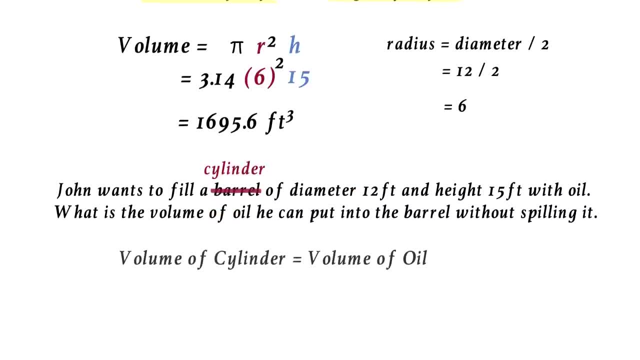 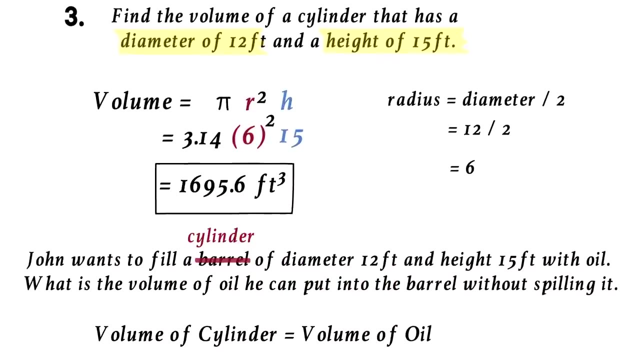 with cylinder. second, you have to know that volume of the cylinder will be the same as the volume of the oil that will be put into it without spilling. once you know these two things, you'll go through the exact same process to get the volume of the oil as one thousand six hundred nine to five point. 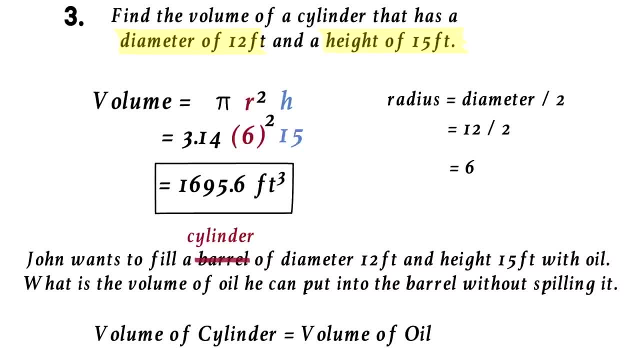 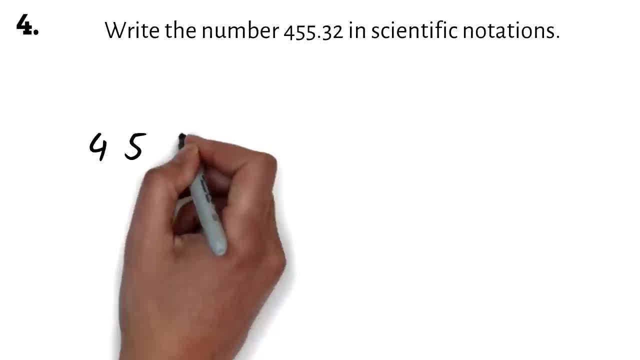 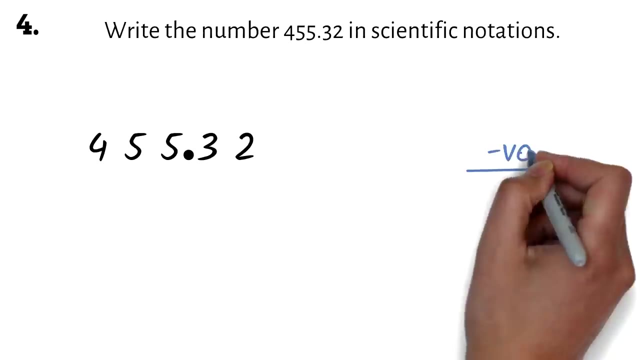 six feet. cute. question four: write the number 455.32 in scientific notations. to write in scientific notations we have to move the decimal behind the first non-zero number. then multiply the new number by 10 exponent the number of times we moved. if we move to the right, then we have a negative exponent. if we move to the left, then we have a. 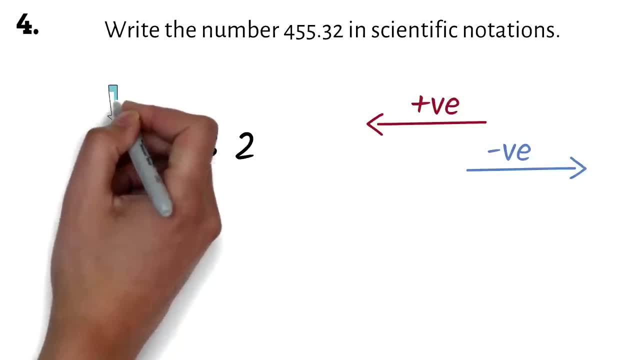 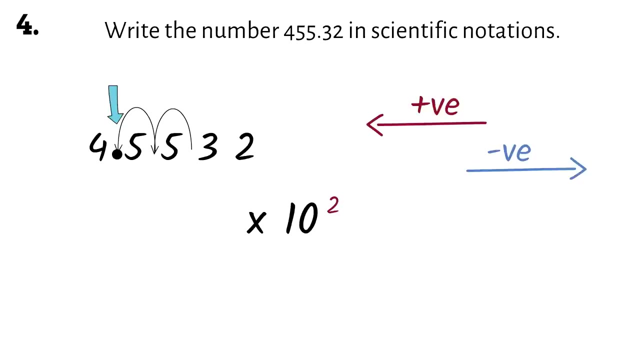 positive exponent. so here we have to move the decimal behind the four, since it's the first non-zero number. we start from where the decimal point is and we move one, two points to the left. so this will be times ten to the power positive two, since we move to the left. 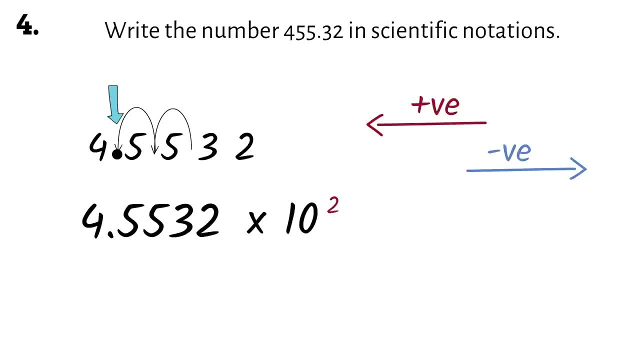 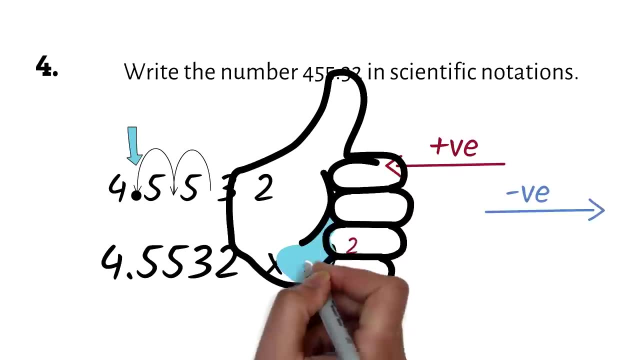 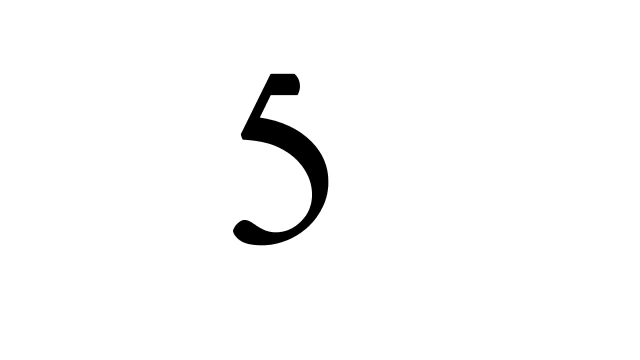 so our final answer is four point five, five, three, two times ten to the power two. please encourage us to post more videos by liking this video and sharing. if we don't know you like it, there'll be no reason to post more, thank you. question five: a singer borrows five thousand dollars for two years. 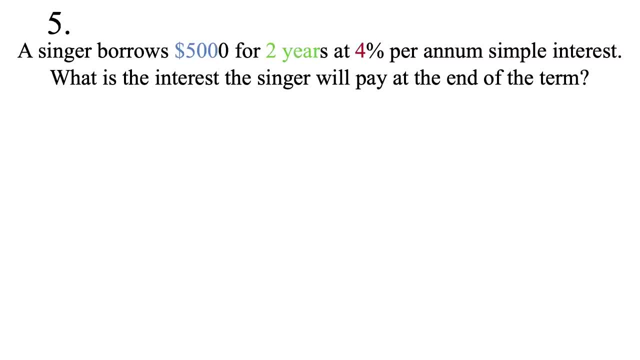 at four percent per annum. simple interest. what is the interest the singer will pay at the end of the term? simple interest questions are basically formula work and the formula will be given to you on the ged formula sheet. symbol interest equals the principle times the rate, times the time. we just substitute our values. 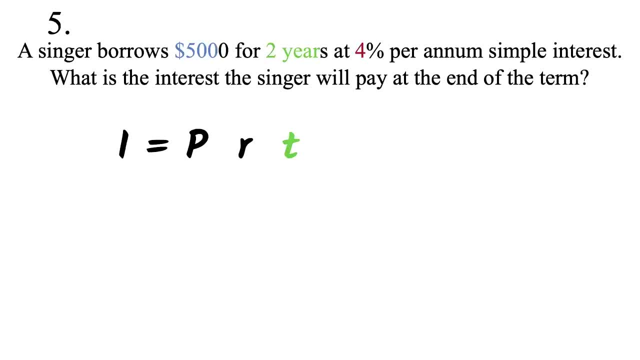 into the formula and solve here. the principle is five thousand dollars, the rate is four percent. we convert it to the decimal form: four percent is four percent when the value is less than one percent. 4 divided by 100. This is the same as 0.04.. So we multiply this by 0.04.. The time is 2 years. 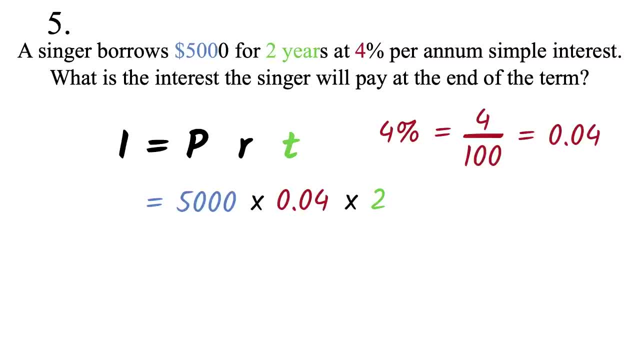 so we have times 2.. We compute this on the calculator 5000 times 0.04 times 2 to get 400.. So the interest the singer will pay is $400.. Hope you've noticed that we keep mentioning the GED. 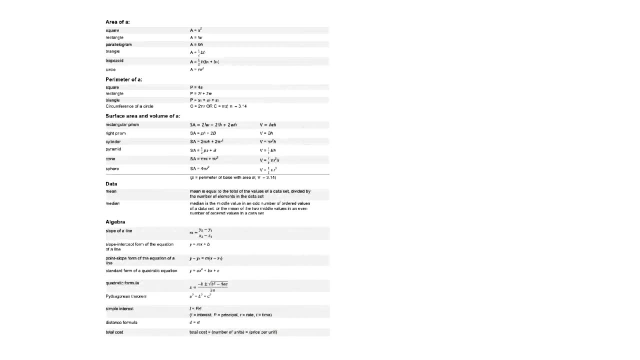 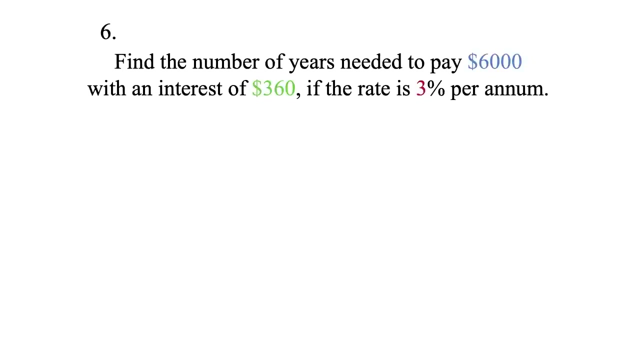 formula sheet. It's something you have to be familiar with before taking the test. You can check ultimategedcom for more on that Question 6.. Find the number of years needed to pay $6,000 with an interest of $360, if the interest. 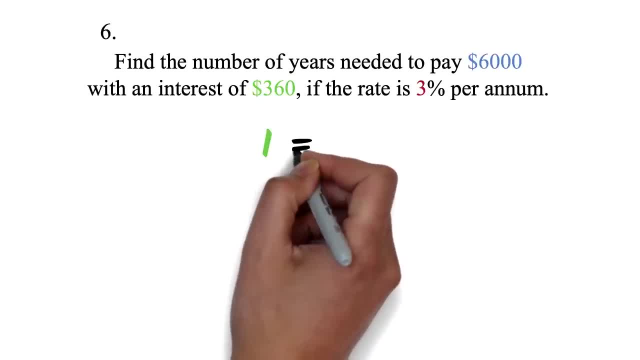 rate is 3% per annum. For every formula you are given, you can be asked to find any of the values in that formula. You can be asked to find the number of years needed to pay $6,000.. You can be asked to find the rate, principal, interest or time. Here we are supposed to find. 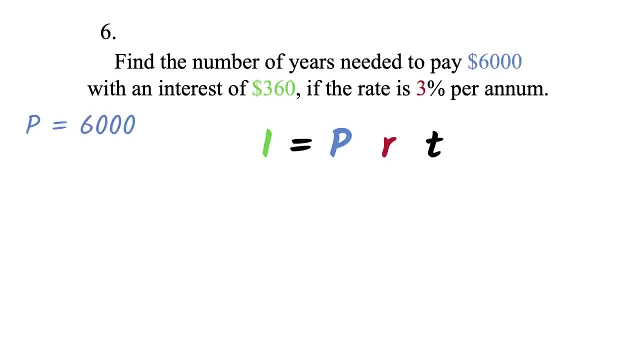 time We know, our principal is $6,000.. Our interest is $360. And our rate is 0.03.. We divided the 3 by 100 to get the decimal form of 3%. Simple interest equals the principal times the rate, times the time. as we saw in the previous question, We have 360,. 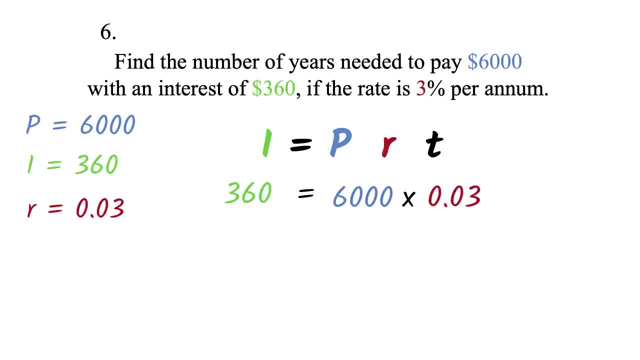 equals 6,000 times 0.03. times t, We solve for t. Since the 6,000 times 0.03 are multiplying, we can divide both sides by it. This will cancel out. We can now compute this side with our. 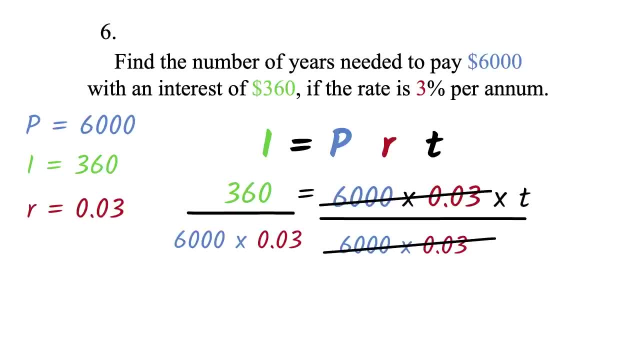 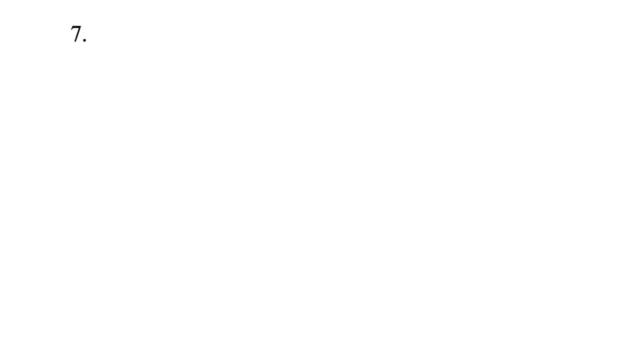 calculator: 360 divided by 6,000 times 0.03.. This will give us t equals 2, meaning the time is 2 years. Question 7.. We are supposed to calculate 3 exponent 10 times 3 exponent, 5, all over 3. 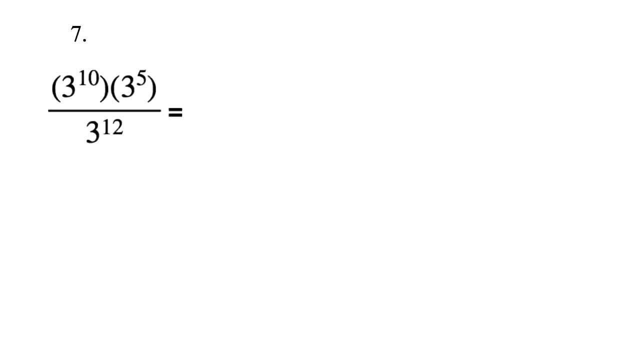 exponent 12 without using a calculator. If you have two numbers multiplying and the bases are the same, you can just add the exponents. Example: let's look at 2 exponent 3 times 2 exponent 4.. Because they both have the same bases, which is 2 in this case, we can just 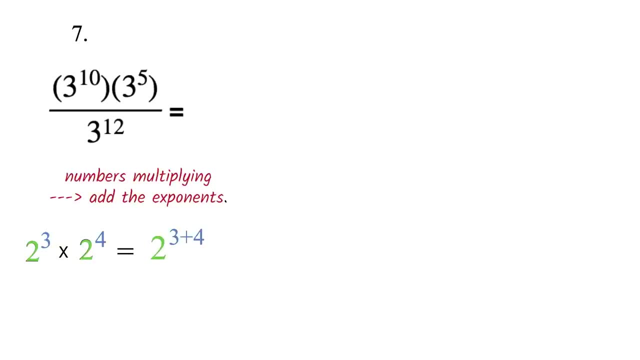 add the exponents, So this will be 2 exponent 3 plus 4, which is 2 exponent 7.. Now if you have a number being divided by another number with the same base, then you can simply subtract the exponents. 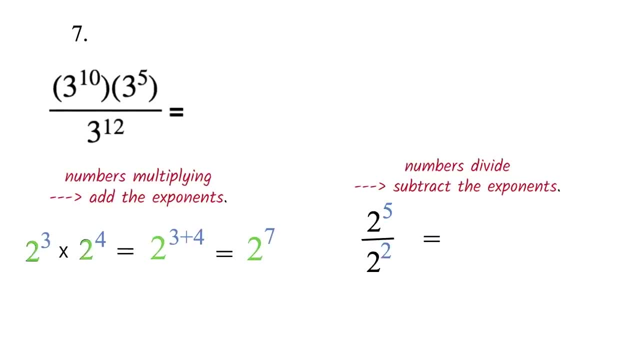 So 2 exponent 5 divided by 2 exponent 2 will be 2 exponent 5 minus 2, which is 2 exponent 3.. Please, these two rules applies only when the bases are the same. It will not work for. 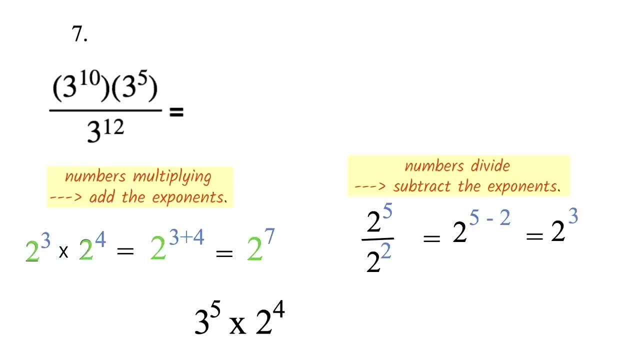 3 exponent. 5 times 2 exponent. 4. The bases are different. One is 3 and the other is 2. Even if the exponents are the same and the bases are different, it won't work. Example: 3 exponent- 5 times 2 exponent. 5. The exponents being the same is irrelevant. 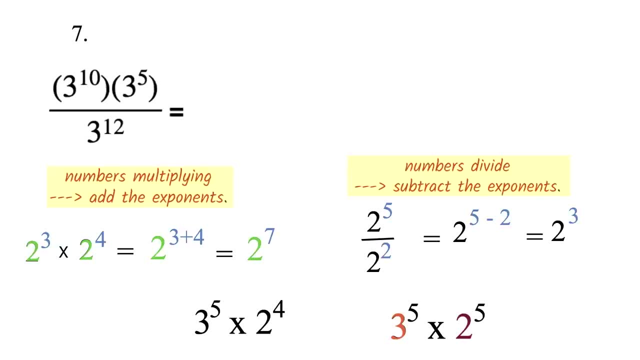 The bases are not the same so we can't use this So for our question. we can see that they all have the base of 3, so the rules can apply. So 3 exponent 10 is multiplying 3 exponent 5.. 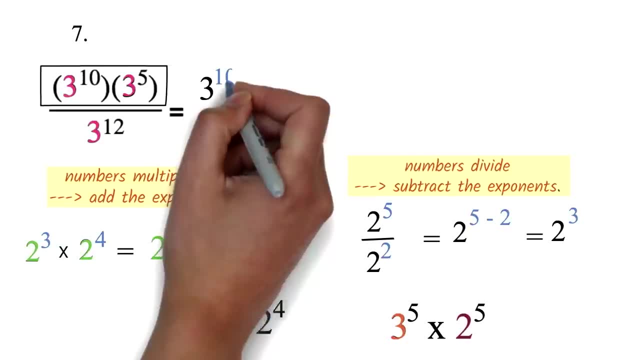 So we can add the exponents to get 3 exponent 10 plus 5. This will give us 3 exponent 15.. This 3 exponent 15 is being divided by 3 exponent 12.. We know that when terms with the same base divide, we can simply subtract their exponent. 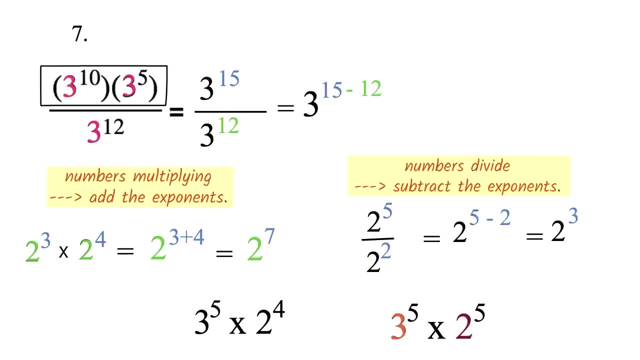 So we have 3 exponent 15 minus 12, which is 3 exponent 3.. So this is the answer. They could have required you to further simplify the 3 exponent 3.. Which will be 3 times 3 times 3.. 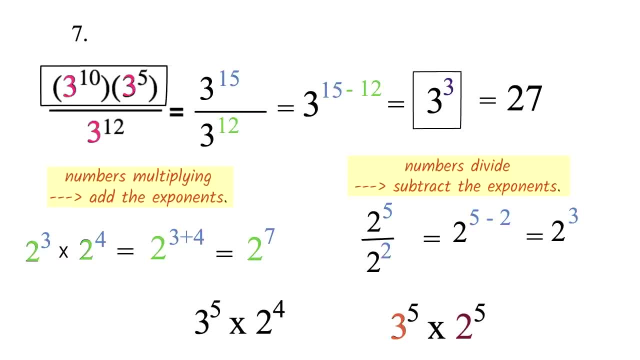 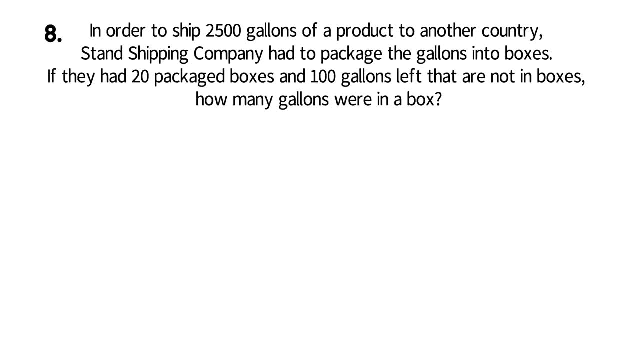 This will be 27.. Question 8. In order to ship 2,500 gallons of a product to another country, Stan's shipping company had to package the gallons into boxes. If they had 20 packaged boxes and 100 gallons left that are not in boxes, how many gallons? 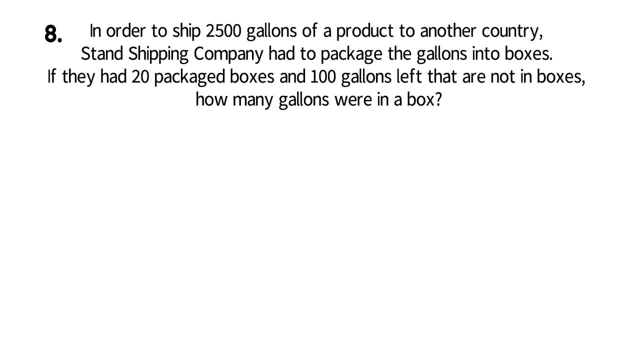 were in a box. This kind of two-step equation word problem Is very common on the GED. We are first going to solve it in details for teaching purpose. Then I'll show you how you can solve it in less than 10 seconds on an actual GED test. 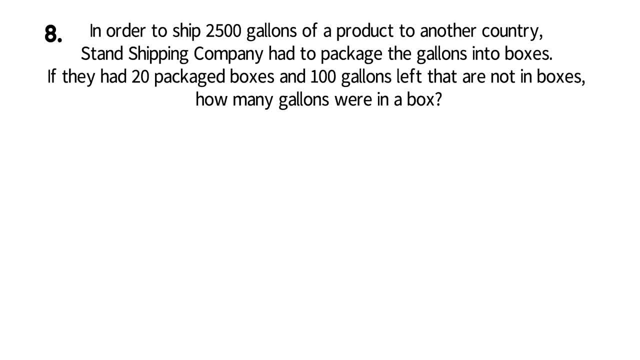 You have three values in these type of questions. Let's write them down. We have 2,500 gallons, We have 20 boxes And finally we have 100 gallons. The 2,500 gallons represents the total. So we have. 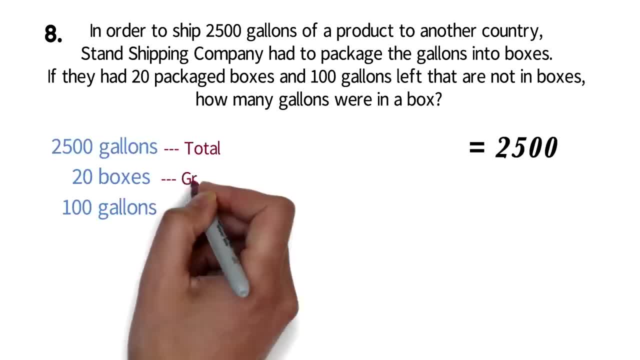 The 20 boxes is what I call the group. The gallons have been grouped into boxes. For most questions the group can also be identified as the number that represents something different from the other two numbers. So here 2,500 represents gallons. 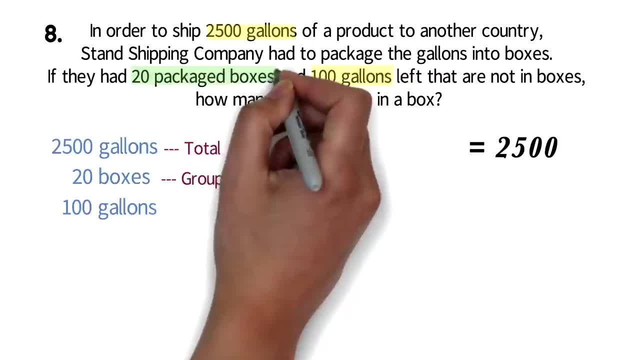 The 100 also represent gallons, But the 20 represent boxes, So the 20 will be the group. The group is the one with the x, So we will have 20x. We can now add the 100 gallons left to the equation and solve for the x in this two-step. 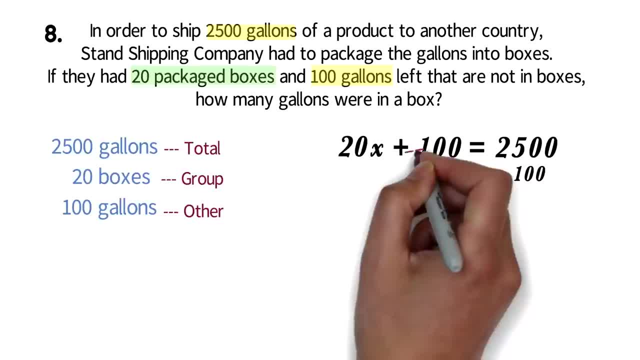 equation: Subtract 100 from both sides, These will cancel out. 2,500 minus 100 will be 2,400.. We now have 20x equals 2,400.. Divide both sides by 20.. The 20 will cancel out. 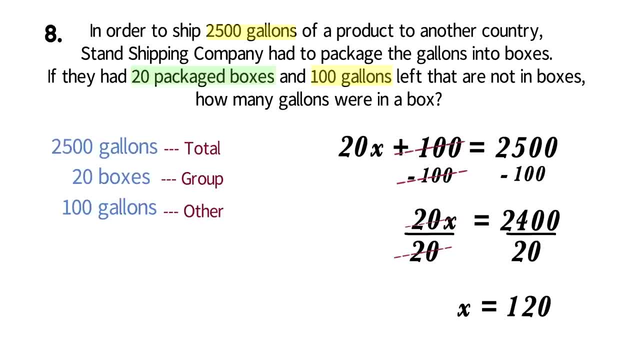 2,400 divided by 20 will be 120.. This means that the 20 will cancel out. 2,400 divided by 20 will be 120. This means there were 120 gallons in each box. The hard part of this question is to be able to pull out the values from the word problem. 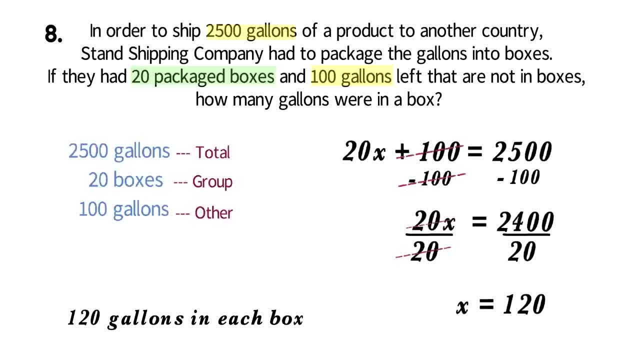 Let's look at how you can speed up solving this question. First, there's absolutely no reason to write this part. if you know what you're doing, You can go straight to writing your two-step equations. We have our group 20x, our other plus 100, and our total 2,500.. 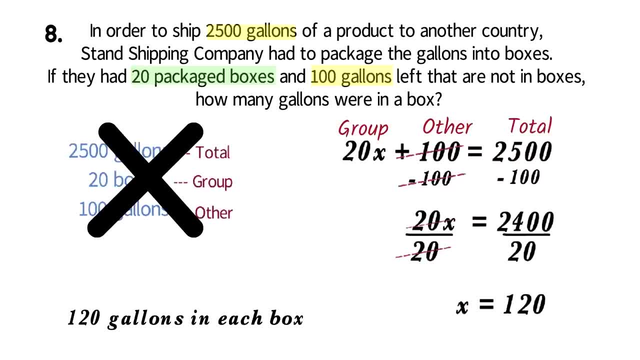 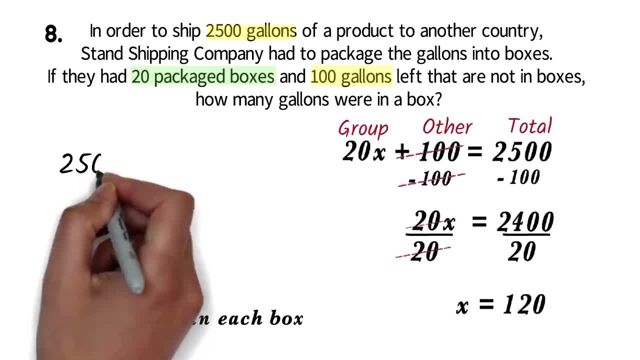 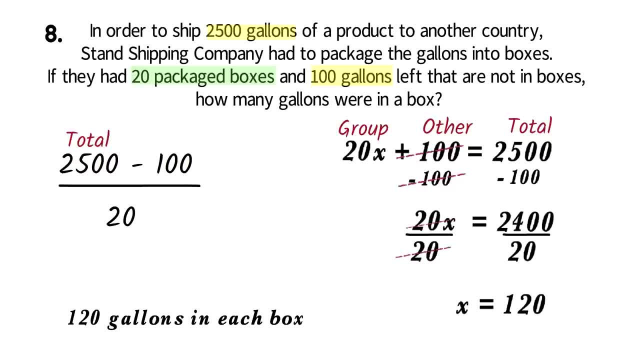 100 divided by 20 on your calculator to get 120. We did the total minus other divided by the group. A big caution when using fast methods is to note that they are very specific to specific questions and little twists to the question can let you get it wrong. 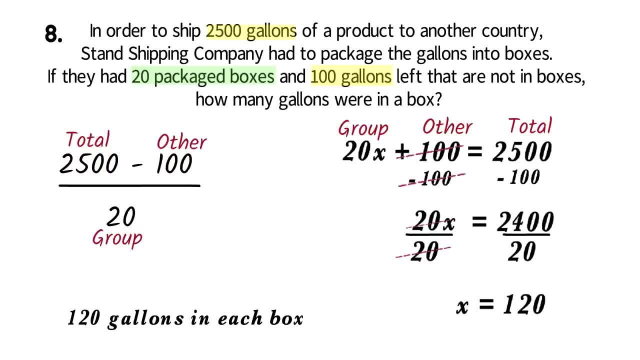 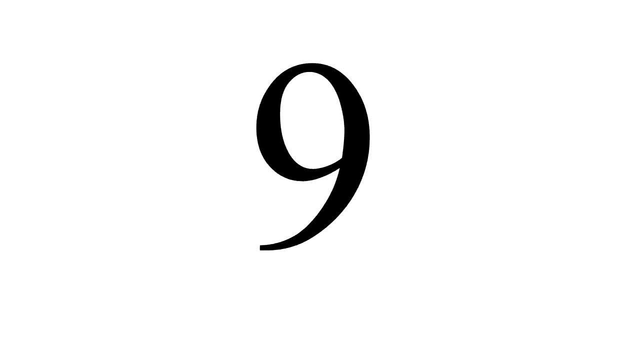 So, when in doubt, use the longer methods. If you have any questions, please let us know in the comments. Thank you. Question 9. Find the slope of the line. The slope of a line is the change in y over the change in x. 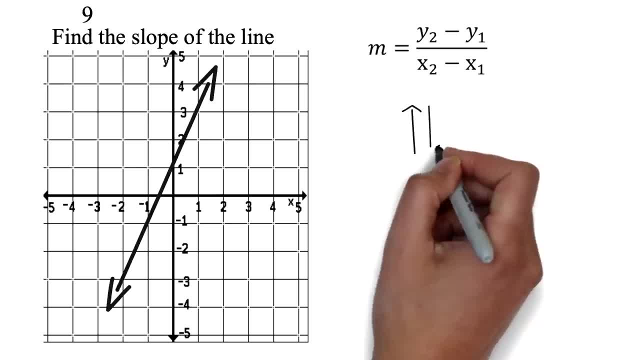 The change in y simply means how many points you are going up or down. If you are going up, then you have a positive change. if you are going down, then you have a negative change. The change in x simply means how many points you are going to the right or left. 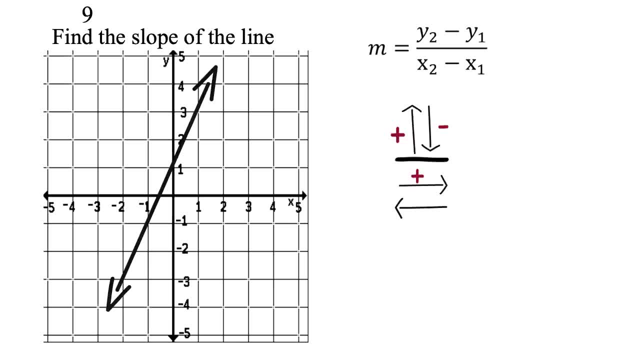 If you are going to the right, then you have a positive change. If you are going to the left, then you have a negative change. Take a moment and let this sink in. It is the basis of most of the things we will be doing with slopes and graphs. 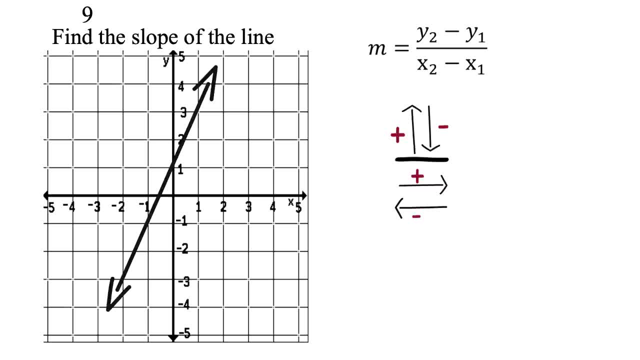 Let's look at our question. Our first step will be to choose any two points on the line. I am choosing these two points. Let me call them A and B. You can choose any two points on the line. However, it is important to choose points that will make your work easier. 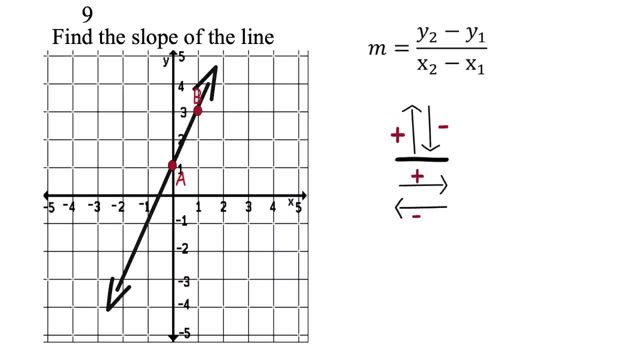 Choose points whose X and Y values can be easily determined. Normally, points at the corners are best. Any of these points would have worked well also. Now to find the slope. all we are doing is moving from one point of the line to the other. 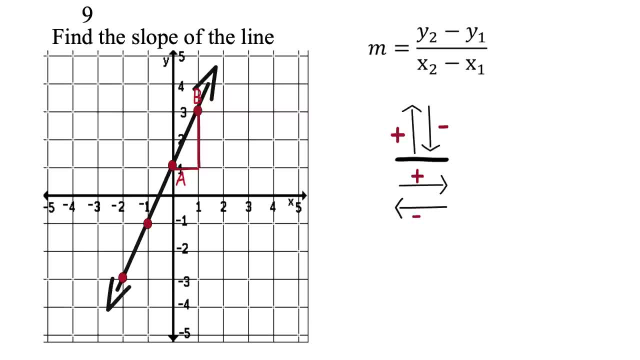 on the slope triangle. Let's move from B to A. We moved down two points. Notice moving down is negative. So we have negative two here. Then we will move to the left. one to get to A. Notice that moving to the left is negative. 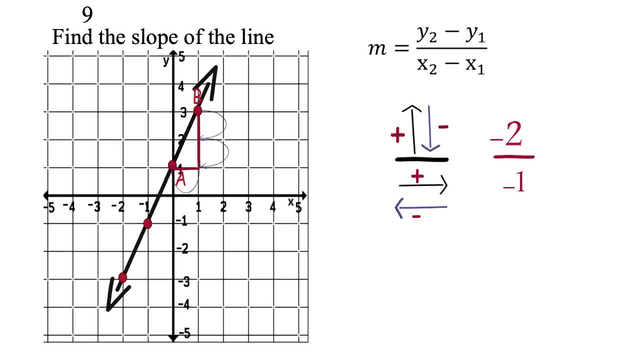 We have negative one here, Negative two over negative one is simply two, So our slope is two. We could have also moved from A to B. Let's look at it. We have our slope triangle here. We move two points up. Moving up is positive. 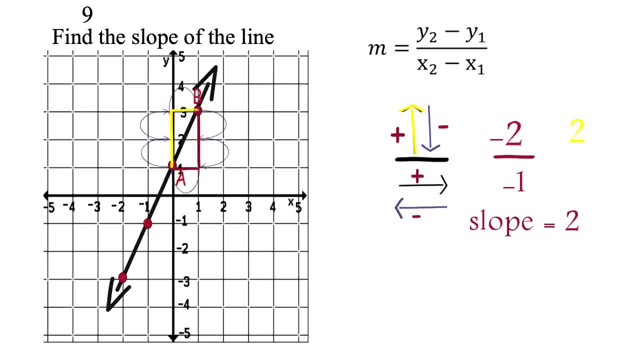 So we have two. Then we will move to the right one. So we have two. Moving to the right is positive, So we have one. Two over one is the same as two. We notice that we got the same answer. There are other things you can do, but I don't want to get you confused with that. 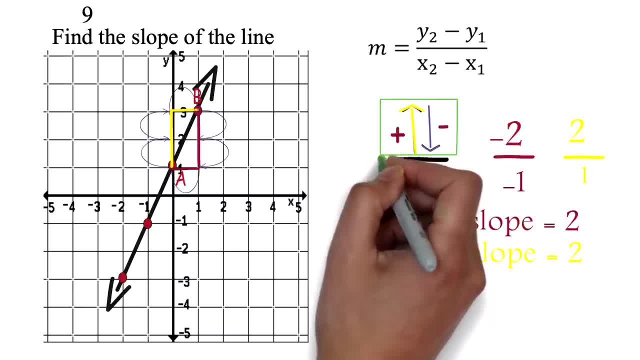 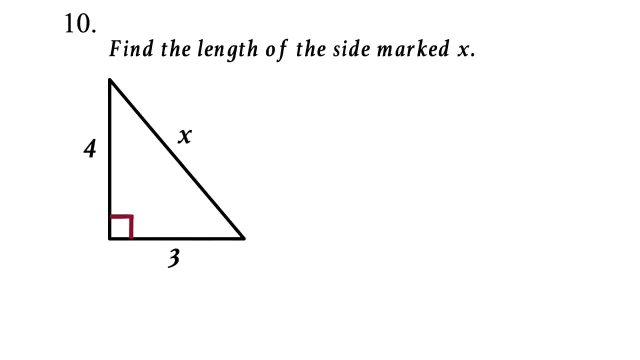 Notice that our first movement is always change in Y, that is, moving up or down. Then our second movement is change in X, That is moving left or right. Question 10. Find the length of the side marked X. When you see this mark on a triangle, it means it's a right triangle. 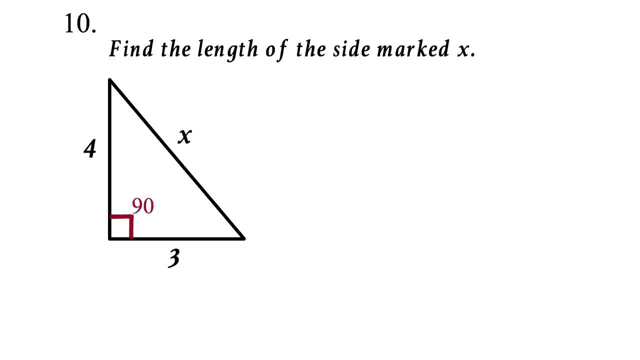 Right triangles have this angle being 90 degrees. When you have a right triangle, you can use the Pythagoras theorem to find the sides. This formula will be given to you on the GED Hypotenuse, which is the long side. squared equals a squared plus b squared. 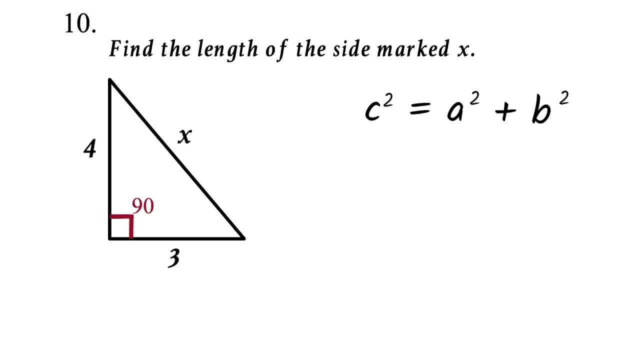 Where a and b are the two other sides. Here the long side, or hypotenuse, is what we are finding. So we have: x squared equals 4 squared plus 3 squared. 4 squared is 16 and 3 squared is 9.. 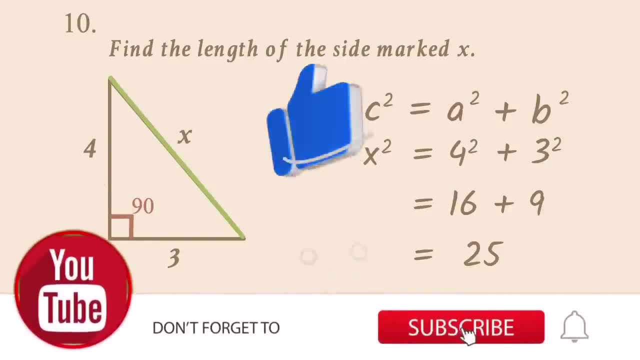 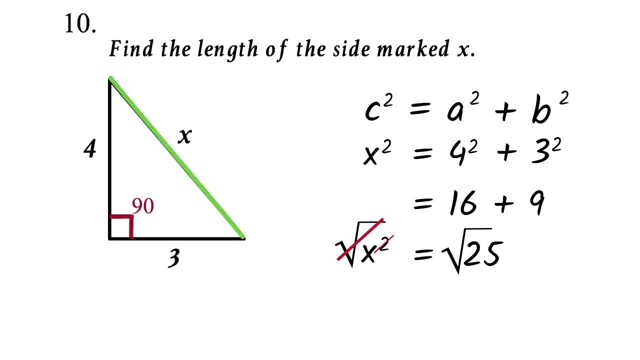 We add them: 16 plus 9 is 25.. To find x, we will find the square root of both sides. This will cancel out. Square root of 25 is 5.. Therefore, x equals 5.. Please note that most questions can be converted to word problems. 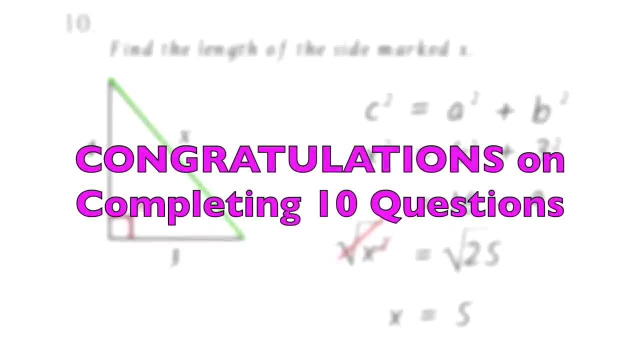 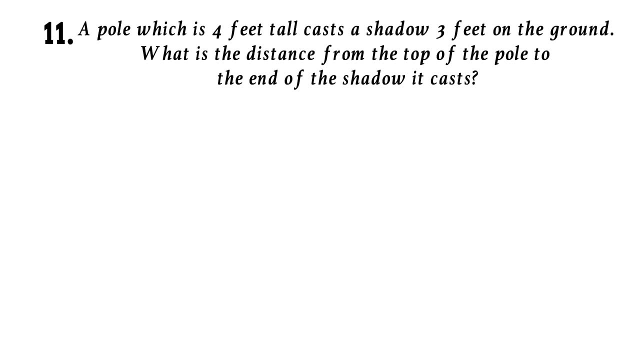 Let's look at a word problem similar to this Question 11.. A pole which is 4 feet tall casts a shadow 3 feet on the ground. What is the distance from the top of the pole to the end of the shadow it casts? 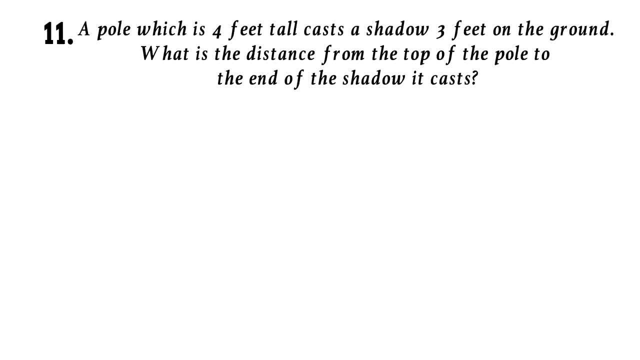 When it comes to solving geometry word problems, your diagram is one of the most important things. Let's get a diagram. So this is our pole, which is 4 feet. This is the shadow it casts, which is 4 feet. We are supposed to find the distance from the top of the pole to the end of the shadow. 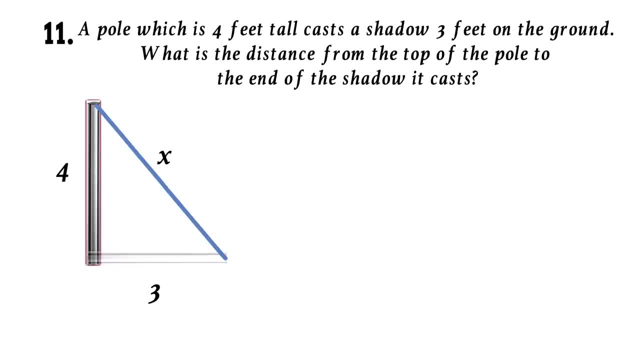 Let's call this x. We see that we have formed a right triangle. Now this question is just like the previous. You can try it out yourself. We can use the Pythagoras theorem to solve it. This formula will be given to you on the GED. 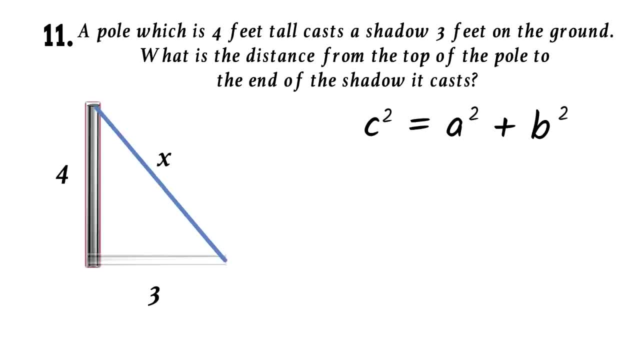 The hypotenuse, which is the long side. squared equals a squared plus b squared. Here we have a long side which is a squared plus b squared. Here we have a long side which is a squared plus b squared. 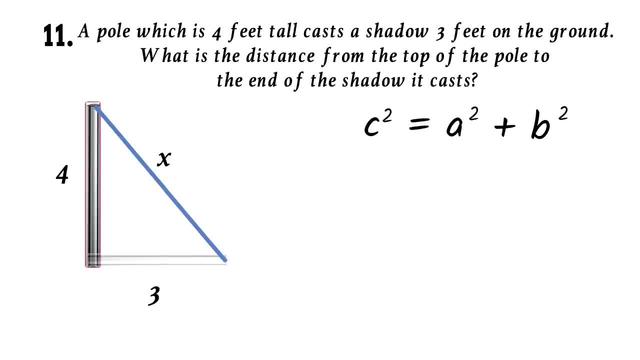 Here we have a long side, which is a squared plus b squared. The long side, or hypotenuse, is what we are finding. So we have: x squared equals 4 squared plus 3 squared. 4 squared is 16, and 3 squared is 9.. 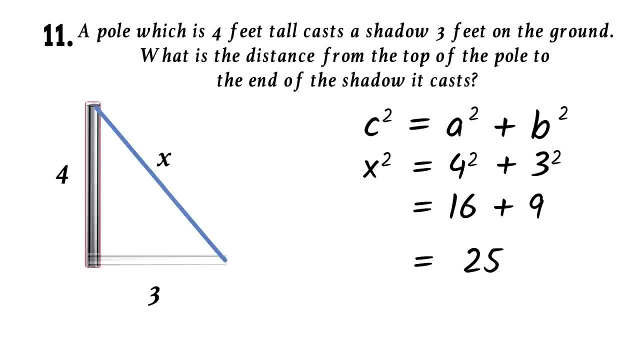 We add them, 16 plus 9 is 25.. To find x, we will find the square root of both sides. This will cancel out. Square root of 25 is 5.. Therefore x equals 5.. So the distance from the top of the pole to the end of the shadow is 5.. 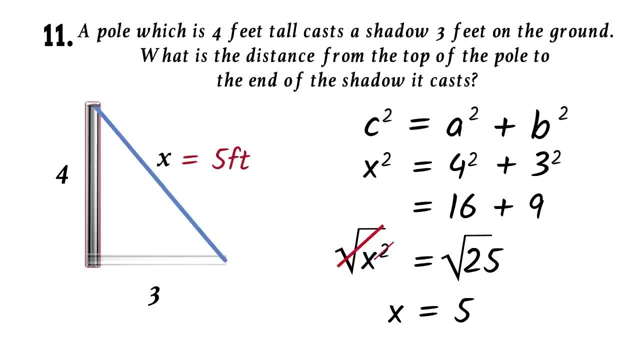 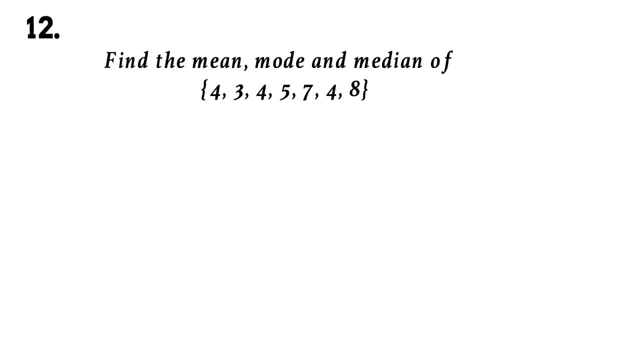 So the distance from the top of the pole to the end of the shadow is 5.. This is 5 feet. Question 12. Find the mean mode and median of 4,, 3,, 4,, 5,, 7,, 4, and 8.. 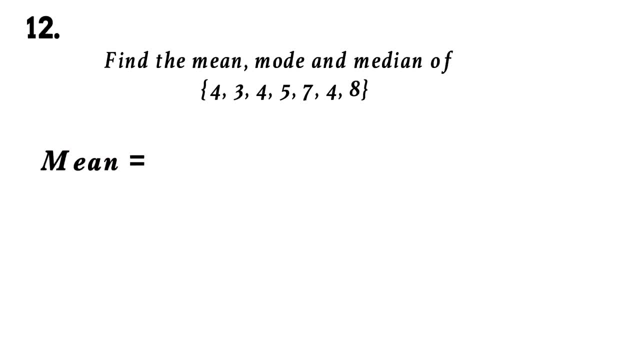 Finding the mean is the same as finding the average. We will add all the values and divide it by the number of values. There are 7 values here, So we will have 4 plus 3 plus 4, plus 5 plus 7 plus 4,. 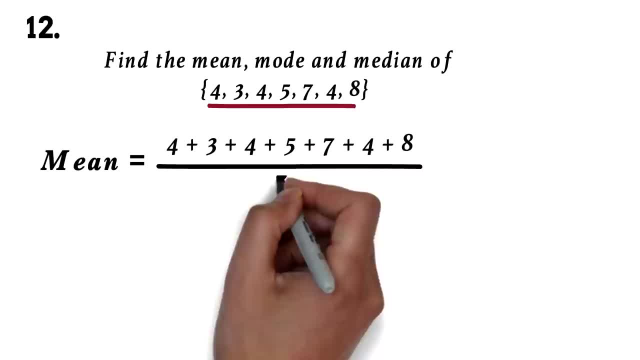 plus 8, divided by the number of values, which we know is 7.. Adding this, we will have 35 over 7.. 35 divided by 7 is 5.. Therefore, the mean is 5.. The mode is the item with the highest frequency. 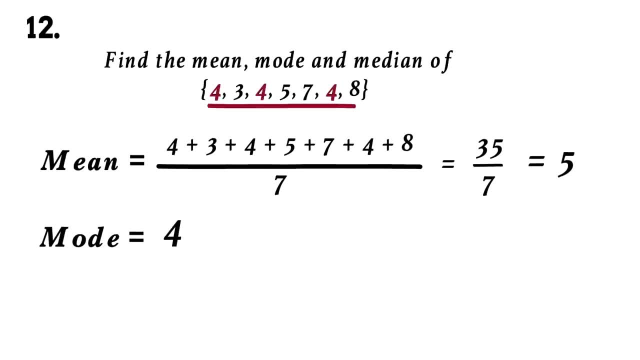 Here there are more 4s than any other number. so 4 is the mode, The median is the middle number. To find the median we first have to arrange the numbers. So we have 3,, 4,, 4,, 4,, 5,, 7, and 8.. 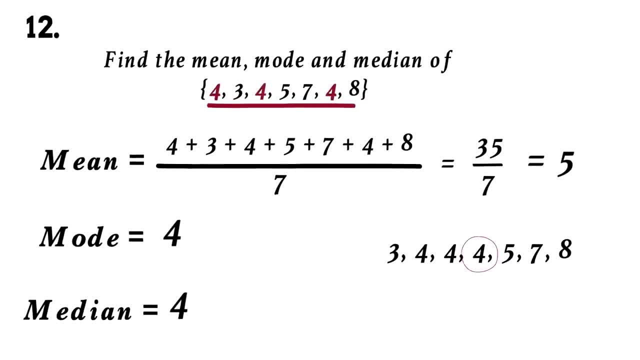 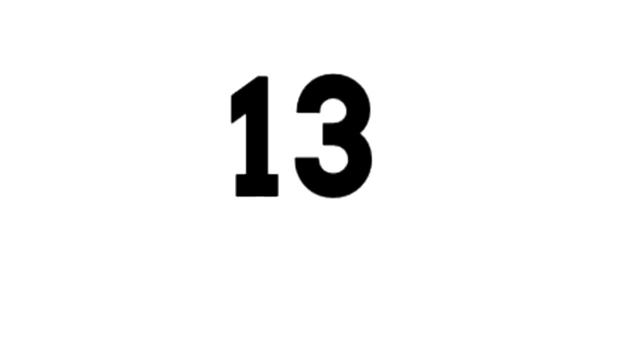 Here the median will be 4.. It's the number in the middle. Please note that if you have an even number of values, you'll add the two middle numbers and divide it by 2.. Please let us know if you have questions on this part. Question 13. In order to graduate. 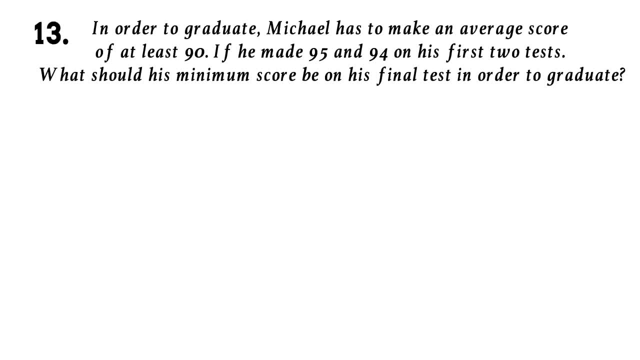 Michael has to make an average score of at least 90. If he made 9 to 5 and 94 on his first two tests, what should his minimum score be in his final test in order to graduate? This is an average or mean question. To find the average, we need to add all the scores divided by the. 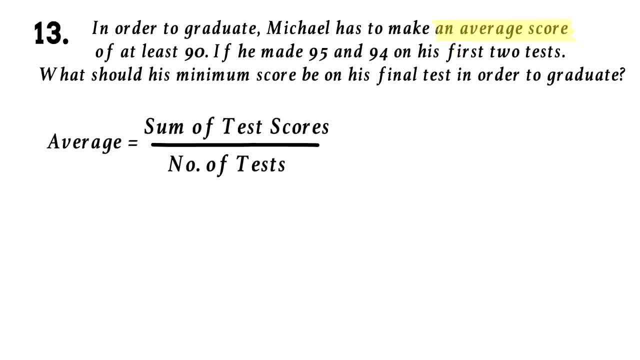 number of tests taken. We've been given the average he must get, which is 90. So we can put it here. Now we also know the number of tests he is taking. He's taken two and there's one more left, So he's taken a total of three tests. So we can put 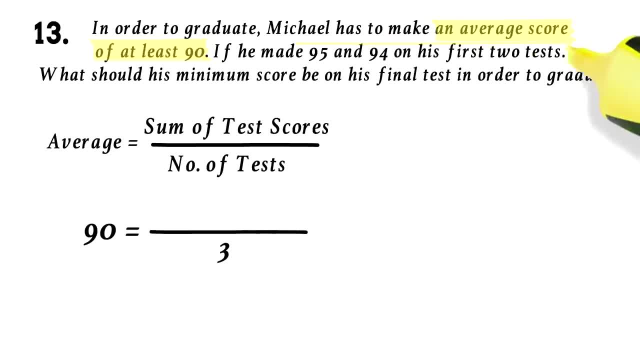 it here. We know what goes at the top is the sum of the tests. Two of them have been given. We have 9 to 5 as the first score, plus 94 as the second score. We don't know the third score, so we will. 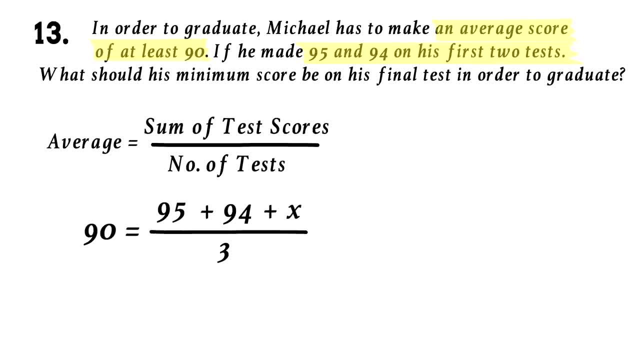 represent it by x and solve for x. Please learn this setup. It's quite common on the GED. Okay, let's solve it. Since the three is dividing, we can multiply both sides by three. This three will cancel out. 90 times three is 270.. Now let's add this: 94 plus 9 to 5 is 189.. We have a one-step. 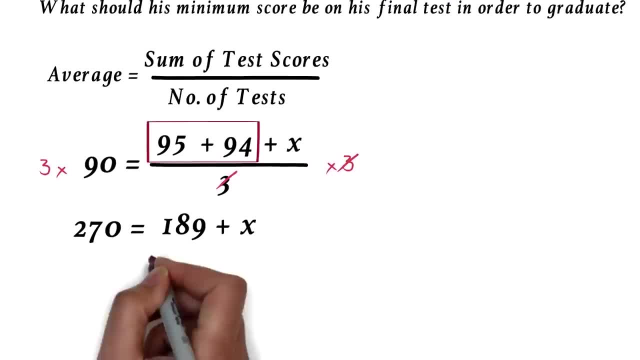 equation. Since the 189 is adding, we can subtract 189 from both sides. This will cancel out. 270 minus 189 is 81. So Michael must get a minimum score of 81 to graduate. There are other ways we could have. 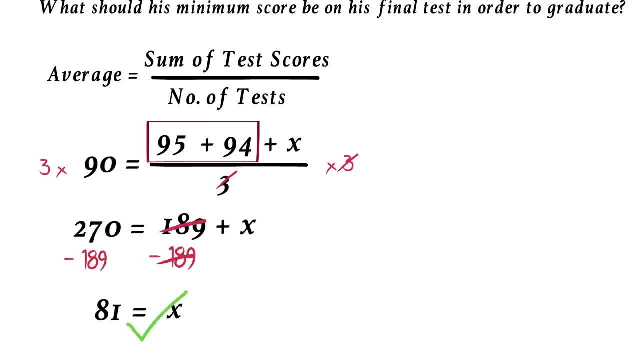 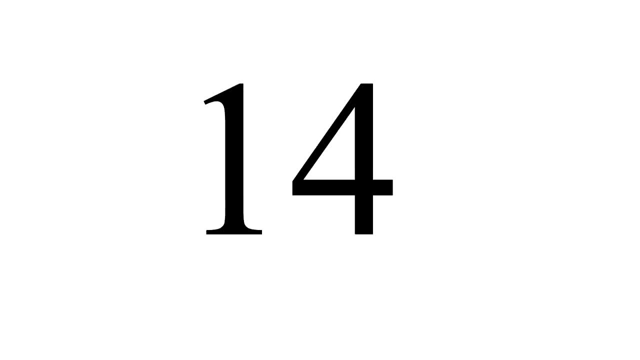 solved this, but we chose this method because it helps you solve any average or mean question, no matter the twist. Question 14. Find the slope and y-intercept of the line. y equals negative 3x plus 5.. Slope questions are now very common on the GED math Almost everyone. 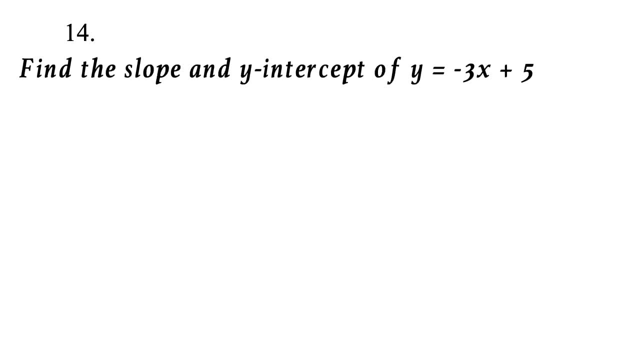 gets something on slope. We've already looked at finding the slope given two points on question two, and finding the slope from a graph on question nine. For this question you'll use the formula for the slope-intercept form of the equation of a line which is y equals mx plus b. This will be given on the GED formula. 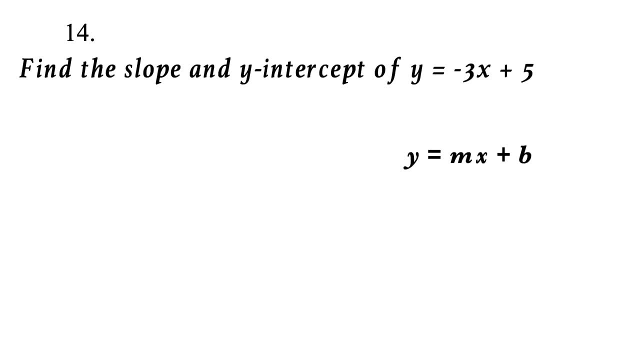 sheet, so you don't have to memorize it, but being familiar with it can help with your speed. In this form, the slope is the m, This is the coefficient of the x, Or simply put, what is with the x. So here the negative 3, which is the coefficient of the x. 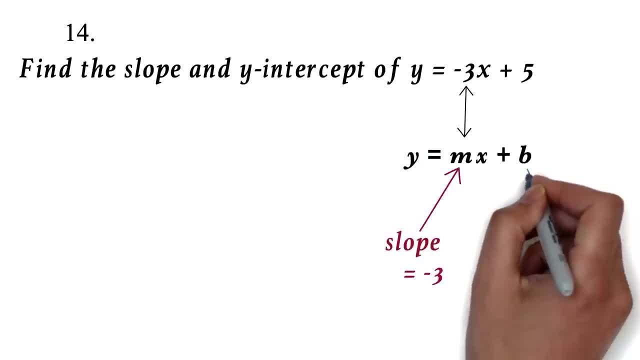 is our slope, The y-intercept is the b. This is the constant, or simply put, what is without the x. So here the 5 will be our y-intercept. Slope is negative 3, y-intercept is 5.. 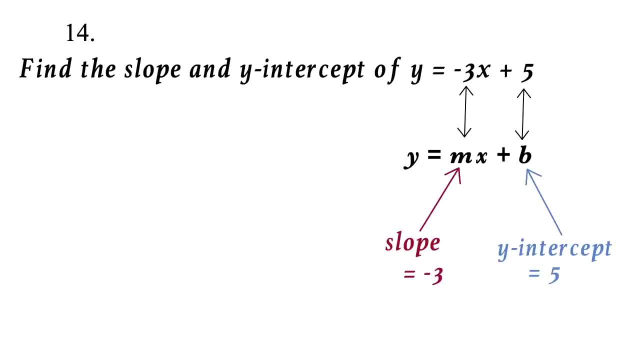 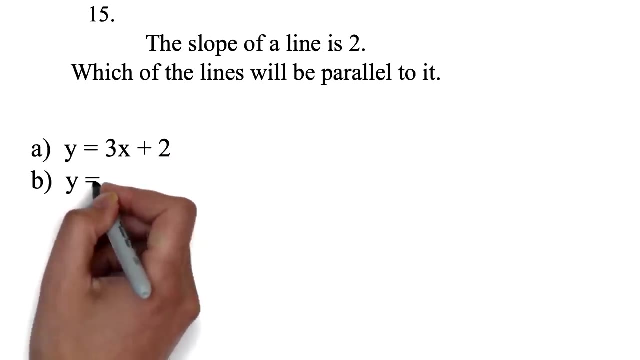 Pretty straightforward once you know the formula. Question 15.. The slope of a line is 2.. Which of the lines will be parallel to it? a? y equals 3x plus 2.. b? y equals 2x plus 3.. 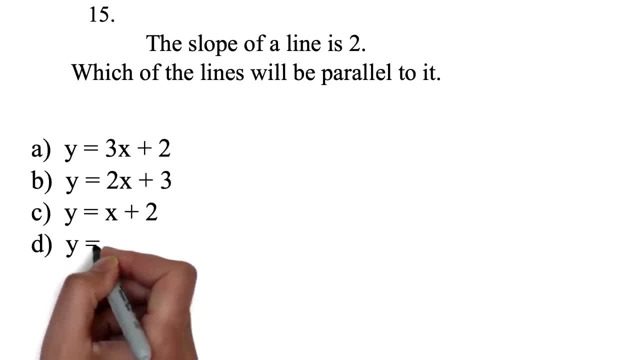 c? y equals x plus 2.. d? y equals negative 1 over 4x plus 3.. Lines with the same slope are parallel. Since the slope of the line is 2, we are basically looking for the answer which also has slope of 2.. 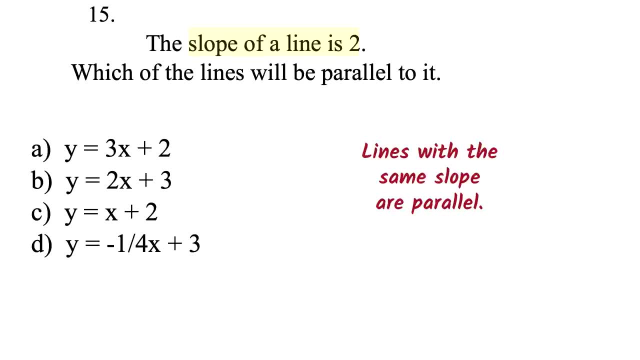 All the answers are in the slope-intercept form of the equation of a line That is: y equals mx plus b. We know that in this form, the coefficient of the x- or simply put what is with the x- is the slope Choice. b has the coefficient of the x to be 2.. 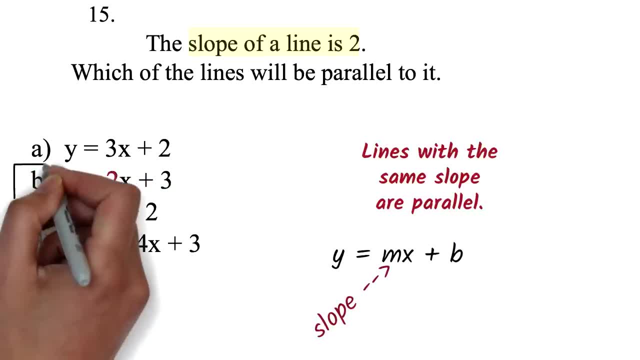 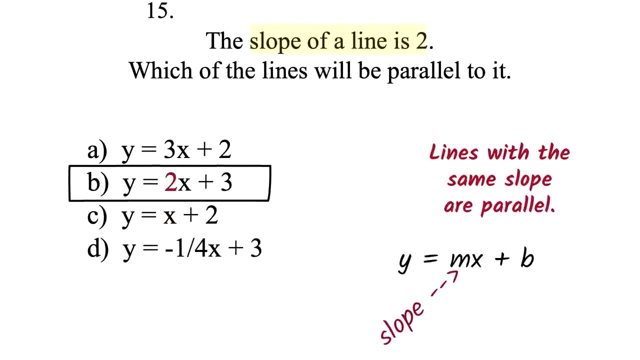 That means it has the same slope of 2 as the question. Therefore it's parallel Question 16.. The slope of the line is 2.. Let's take a look at the question again, Question 17.. The slope of the line is 3.. This is the constant, or simply put, what is without the x? 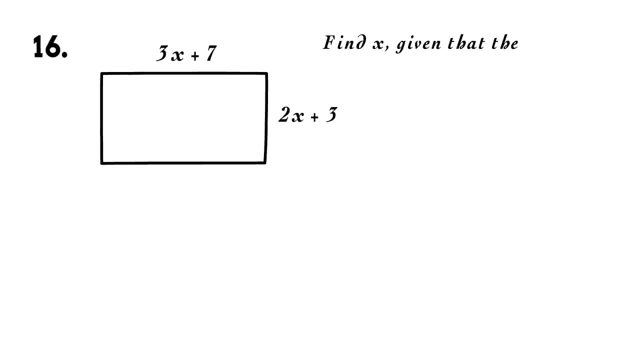 question 16.. Here we are supposed to solve for x, given this rectangle. We know that perimeter simply means adding all the sides. We know this is a rectangle, so opposite sides have the same size. This place will also be 2x plus 3. This will be 3x plus 7.. Now we can add all these parts. 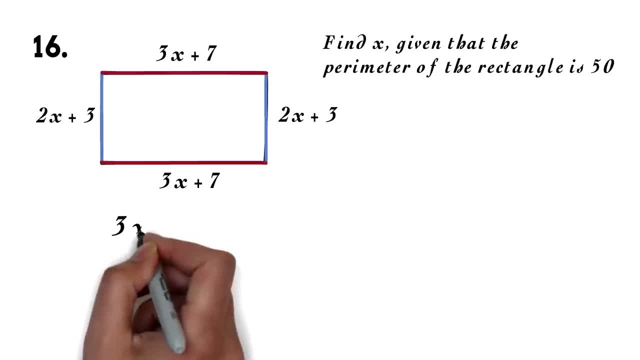 and it must be equal to the perimeter 50. We have 3x plus 7 plus 2x plus 3 plus 3x plus 7 plus 2x plus 3. This is equal to 50. We can add all the x terms: 3x plus 2x plus 3x plus 2x. 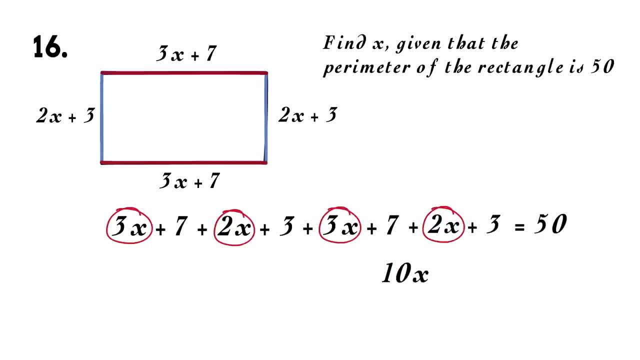 This will give us 10x. We can add the numbers 7 plus 3 plus 7 plus 3.. This will give us 20.. We have a two-step equation here which you should be very familiar with how to solve. 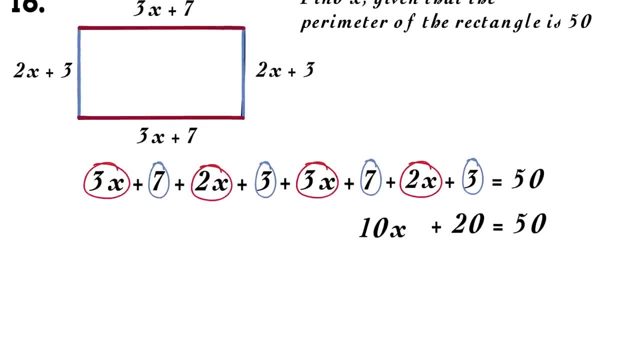 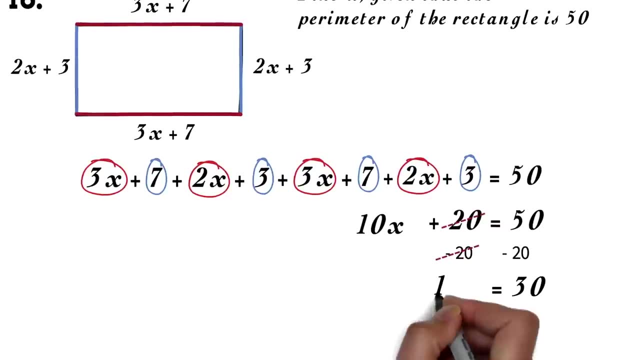 You can check out our video on equations if you need help. Subtract 20 from both sides. The 20 will cancel out. 50 minus 20 is 30. Now we have 10x equals 30. We can divide both sides by 10.. 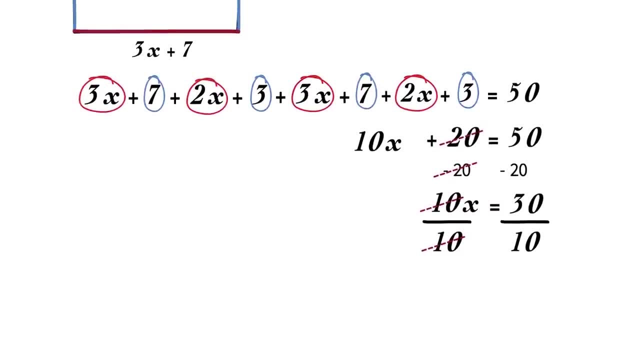 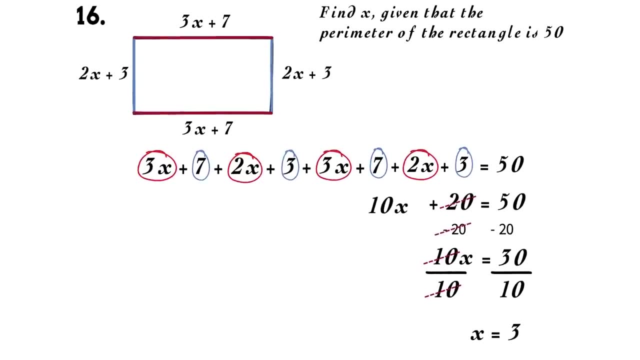 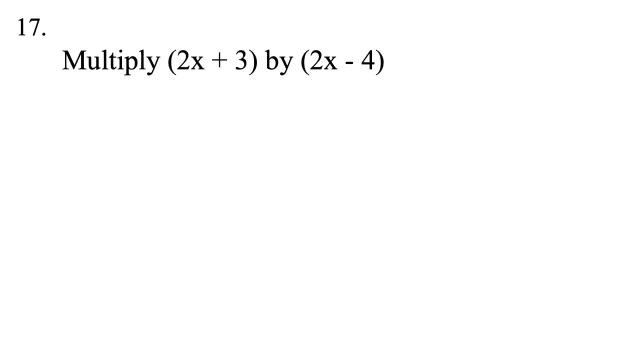 The 10 will cancel out. 30 divided by 10 is 3.. So we have x equals 3.. Question 17.. We want to multiply the polynomials 2x plus 3 and 2x minus 4.. We multiply each term in the second parenthesis by the terms in the first. 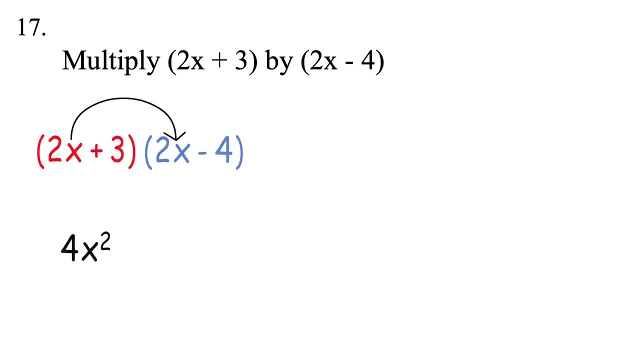 So 2x will multiply 2x to get 4x squared. Then 2x will multiply negative 4 to give us negative 8x. Next we will multiply by the 3. 3 times 2x is 6x. 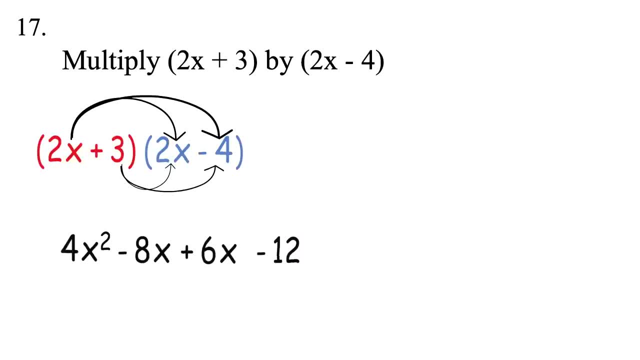 3 times negative. 4 is 6x 3 times negative. 4 is 6x 3 times 2x is 6x 3 times negative. 4 is 6x. 4 is negative 12.. 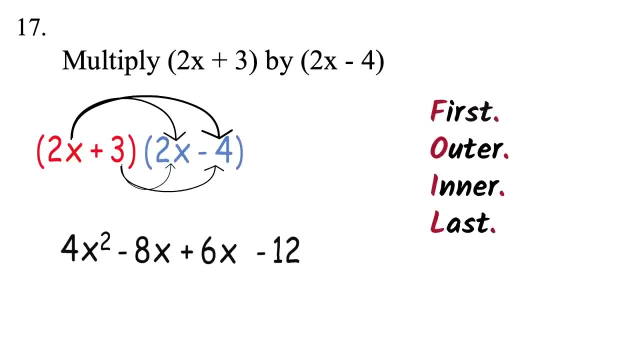 Please note that the method we used is what is commonly known as the FOIL method. I'm personally not a fan of most acronyms in math. They bring little benefits and can actually cause you to get questions wrong. Next we check if there are like terms we can add or subtract. 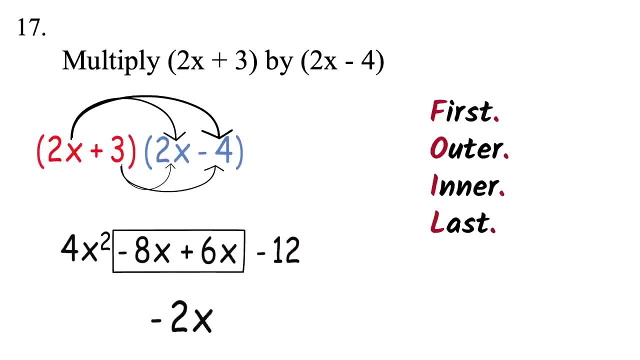 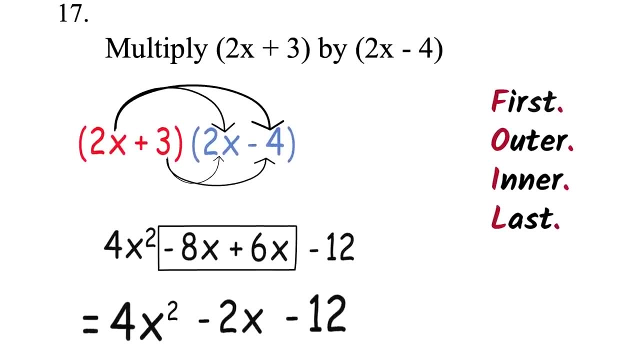 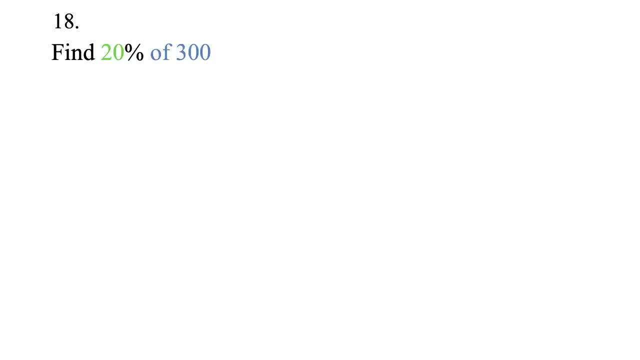 We can add negative 8x and 6x to get negative 2x. So our final answer is 4x squared minus 2x minus 12.. Question 18. Find 20% of 300.. There are three good methods for solving questions like this. 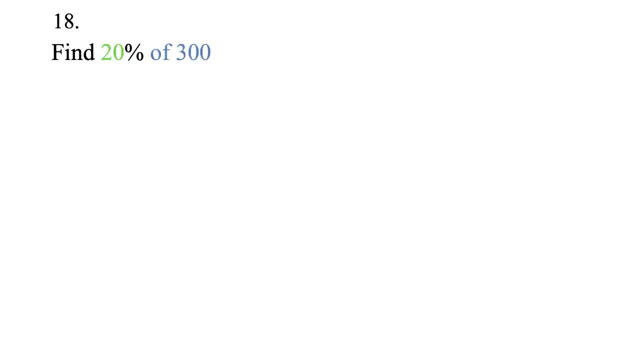 Please watch our other videos to see other ways of solving it and pick the one that's best for you. We will use the proportion method For this method. we will put our is value here. We will put our of value here. We will put our percent value here. 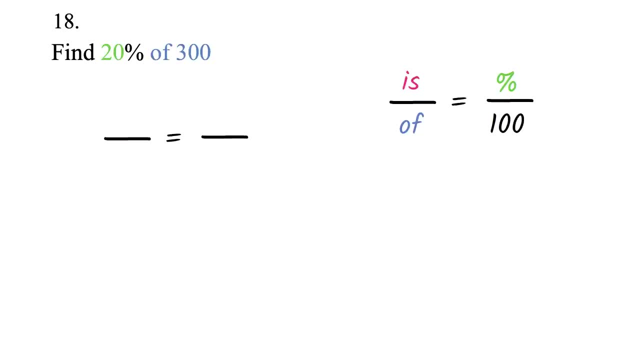 Then 100 here For this question. we have 20%, So we put 20 for our percent value. We have of 300.. So the 300 is our of value. We will put it here. We have 100 here, which is constant. 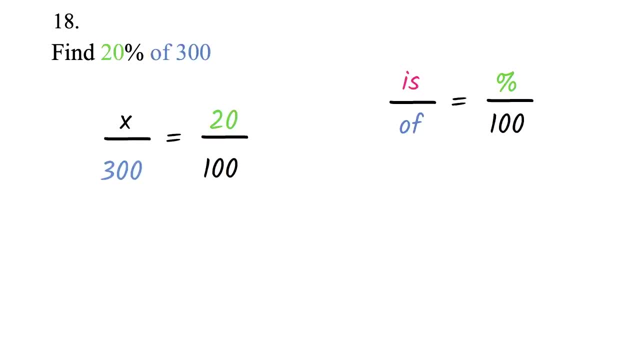 Now we have our, is value left, so we can represent by x and solve for x. This is a one-step equation. Since the 300 is dividing, we will perform the opposite operation on both sides of the equation: We will multiply both sides by 30.. 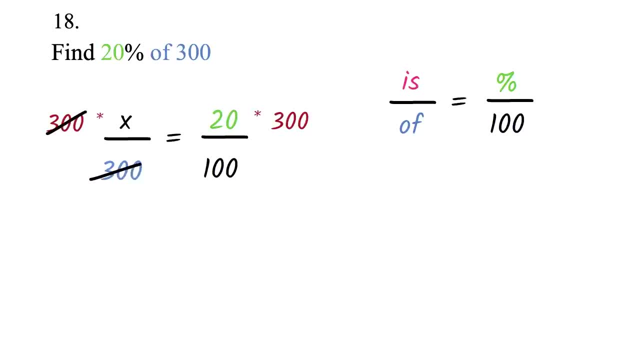 The 300 will cancel out. We simplify this part: 300 divided by 100 is 3.. We have 20 times 3,, which is 60.. Therefore, x equals 60.. So 60 is 20% of 300.. 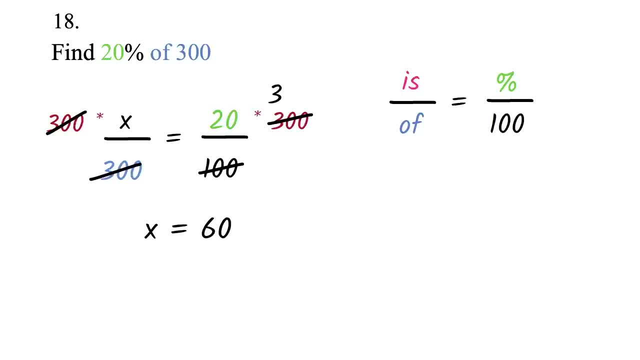 We can see that once you can set it up, it takes a little algebra and basic math to get the answer. The only problem I see is when the question is phrased like: what is 20% of 300?? We can see that once you can set it up, it takes a little algebra and basic math to get. 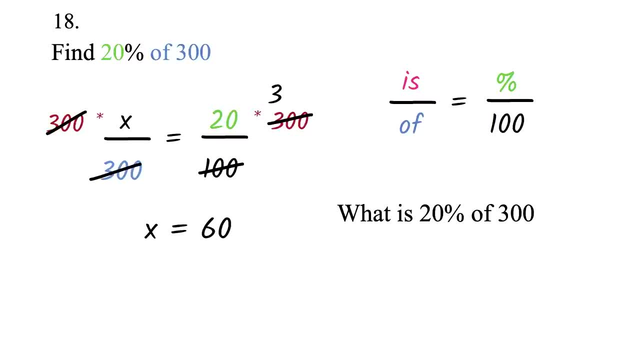 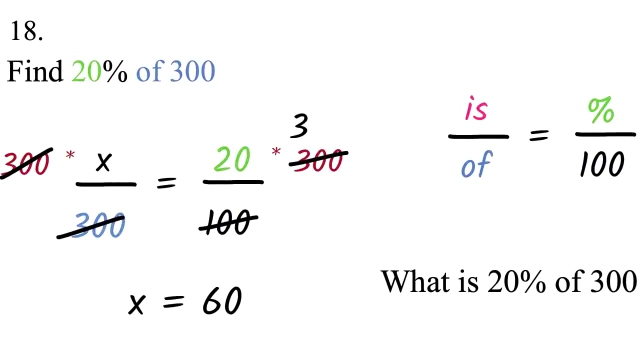 the answer. Students get confused if the 20 is an is value or a percent value. Numbers with percentage symbols are always the percent value, irrespective of where they are placed, So this question is exactly like what we just solved. Let's look at another example. 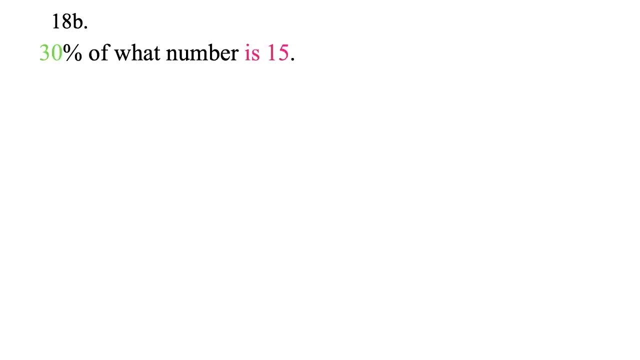 Question 18b: 30% of what number is 15?? The answer is 15.. The answer is 15.. We are using the same method as the question 18.. Please watch our other videos for other methods. For this method we have our is value here. 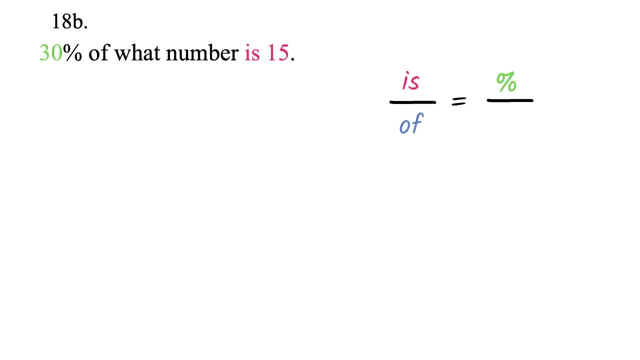 We have our off value here, We have our percent value here And then 100 here. Now let's look at our question. We just replaced the values. Let's write our 100 here first, We know it's constant. We can write the 30 here, because it's our percent value. 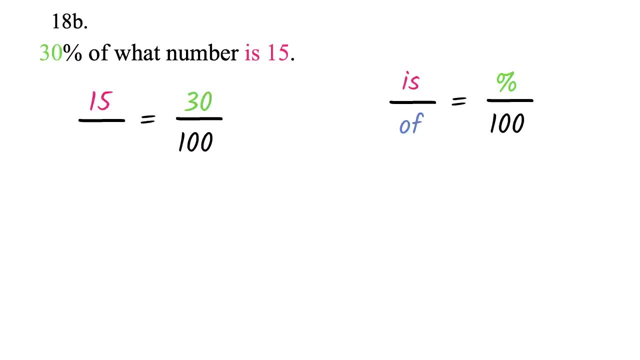 We have is 15.. So we write 15 as our is value. Finally, we have off, but there's no number with it. We represent it by x and solve for x. Since the x is in the denominator, your first step will be to cross multiply. 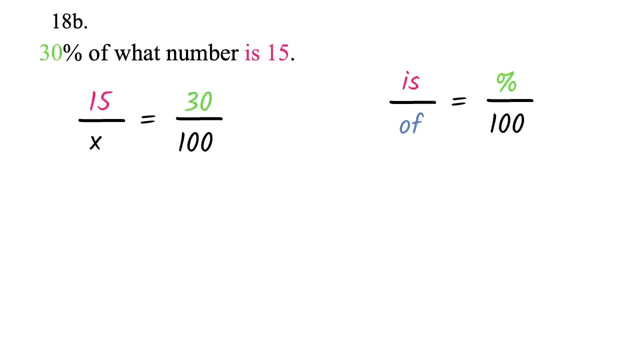 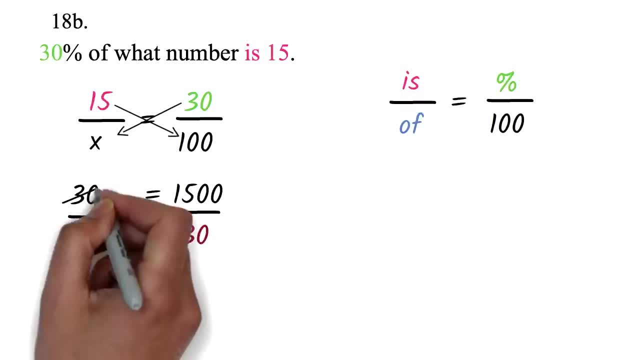 Then we have x and solve for x. so we will divide both sides by 30. The 30 will cancel out. 1,500 divided by 30 is 50. Therefore x equals 50, meaning 30% of 50 is 15.. 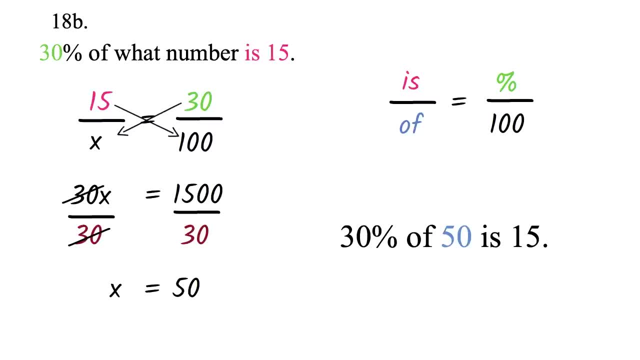 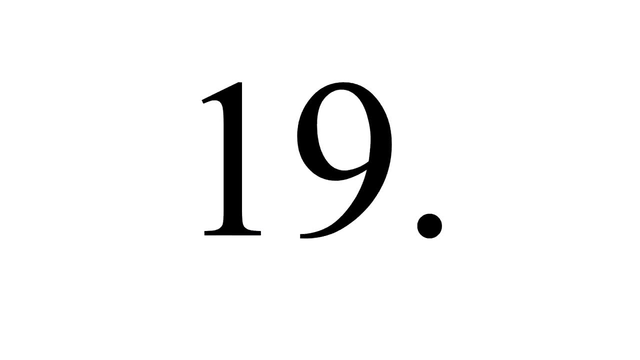 Please, I cannot overstress the importance of knowing how to solve these kind of percentage problems. You have to master it. Graph the inequality x greater than negative four. Let's bring our number line. When graphing inequalities, the first thing is to locate your point. 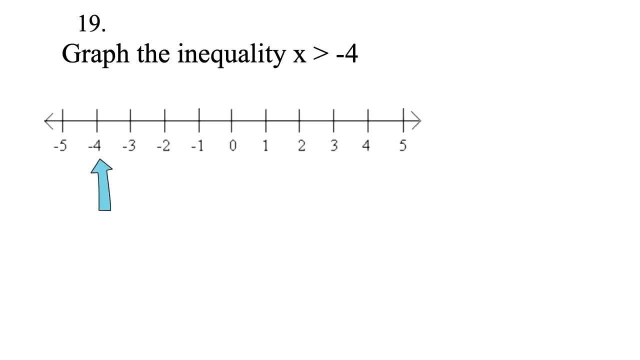 which will be the number Here? it is negative four. Then you'll draw a shaded or unshaded circle at the point. If you have less than or greater than, then the circle will not be shaded. If you have less than or equal to, 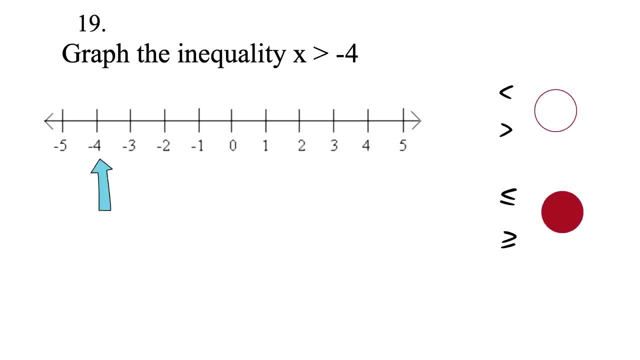 or greater than or equal to you will use the shaded circle. So, basically, if it has an equal to you will shade. In this case, since it's just greater than we will not shade the circle. Then, finally, we draw an arrow. 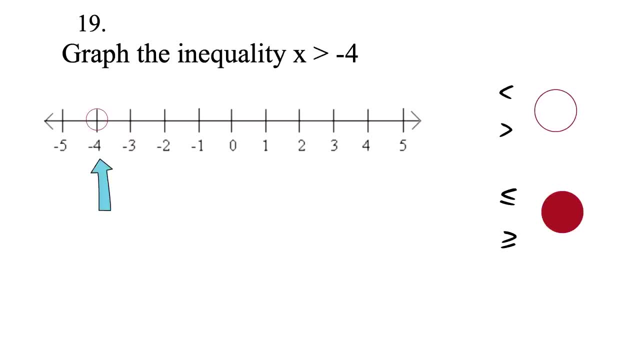 The easiest way to get this always right without thinking is to make sure your inequality is in the form variable inequality sign and then the number. In that form, the direction of your arrow will be the same as the direction of the inequality sign. 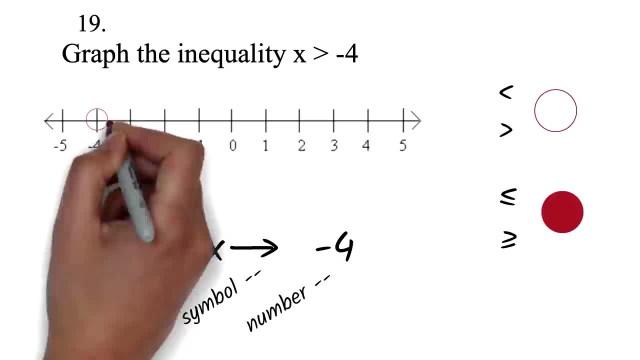 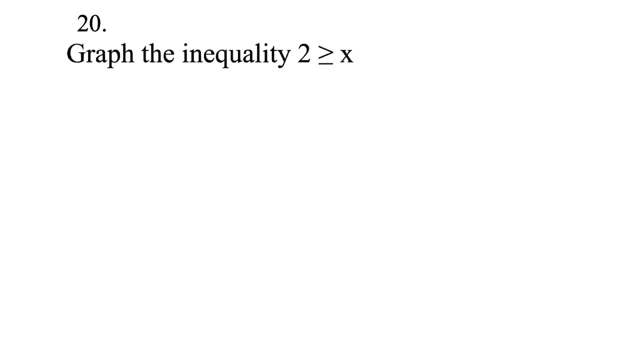 Here, since this is in that form we will draw our arrow facing here, and we are done. Graph the inequality: two greater or equal to x. Let's bring our number line. We follow our steps. We first locate our point, in this case two. 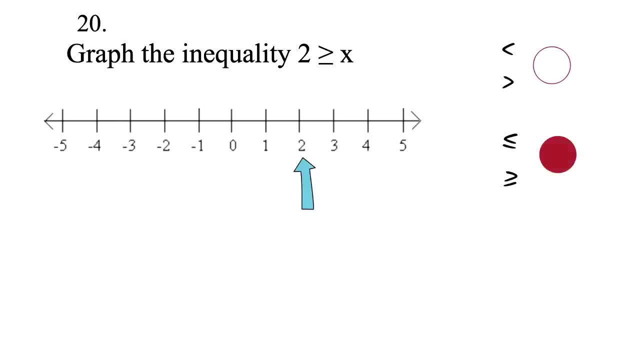 We decide if it should be shaded circle or not. In this case it will be shaded because it's greater than or equal to. We set it shaded if there is equal to. Then, finally, we find out the direction of our arrow. We set if the inequality is in the form. 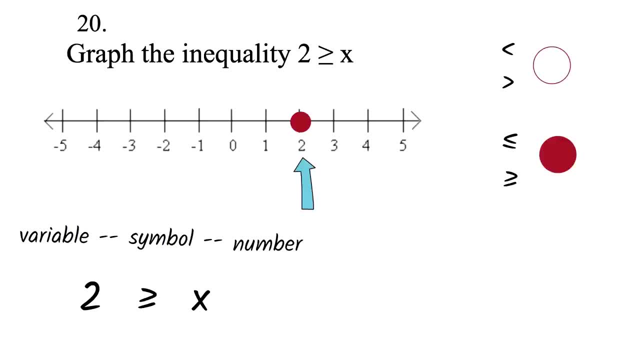 variable inequality sign and the number. the direction of your arrow will be the same as the direction of the inequality sign. This is not in the form, so your arrow will face the opposite direction as the inequality Here. normally your arrow will face this way. 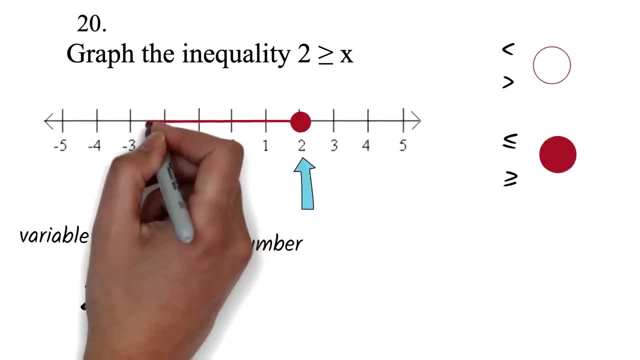 but now it will rather face this way, So we will draw our arrow here. Another way to look at inequalities in this form is to always convert it to the form variable inequality sign and the number If your brother is older than you. 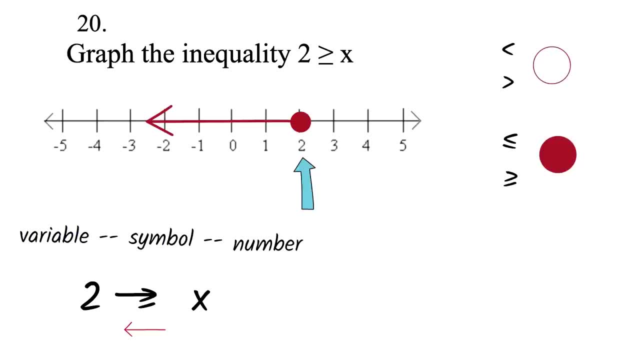 it means that you are younger than your brother. So if two is greater or equal to x, then we can say that x is less or equal to two. You can look at it as just a mirror image. In this form we can easily notice. 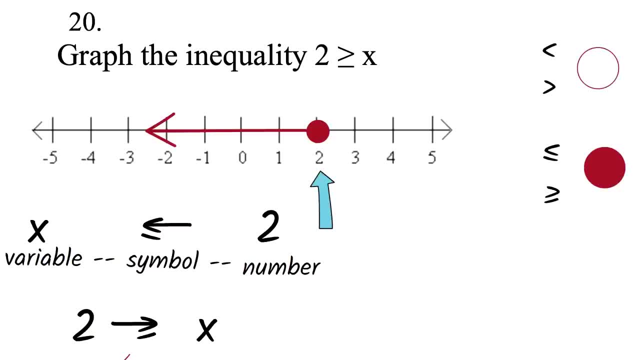 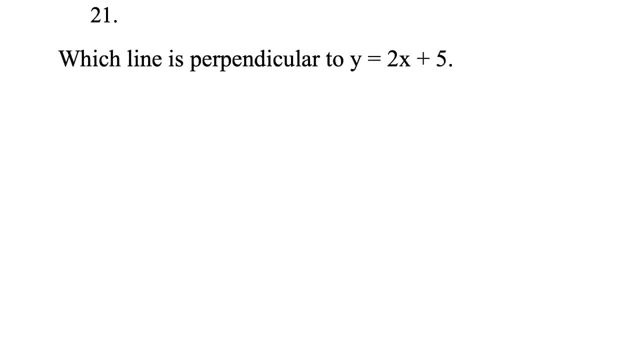 the direction of the arrow, We get exactly the same answer. Question 21.. Which line is perpendicular to? y equals two x plus five. A? y equals two x minus one. B? y equals negative two x plus five. C y equals three over four x plus five. 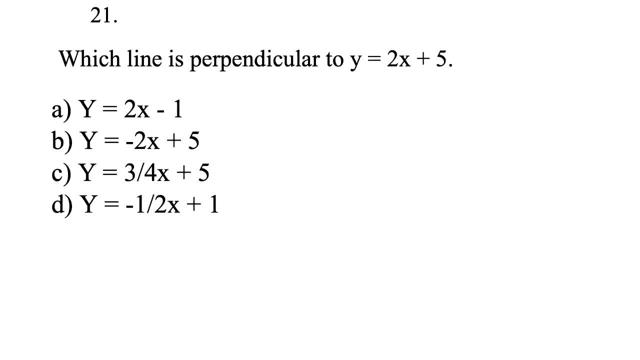 D, y equals negative one over two, x plus one. The slope of a perpendicular line is the negative reciprocal of the slope of the original line. The reciprocal of a number is basically flipping the numerator and denominator. So three over four will be four over three. 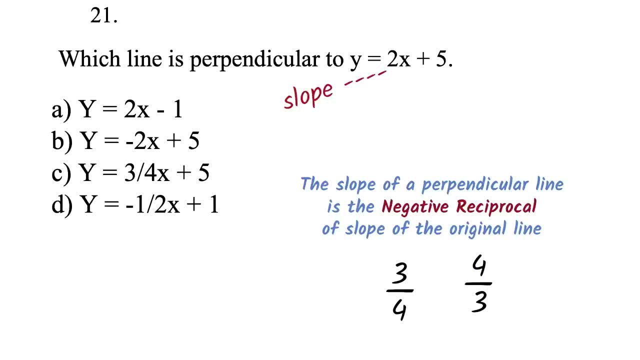 Here we know the slope of the question is two. Since this is in the slope intercept form of the equation of a line, Please revise question 14 and 15 if you have forgotten. the slope intercept form. Two is the same as two over one. 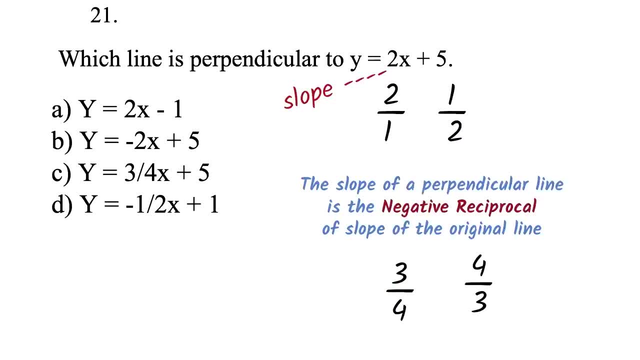 The reciprocal is one over two. The negative reciprocal of two is therefore negative one over two. We are looking for the answer which has a slope of negative one over two, 2. Choice D has the coefficient of the x to be negative 1 over 2. That means choice D has a. 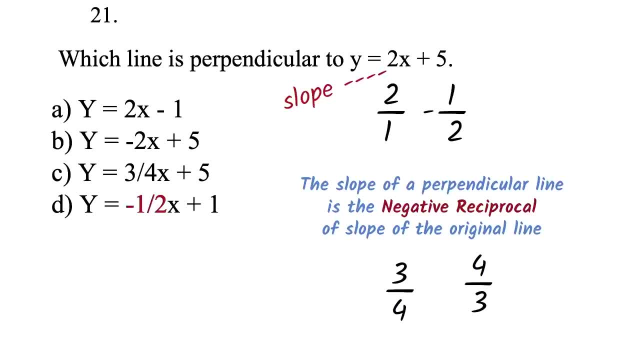 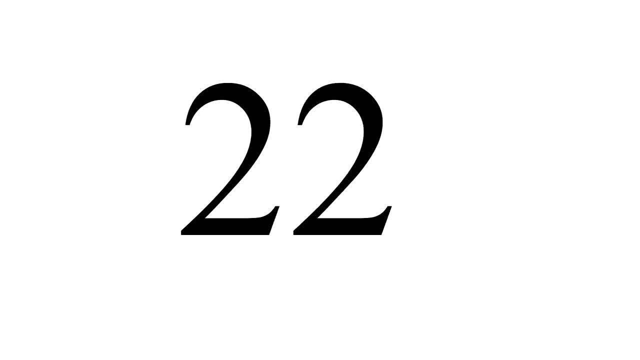 slope of negative 1 over 2.. This is the negative reciprocal of the slope 2 in the question. Therefore it's perpendicular. The product of two consecutive integers is 30.. Find the two numbers. This is a question that you can easily solve without using any mathematical methods. 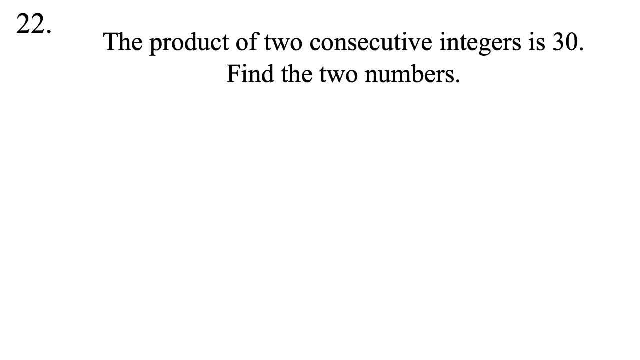 Consecutive integers are simply numbers that follow each other. So 3,, 4,, 5, 6 are consecutive integers. 25 and 26 are also consecutive integers. I'm sure you get the point. So we are looking for two numbers that multiply to get 30. The two numbers must also follow each other. The two 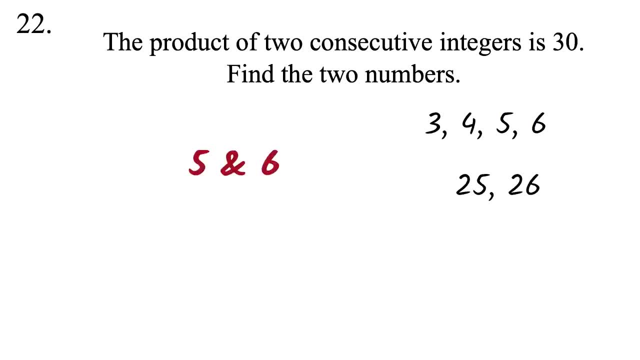 numbers are 5 and 6.. 5 times 6 is 30. Pretty straightforward if you know your multiplication table. Question 23.. The product of two consecutive integers is 30. If the smaller number is x, write an equation to find the value. This is the same as question 22,. just harder: The GED. 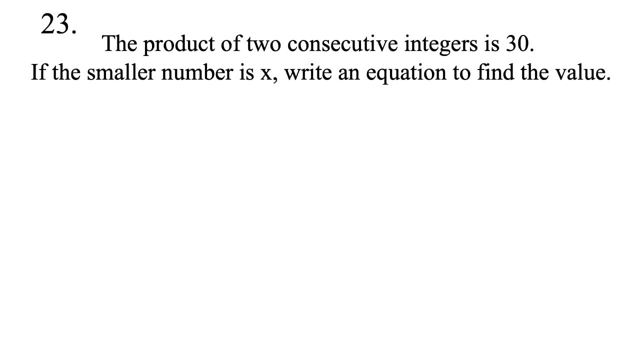 is now having more questions in which the answers are not actual values, but an expression, a function or an equation. This is a typical example. We know that consecutive integers are numbers that follow each other For consecutive integers. we know that consecutive integers are: 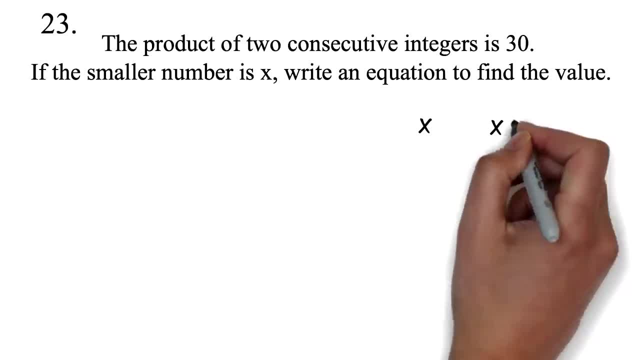 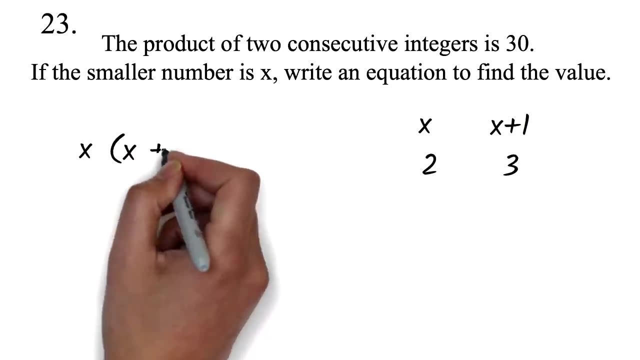 integers. If the smaller number is x, then the next number will be x plus 1.. So if x is 2, then the next number will be 2 plus 1, which is equal to 3.. Product means multiplication. So we have the smaller number x times the next number, x plus 1, to be equal to 30. We can expand. 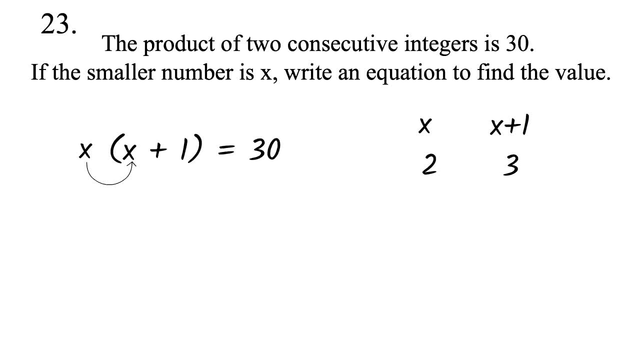 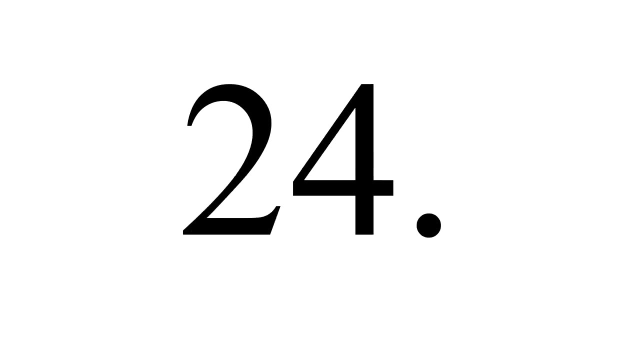 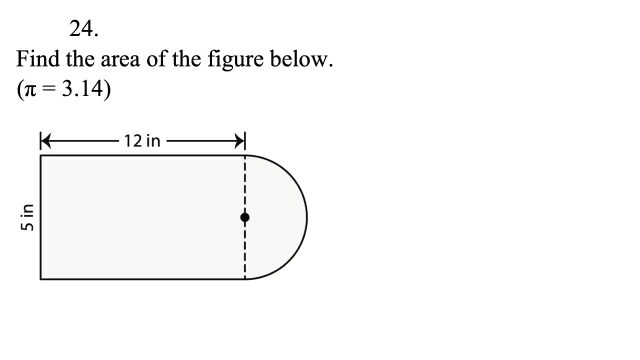 this. We have x times x. This will give x squared. Then we have x times 1, which is 1x or simply x. So the equation is: x squared plus x equals 30.. Find the area of the figure below. Use pi equals 3.14.. The work here is to be able to identify that. 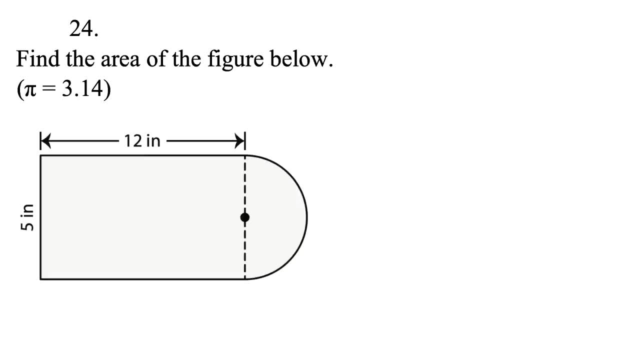 you can break this into multiple shapes. Find the area of each shape and add the areas For this figure. we can draw a line here so that we have a rectangle A and a semicircle B. Area of a rectangle is length times width. This formula is given on the GED formula sheet. 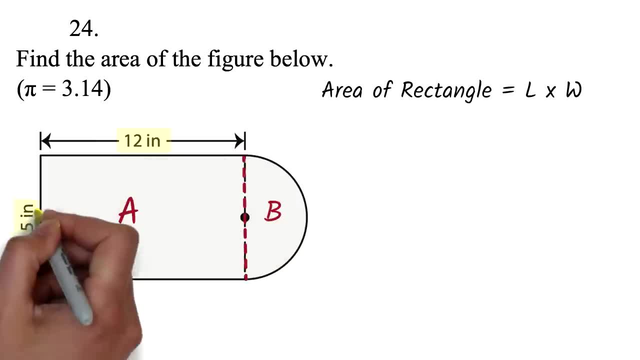 We know the length as 12 inches and the width as 5 inches. We multiply it to get 60 inches squared. Next we have to find the area of the semicircle. The area of a circle is pi r squared. This formula is also provided on the GED. So the area of a semicircle or half a circle. 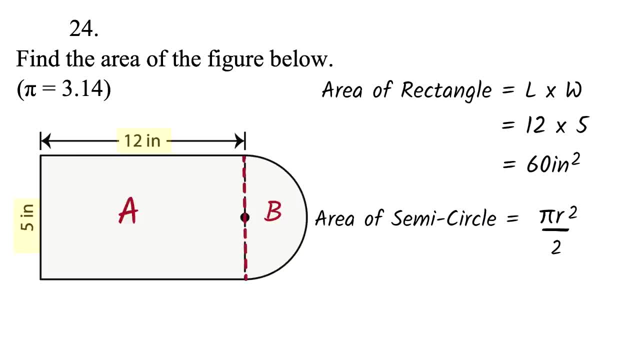 will be pi? r squared over 2.. We don't know r. We know that, since this is a rectangle, if this side is 5 inches, it means this side will also be 5 inches. This means the diameter of the circle is 5.. 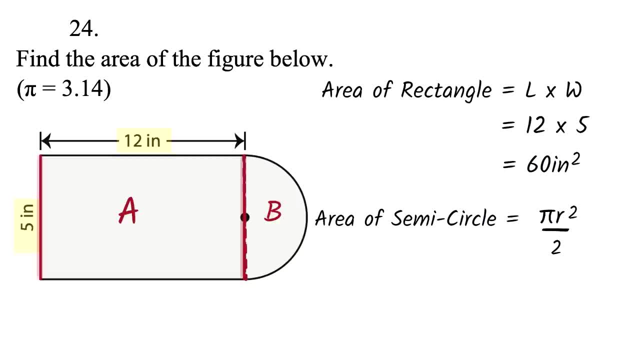 The radius of a circle is half the diameter, so we divide the 5 by 2 to get 2.5 as the radius. Now we find the area of the semicircle, pi, which has been given as 3.14 times 2.5, squared over 2.. 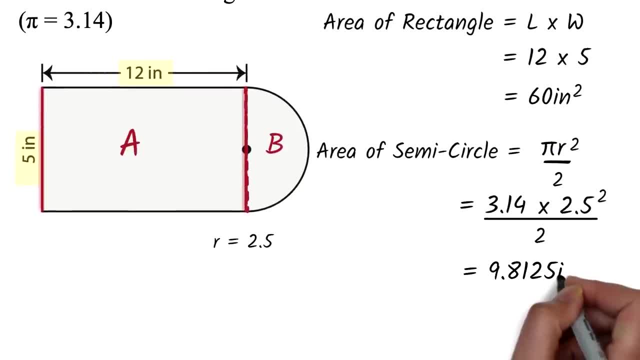 We compute it on the calculator to get 9.8125 inches squared. Finally, we add the area of the two shapes. We have 60 plus 9, .8125.. This will give us 69.8125 inches squared as the area. 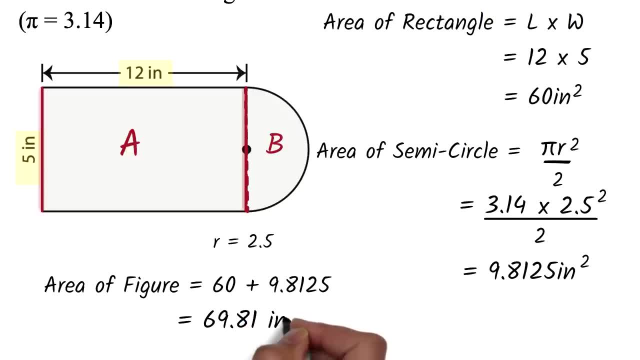 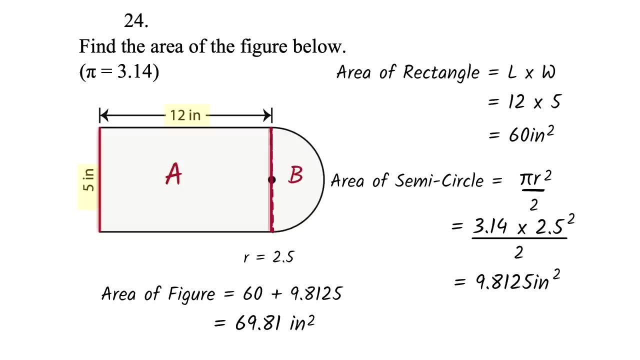 To two decimal places will be 69.81 inches squared. Please? questions here can be in any form. Break them into multiple shapes. Find the measurements you need to find the area of each shape. Then combine the shapes. What function represents the information in the table? 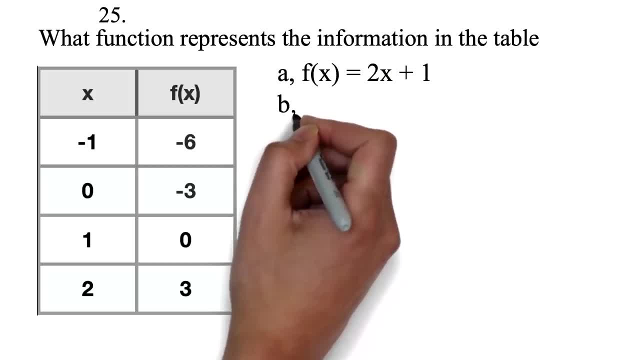 a- f of x equals 2x plus 1.. b- f of x equals x minus 3.. c- f of x equals x plus 3.. d- f of x equals 3x minus 3.. Here the best way is to solve. 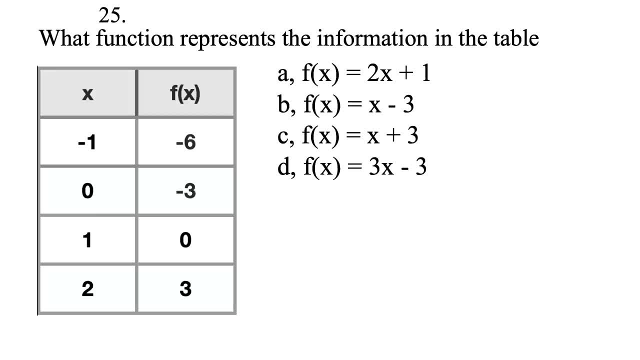 the equation. by using the equation We input the x values into the various functions and see if we will get our f of x values For teaching purpose. we are going through everything You don't have to. on the test You can accurately eyeball and eliminate obvious wrong choices. 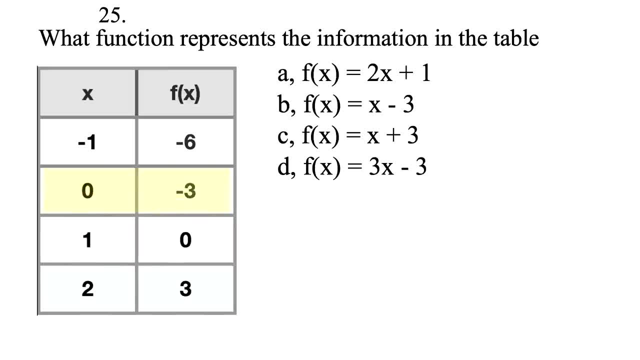 Since it's easy to work with 0, I'll try that first so I can narrow the possible answers. Replace x with 0 for choice A. 2 times 0 plus 1 equals 1.. It was correct. It was supposed to be negative 3.. 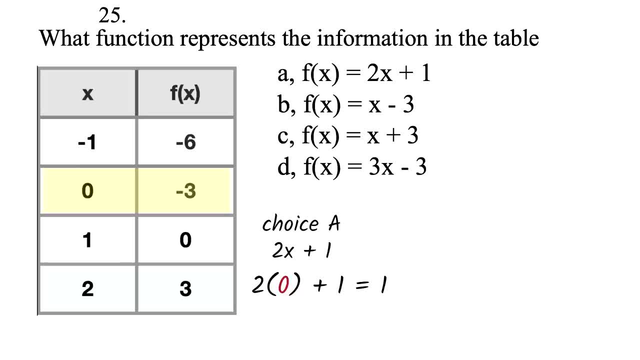 So choice A is definitely wrong. Replace x in choice B with 0.. 0 minus 3 equals negative 3.. So choice B is a possible answer. Now replace x with 1 in choice B to confirm: 1 minus 3 equals negative 2.. 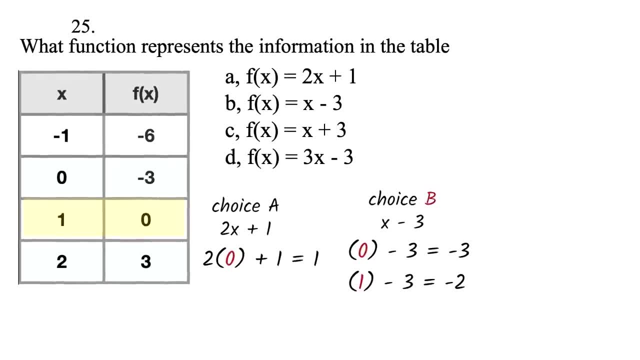 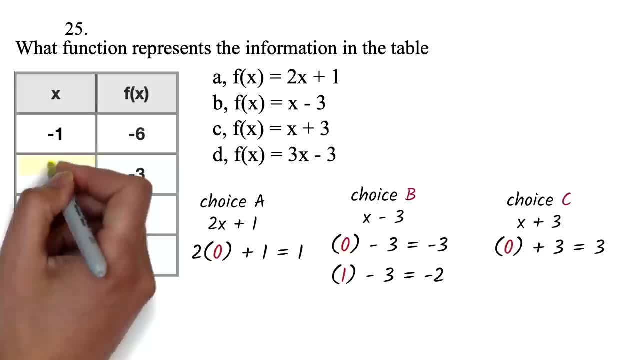 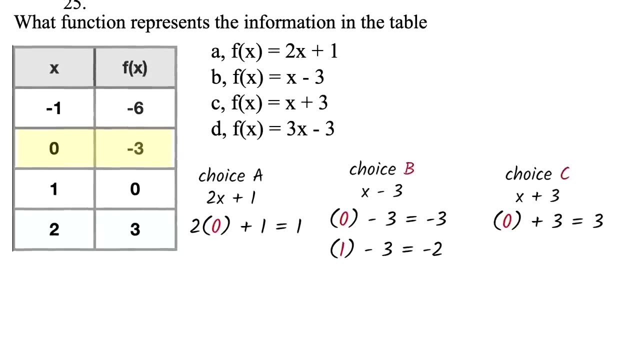 It was supposed to be 0. So choice B is wrong. Replace x in choice C with 0.. 0 plus 3 equals 3.. It was supposed to be negative 3.. So choice C is wrong. So since choice A to C are wrong, it means choice D will be the answer. 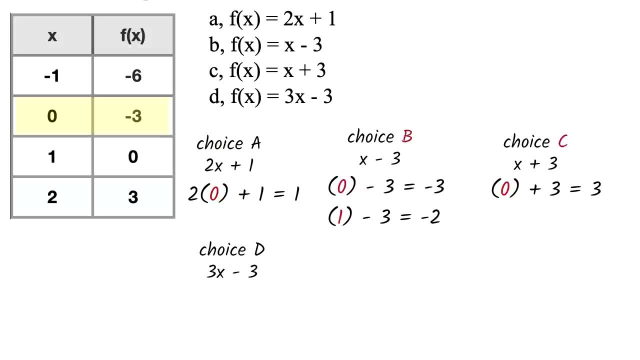 Let's confirm. Let's replace x with 0.. We have 3 times 0 minus 3 equals negative 3, as expected. We try 1.. We have 3 times 1 minus 3 equals 0, as expected. Then we try 2.. 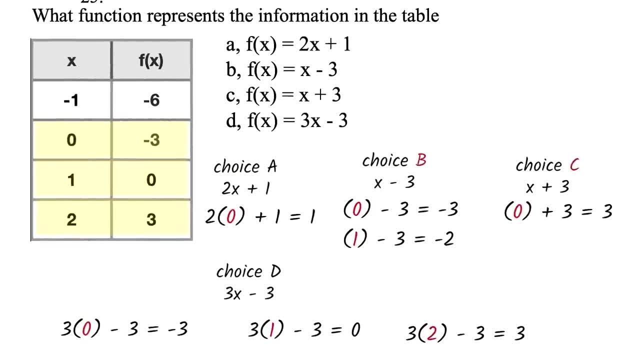 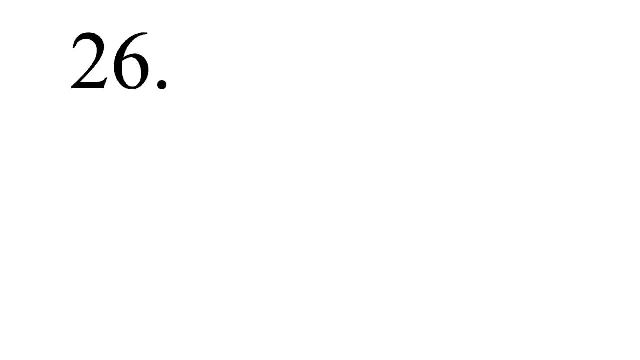 We have 3 times 2 minus 3 equals 3, as expected, So D is definitely the answer. A bus can take 12 students for a trip. How many such buses are needed to take 235 students for a school field trip? 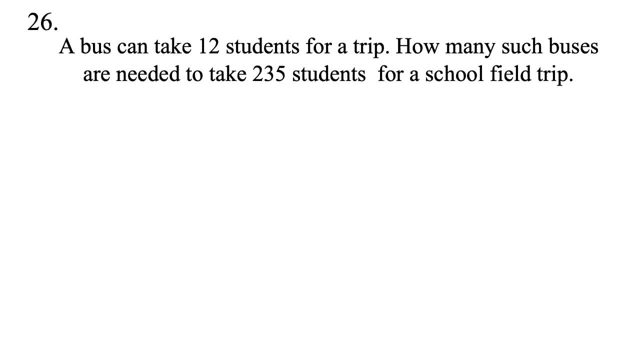 This is a straightforward division question. All you have to do to find the number of buses needed is to divide 235 by 12.. You compute this on the calculator to get 19.583.. For questions like this, when you get a decimal, you'll always round it up. 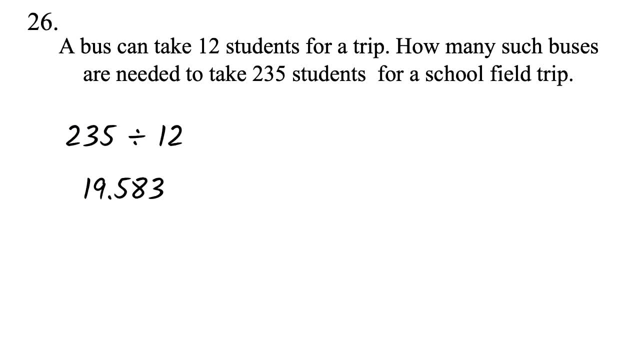 Because even if you have one student left, you have to use a full bus to take them. So we'll round the 19.583 up to get 20 buses as our answer. This question was pretty straightforward. That's why we simply used division. 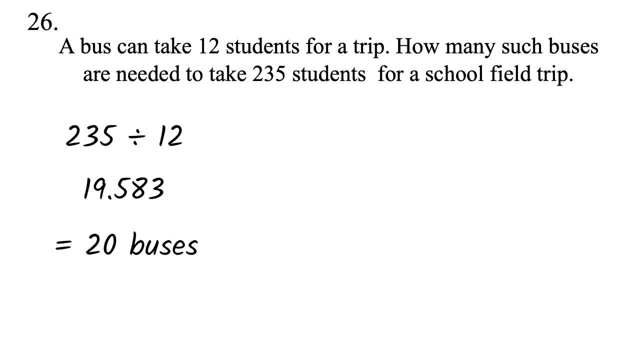 But the right way to solve questions like this, especially if complexities are introduced, is to use proportion. Setting up proportions is one of the most important word problem skills on the GED For this we will have. buses is to student. One bus took 12 students. 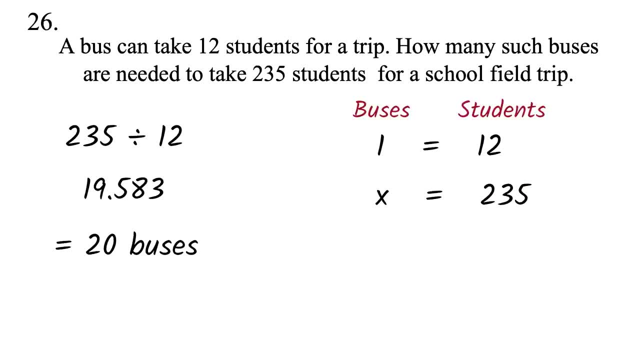 X buses will take 235 students. We solve for X. We first cross: multiply 12 times X is 12X. 1 times 235 is 235.. Next we can find the X by dividing both sides by 12.. The 12 will cancel out. 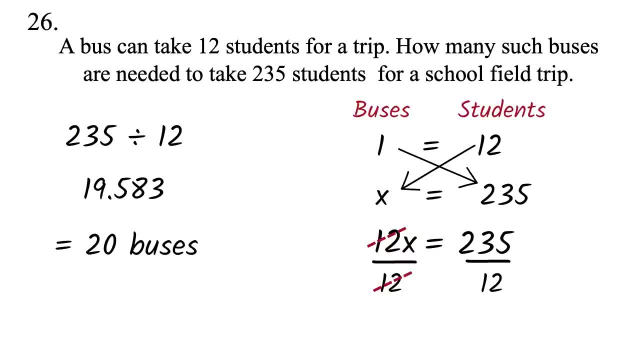 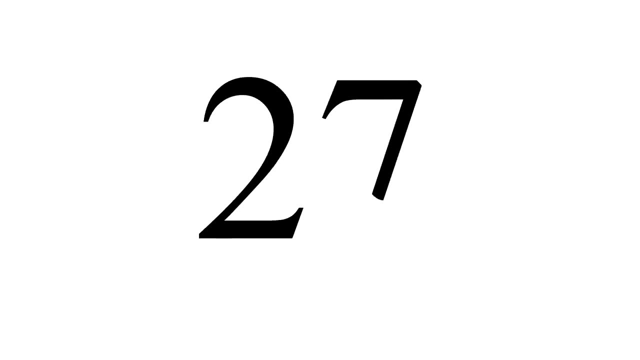 235 divided by 12 is 19.583.. You'll notice we got the same thing. The rest of the process is exactly the same. We round it up to get 20 buses as our answer. Faith spends 3 hours hiking 6 miles. 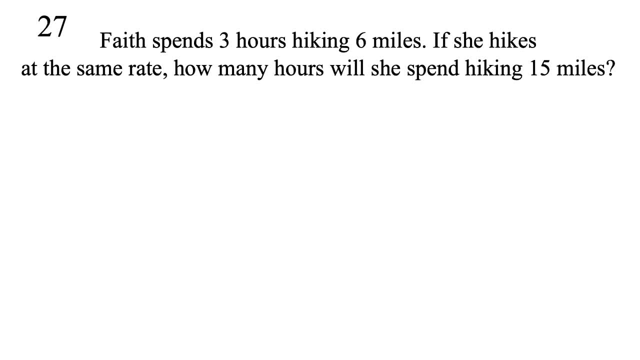 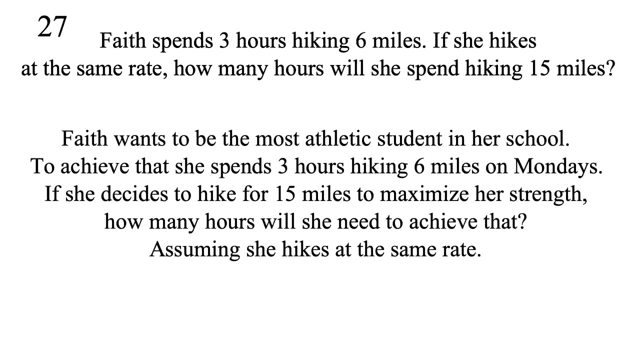 If she hikes at the same rate, how many hours will she spend hiking 15 miles? This is a typical proportion question. Please note that on the GED you can have questions with lots of unnecessary reading. This same question could have been: Faith wants to be the most athletic student in her school. 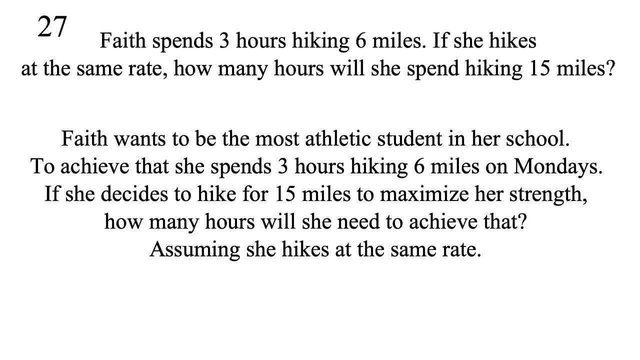 To achieve that. she spends 3 hours hiking 6 miles on Mondays. If she decides to hike for 15 miles to maximize her strength, how many hours will she need to achieve that, Assuming she hikes at the same rate? Okay, let's solve it. 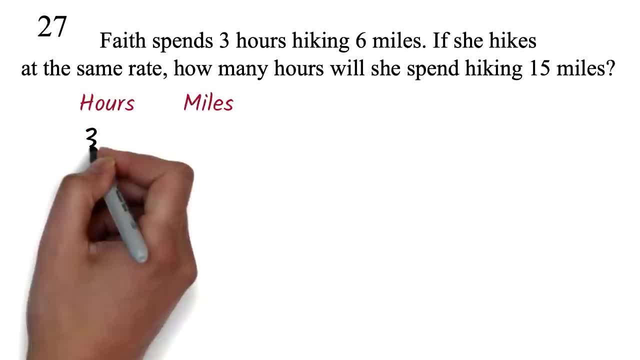 We have our hours here and miles here 3 is to 6.. Since we know the miles, 15, we'll put it here. Since we don't know the hours, or the hours is what the question is asking for- we will represent with X and solve for X. 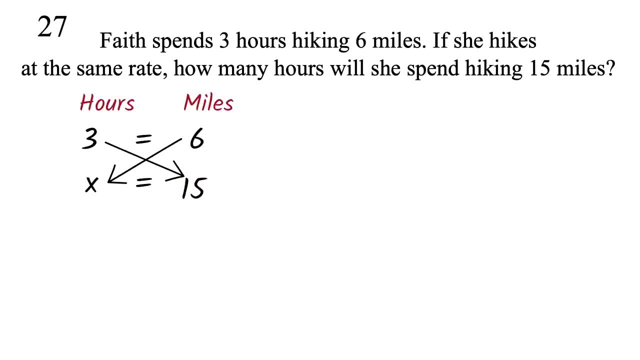 We cross. multiply 6 times X is 6X. 3 times 15 is 45.. We will now divide both sides by 6.. The 6 will cancel out. 45 divided by 6 is 7.5.. 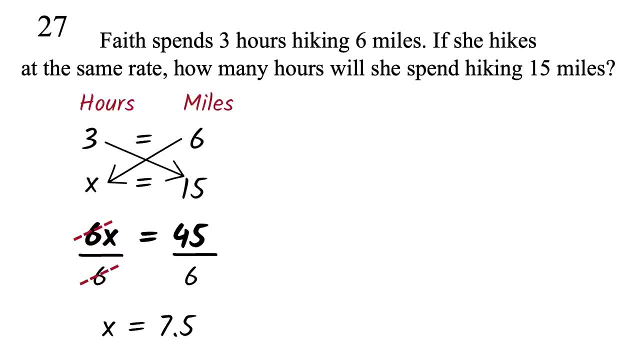 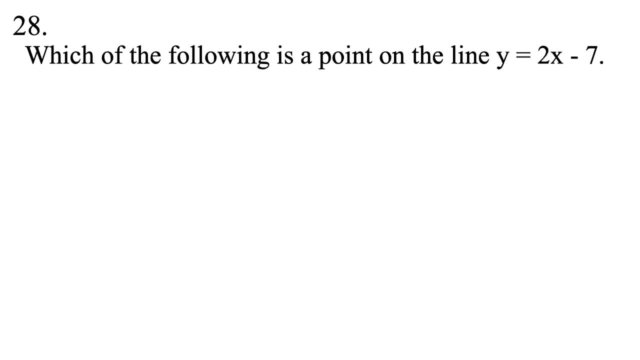 This is 7.5 hours, which is the same as 7 hours 30 minutes. Which of the following is a point on the line? Y equals 2X minus 7?. A 2, 5.. B 3, negative 1.. 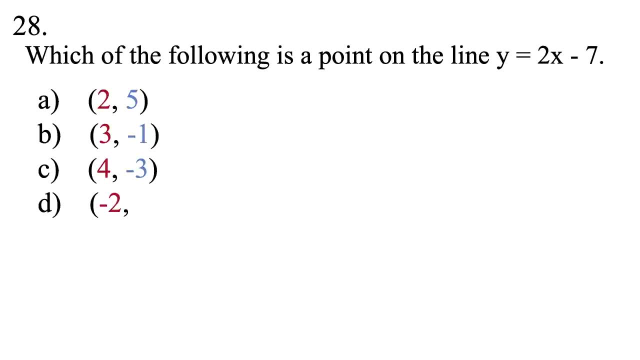 C- 4, negative 3.. D- negative- 2, 2.. We know that for a point, the first value is your X value and the second value is your Y value. If a point lies on this line, then when you input the X value into the equation of the line, 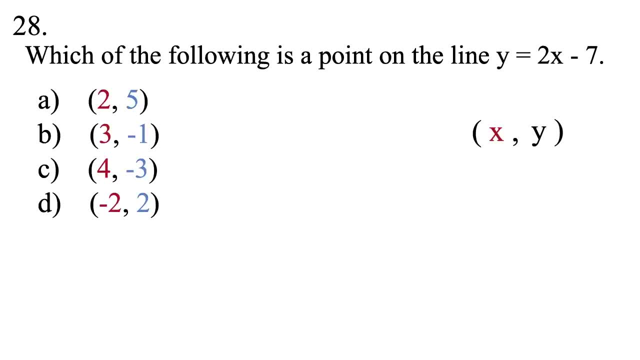 you should get the corresponding Y value. So we start with option A. We replace the X with 2. We have 2 times 2 minus 7. This is negative. 3. It was supposed to be 5. So choice A is wrong. 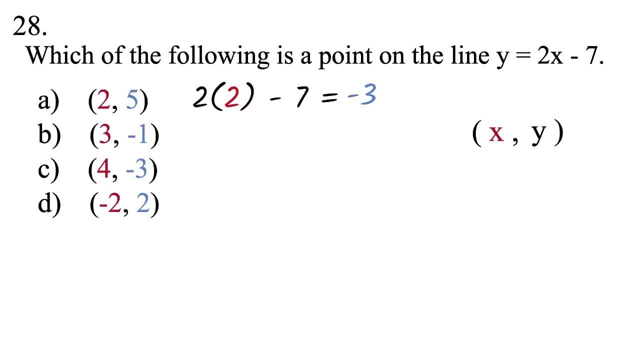 Let's try choice B. We replace the X with 3.. We have 2 times 3 minus 7. This will give us negative 1, which is what we expected. So choice B is the answer. The following graph represents the score range of students in a math class. 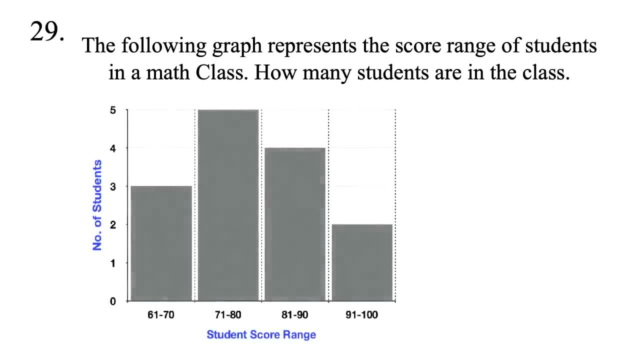 How many students are in the class. Being able to read and interpret graphs is a must on the GED. Here the X axis represents the score range and the Y axis represents the number of students whose score are within that range From the graph. 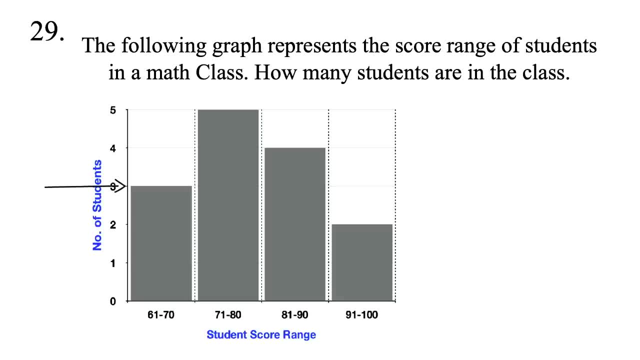 you'll notice that there are 3 students whose score ranged from 61 to 70.. From the graph, there are 5 students whose score ranged from 71 to 80.. From the graph, there are 4 students whose score ranged from 81 to 90.. 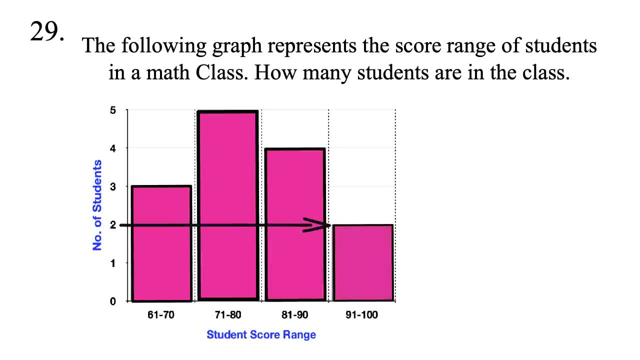 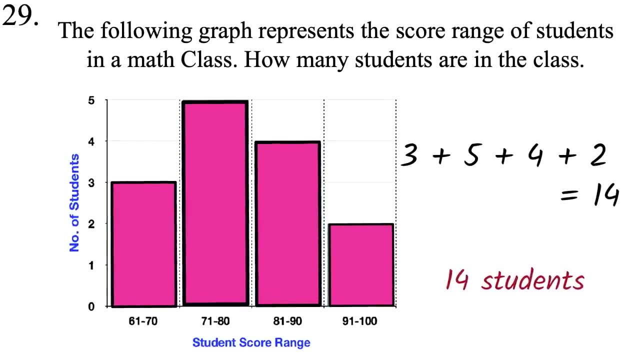 From the graph, there are 2 students whose score ranged from 90 to 100.. ranged from 91 to 100.. We add these to get the number of students. 3 plus 5 plus 4 plus 2 equals 14.. Therefore, there are 14 students in the class, Question 30.. The following graph represents the 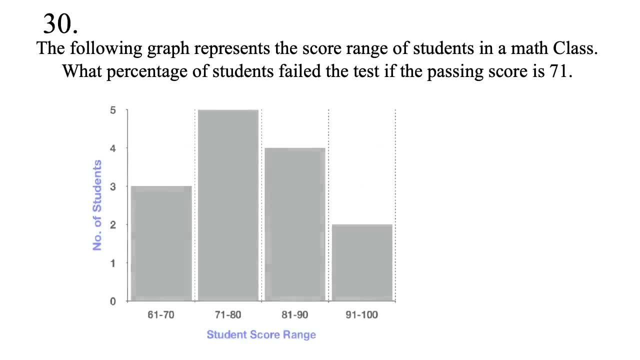 score range of students in a math class. What percentage of students failed the test if the passing score is 71?? Please, it's very important you master how to find percentages, especially from graphs. From the graph we can see that three students scored 61 to 70.. All the other students? 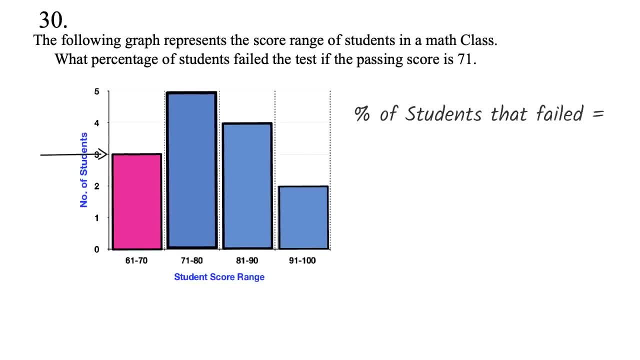 scored 71 or above. Percentage of students that failed will be the number of students that failed, which is 3,, over the total number of students, which is 14,, like we saw in question 29.. This will be multiplied by 100 to get the percentage. Compute this on the calculator to get 21.43%. 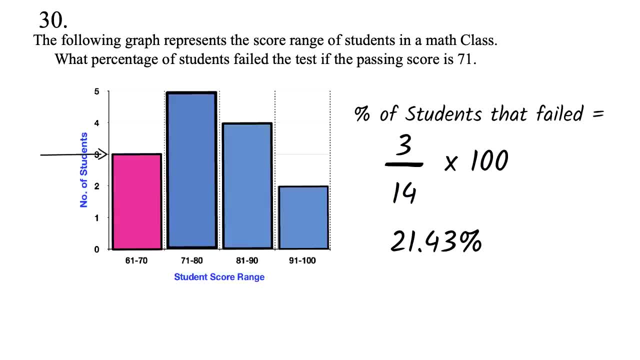 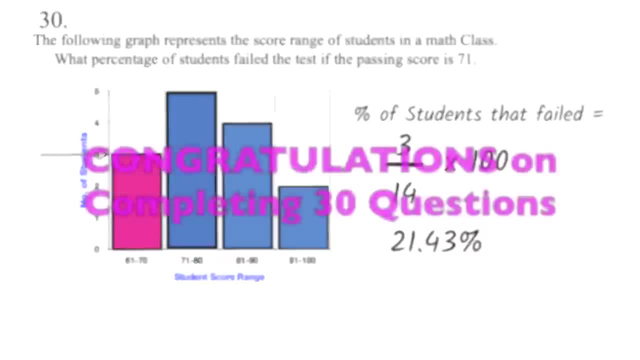 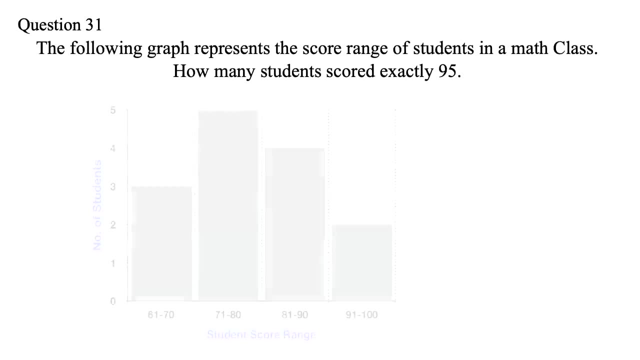 failed. With what you just learned, you should be able to answer questions like what percentage of students passed and what percentage of students scored 71 to 80.. Question 31.. The following graph represents the score range of students in a math class. How many students scored exactly 95? This? 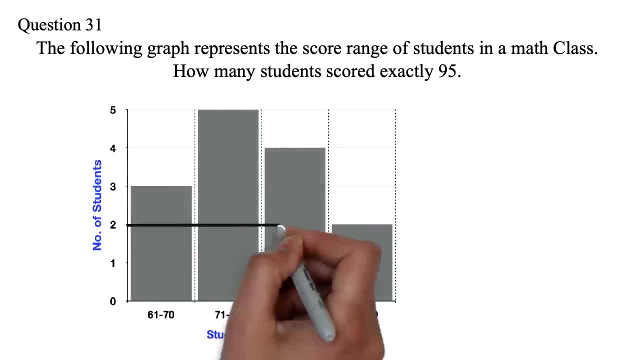 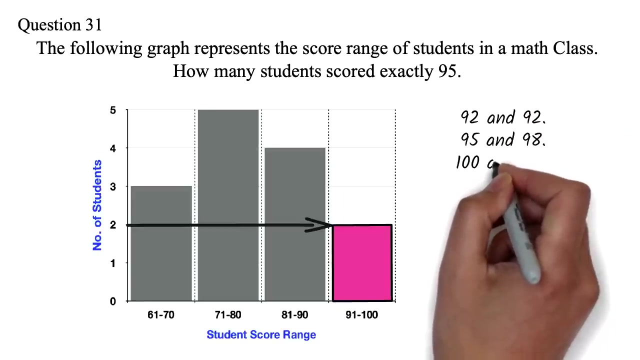 is a trick question. Most students assume that the answer is two students. Since the 95 is within 100,. this is wrong. A range doesn't tell you the exact values within the range. So the two students who scored between 91 and 100 could have scored 92 and 92,, or 95 and 98,, or 100 and 100. So the answer is: there's not enough data or information to answer the question. Please watch out for a little trick question like this. Pay extra attention to your graphs. 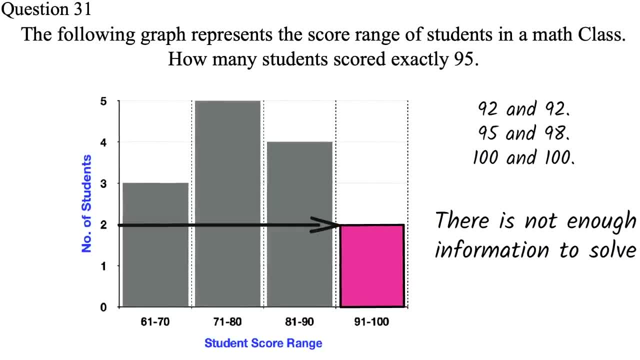 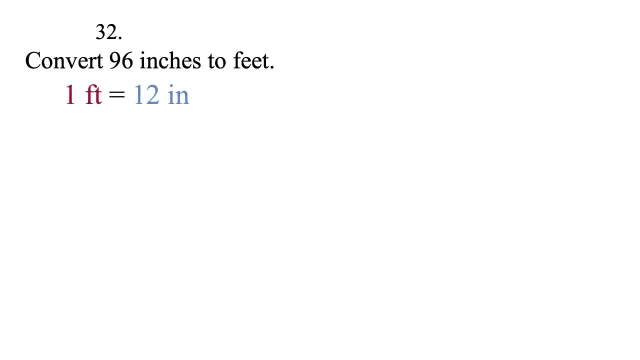 Question 32.. Conversely, do you know the answer for the first and last step? Convert 96 inches to feet. We are given our conversion factor. as one foot equals 12 inches, We can use proportions to solve it, like what we did in question 26 and 27.. Check. 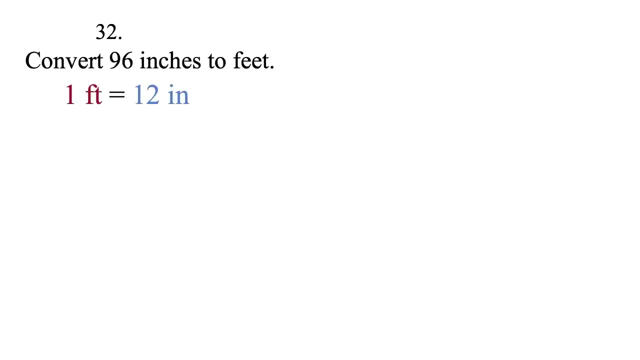 out ultimategedcom if you're interested in that method Here we'll solve it in another way. The best set-up looks like this: You'll first write down what you are converting When you hit No 1, you'll see the answer and enter it. 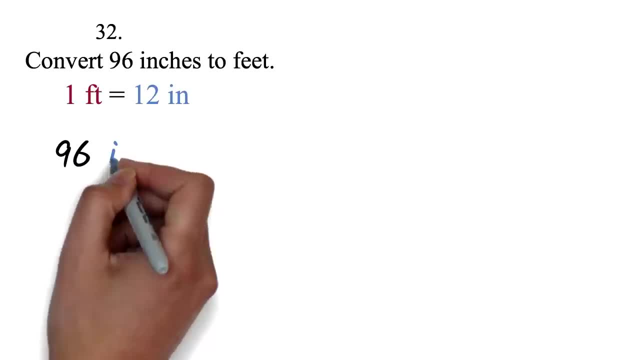 you are converting, In this case 96 inches- Then you'll bring your conversion factor. You want to write it in a fraction form such that the inches will cancel out. You basically want the bottom factor to be the same as the value you're converting, so you can cancel. 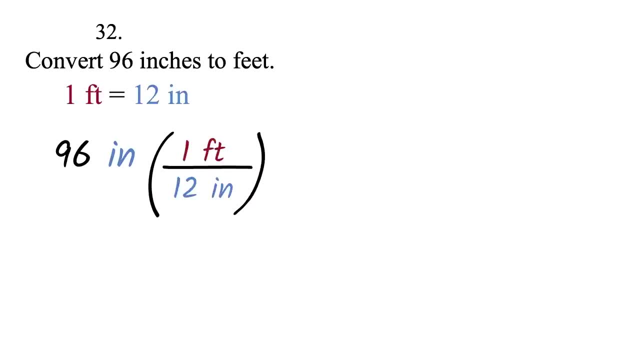 Here we will write 1 foot over 12 inches. The inches can cancel out. We now have 96 times 1 foot over 12. This will give us 8 feet. So 96 inches is 8 feet. Let's take another example, Question 32b: Convert 6 feet to inches. We are given our. 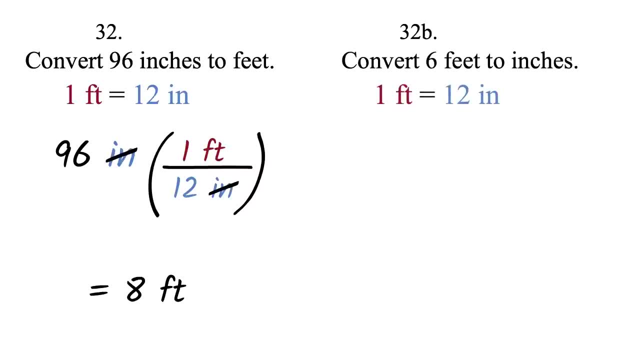 conversion factor. as 1 foot equals 12 inches, You'll first write down what you are converting, In this case 6 feet. Then you'll bring your conversion factor. You want to write it in a fraction form, such that the feet will cancel out. 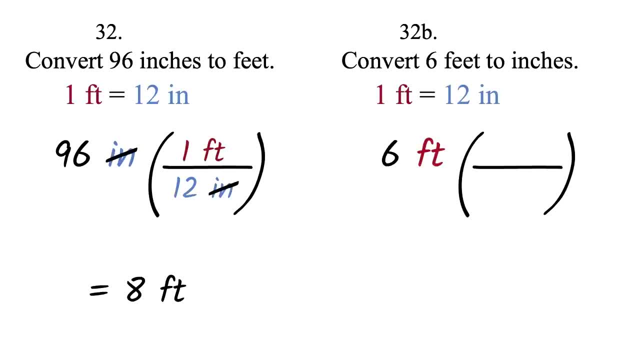 You basically want the bottom factor to be the same as the value you're converting, so you can cancel. Here we will write 12 inches over 1 foot. The feet can cancel out. We now have 6 times 12 inches over 1. This will give us 72 inches. So 6 feet is 72 inches. 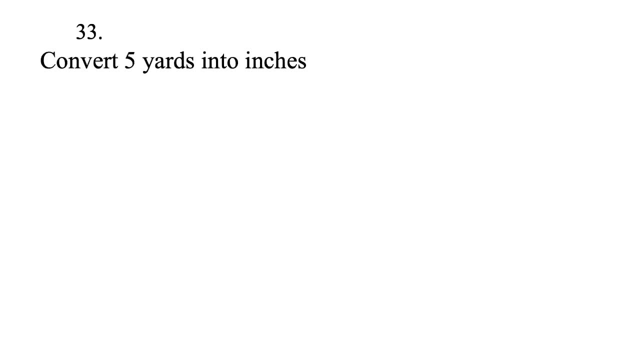 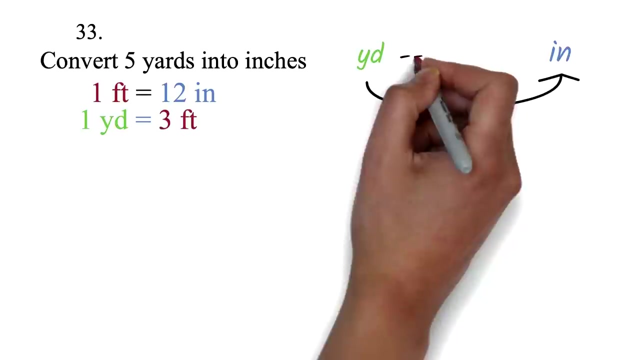 Convert 5 yards into inches. Given the conversion factors, 1 foot equals 12 inches. You can have questions in which you must use multiple conversion factors Here in order to convert from yards to inches. we have to convert from yards to feet first, then we will convert. 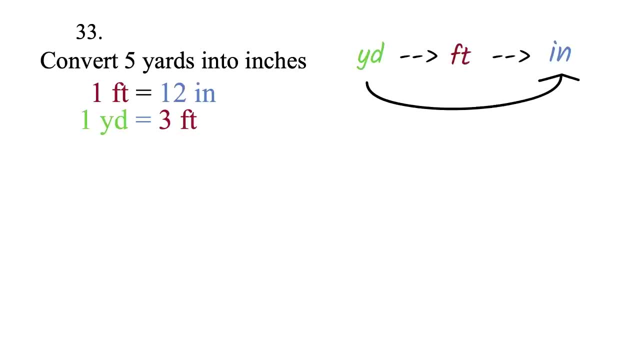 from feet to inches. Let's look at it As usual. we will write down what we are converting, In this case 5 yards. We multiply this by the converting factor 3 feet over 1 yard, The yard will cancel out. 5 yards equals 2 feet. This will give us 72 inches over 1 foot. You can have questions in which you must use multiple conversion factors. Here, in order to convert 5 yards into inches, we will write down what we are converting Here. in order to convert 5 yards into inches, we will write down what we are converting: 5 times 3 is. 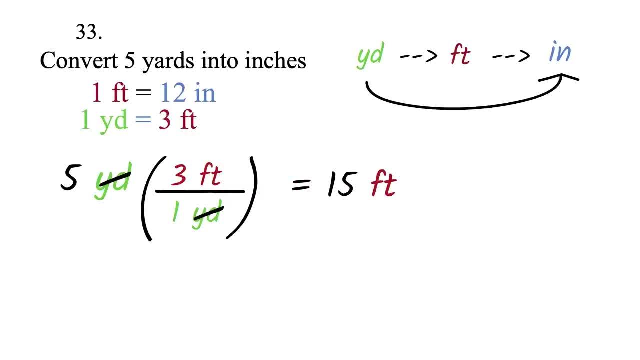 15.. So we have 15 feet. Now we have to convert the 15 feet to inches. We will multiply it by the conversion factor. 12 inches over 1 foot, The feet will cancel out. 15 times 12 is 180.. So the 5 yards we started with is 180 inches. You could have done this entire. 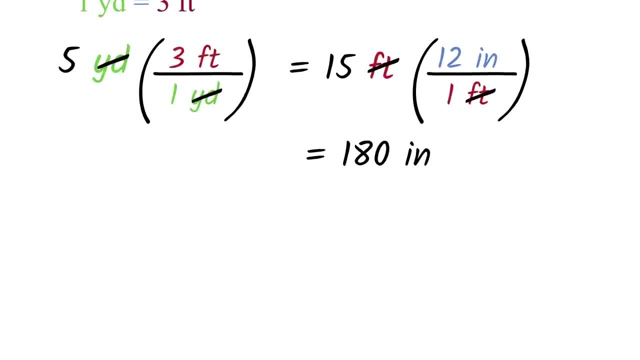 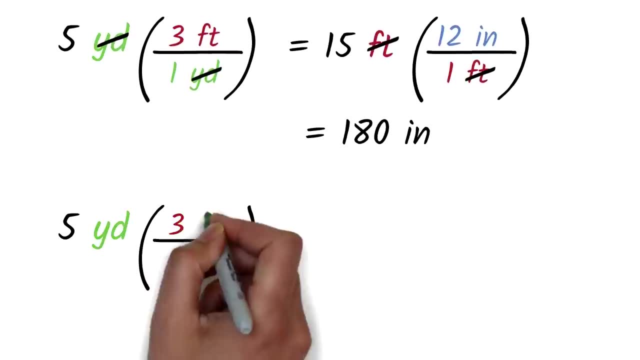 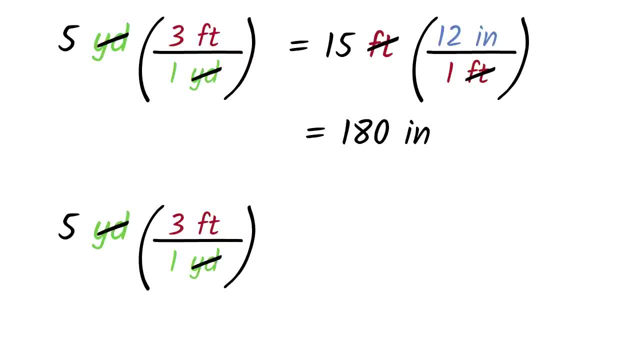 The yards will cancel out. Then we will multiply it by the second conversion factor: 12 inches over 1 foot, The feet will cancel out. We can see that we just have inches left. We compute this on our calculator 5 times 3 times 12. This will give us 180 inches as 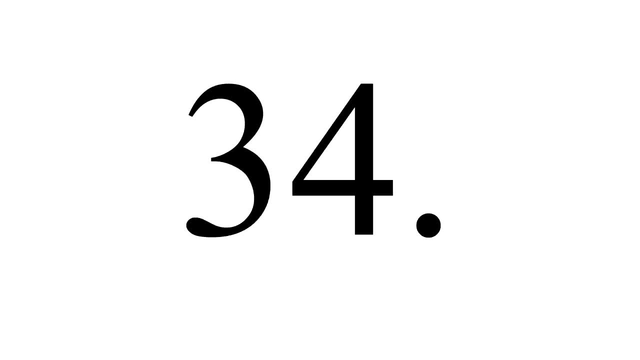 our answer: Find X and find Y in the diagram below. the work here is being able to identify that this is angles on a straight line. angles on a straight line adds up to 180 degrees. once you know that, you will just add everything and equate it to 180. then 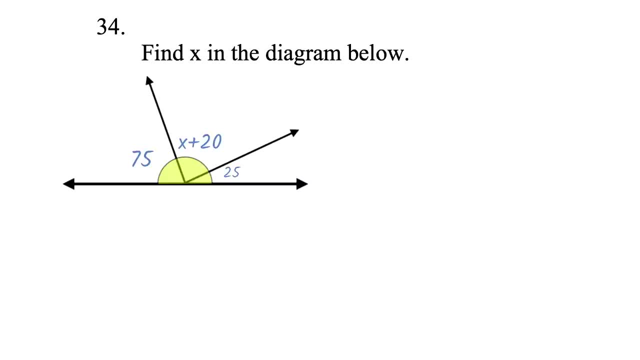 solve the resulting equation. so here we will add 75 plus X plus 20 plus 25 equals 180. we can add the numbers 75 plus 20 plus 25 to get 120, so we have X plus 120 equals 180. we can subtract 120 from both sides. the 120 will cancel out. 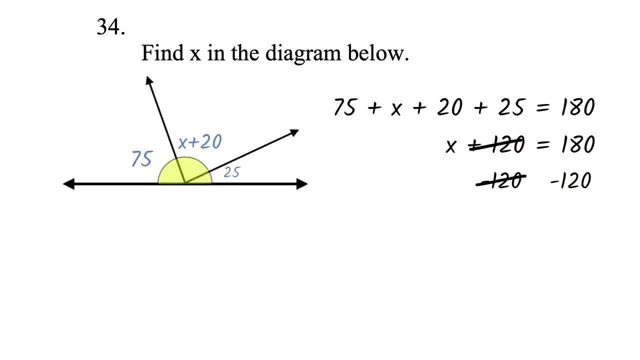 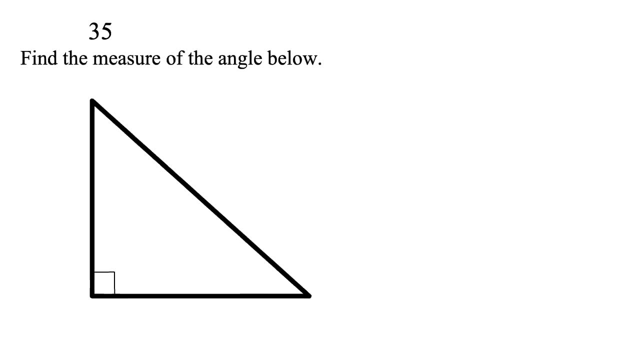 180 minus 120 is 60, so X is 60. find the measure of the angle below. here the first thing you have to identify is that this is a right triangle because of this mark here this means this angle is 90 degrees. we know that the sum of the interior angles 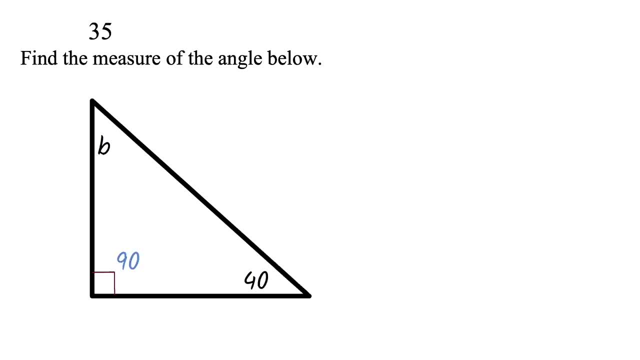 of a triangle is 180 degrees, so we can add 40 plus 90 plus B and this must be equal to 180. 40 plus 90 is 130. we have 130 plus B equals 180. one step equation: subtract 130 sides to get B equals 50 degrees. There's a faster way to solve this, but knowing. 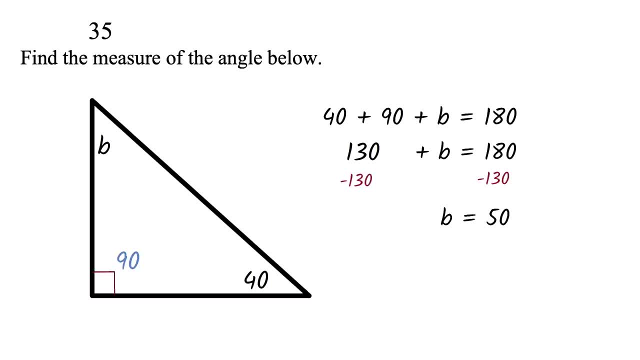 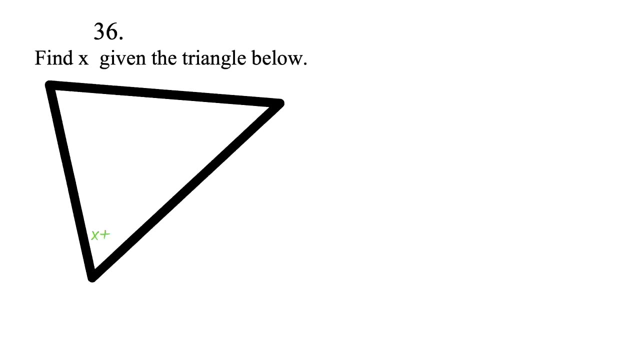 how to solve it by adding everything and equating it to 180 is so important I don't want to even teach any other way. This will ensure you get the answer correct, no matter the twist. Find X, given the triangle below. Questions like this is the reason why I 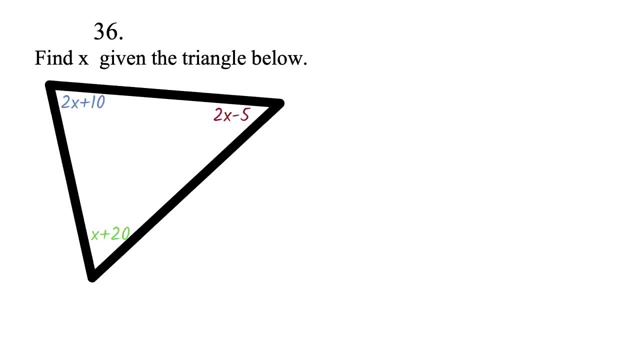 like the setup of adding all the interior angles and equating it to 180.. We add up the angles X plus 20 plus 2, X plus 10 plus 2, X minus 5 equals 180.. We add all the X terms 1 plus 2 plus 2 to get 5 X. Then we add all the numbers 20. 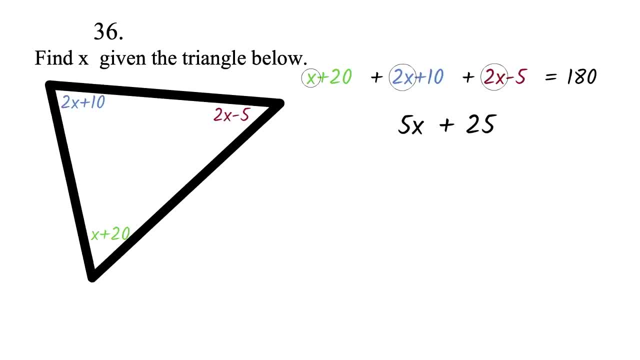 plus 10 minus 5 to get 25.. So we have: 5 X plus 25 equals 180.. We have a two step equation. We subtract 25 from both sides to get 5 X equals 155.. Then we divide both sides by 5 to get X equals. 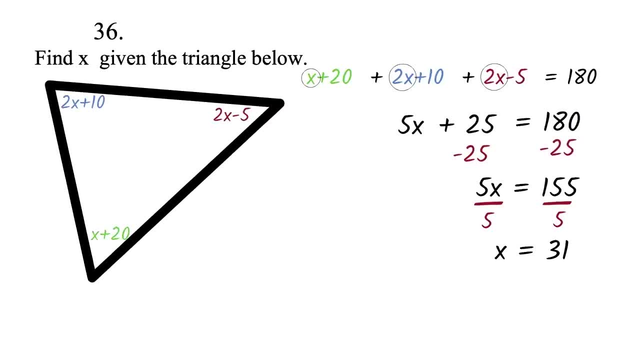 31.. We could have been asked to find the actual angles. In this case we would replace the X in each of the angles with 31.. So for the angle X plus 20, we will have 31 plus 20 to get 51 degrees here. For the angle 2, X plus 10. 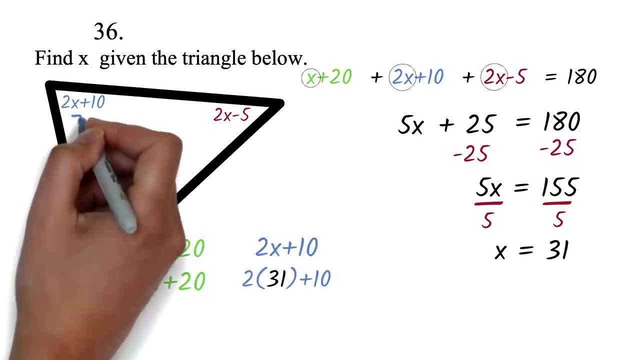 we will have 2 times 31 plus 10.. This will be 72 degrees. And finally, for the angle 2x minus 5, we will have 2 times 31 minus 5.. This will be 57 degrees. We can. 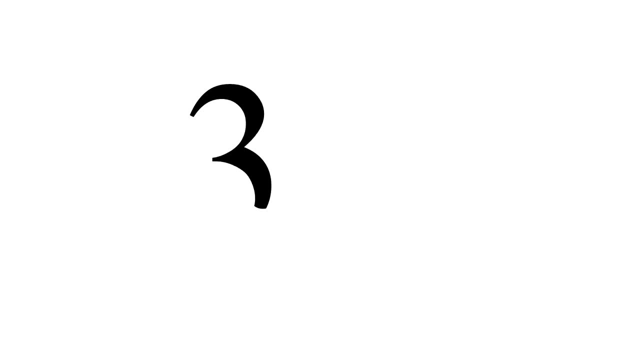 see that when we add these three values we will get 180.. Find the angle X below. You can have questions in which you'll need to use other properties of straight lines to get the interior angles of the triangle. The two most common ones are vertical angles and angles on a straight line. 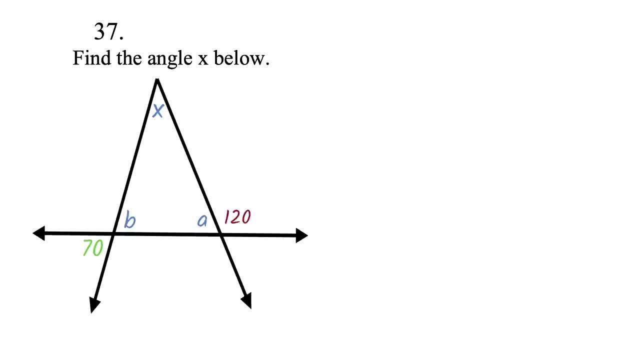 We've already done both In this question. we can find angle B using the idea of vertical angles. We know that vertical angles are equal, So if this angle is 70 degrees, then the opposite, angle B, will also be 70 degrees. To find angle A, we 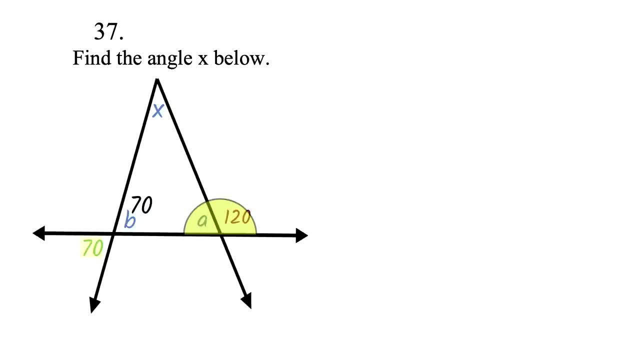 know that this is a straight angle. Angles on a straight line must be equal to 180 degrees. So if this is 120 degrees, then A will be 60 degrees. 60 plus 120 is 180. Now we add all our interior angles and equate it to 180. We have 70 plus 60 plus X equals 180.. I'm 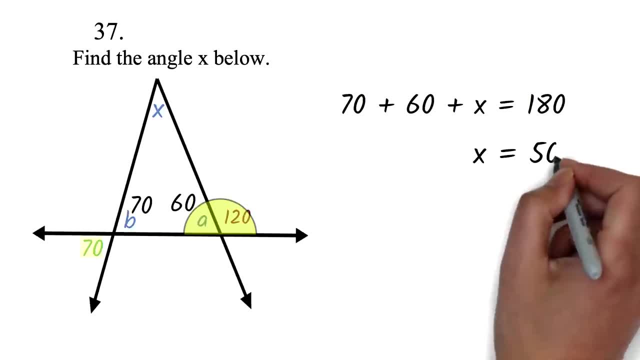 sure you can do this by now. We solve it to get X equals 50 degrees. There's another way we could have solved it Once we knew the angle B is 70. In a triangle, the exterior angle is equal to the sum of the two opposite interior angles. So in this, 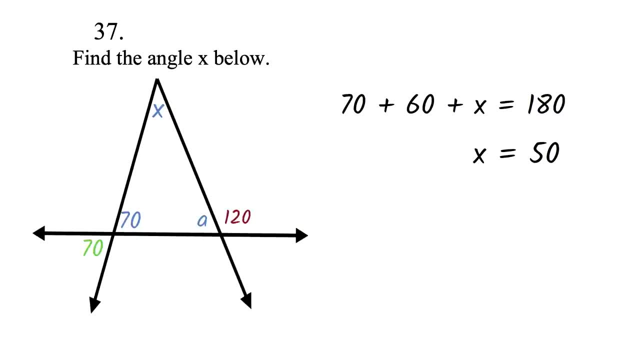 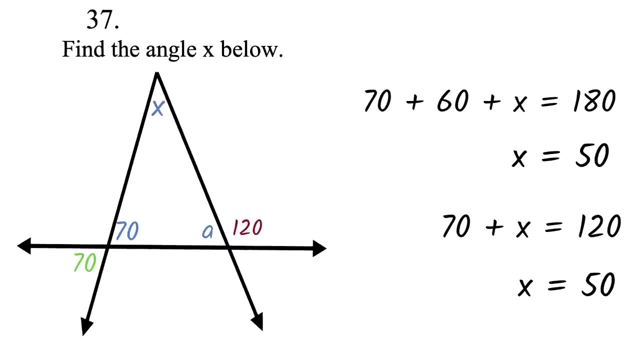 figure. the exterior angle 120 is equal to the sum of the two opposite interior angles, That's X and 70. So we can write: 70 plus X must be equal to 120.. We solve for X to get X equals 50 degrees. Notice we got the same answer. 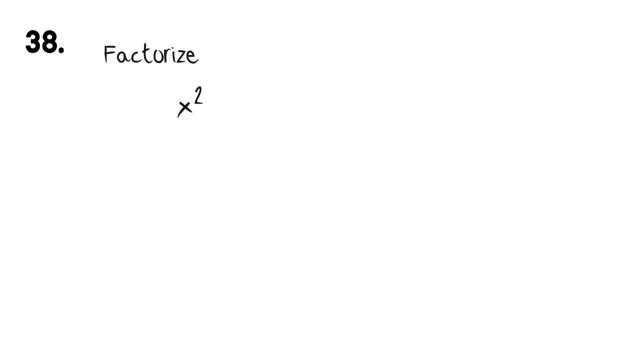 Question 38.. We are factoring the quadratic X squared minus 5X minus 6.. In question 17, we multiplied two binomials to get one trinomial. The idea of factorization is basically reversing the process, Finding out what multiplied to get X squared minus 5X minus 6, you will find. 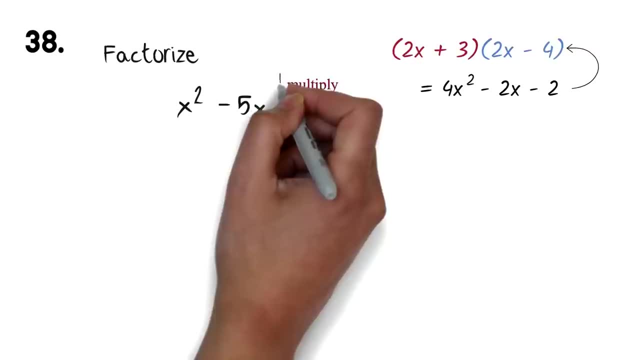 two numbers that multiply to get the constant, In this case the negative 6.. The two numbers must also add up to get the coefficient X squared minus 5X minus 6.. In this case the negative 6.. The two numbers must also add up to get the coefficient X squared minus. 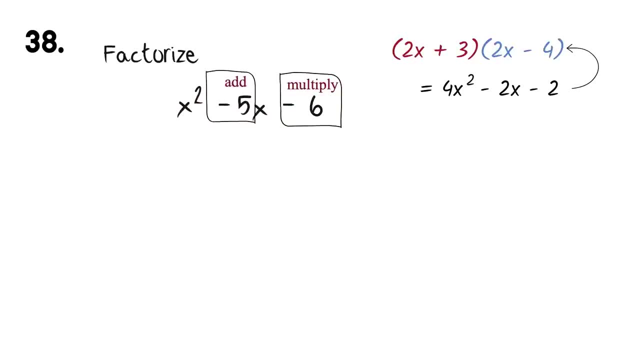 6. The two numbers must also add up to get the coefficient of the X, which is negative 5.. This takes some trial and error and depends mainly on how good your multiplication is. The two numbers here will be negative 6 and 1.. Negative 6 times 1 will be negative 6.. 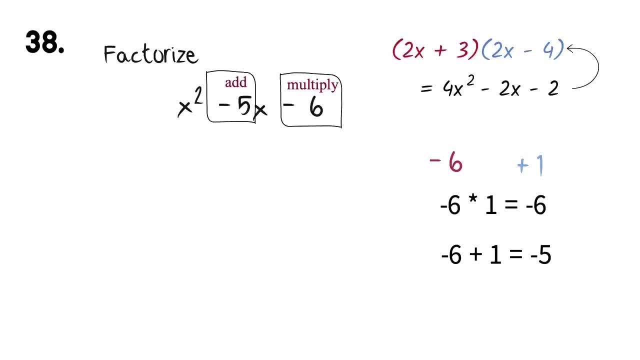 Negative. 6 plus 1 will be negative 5.. After finding these numbers, all you'll do is to put them in parenthesis with the X, and you are done. So we have X minus 6 and X plus 1.. Question 40.. 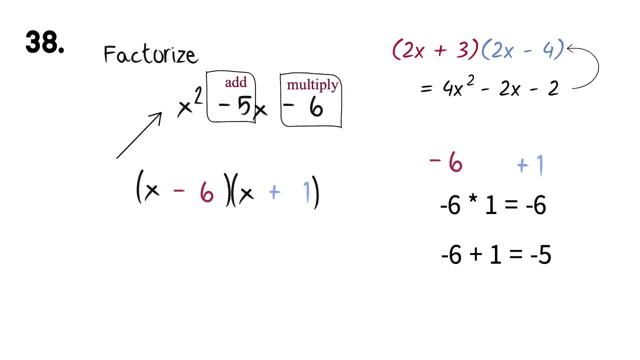 only if there's no number in front of the x squared. In math we say the coefficient of the x squared is 1.. Please check out ultimategetcom for other cases of factoring and factorizations. Here we are supposed to find the area of the green shaded portion. 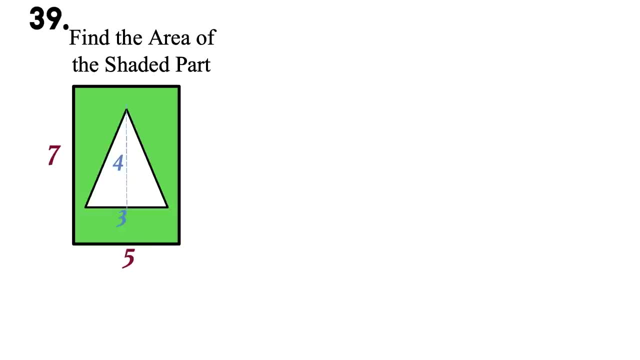 Questions like this is also very common. The work here is to find the areas of the two shapes and subtract it. We starts by finding the area of the rectangle. This is the length times the width. So we will have 5 times 7, which is 3 to 5.. 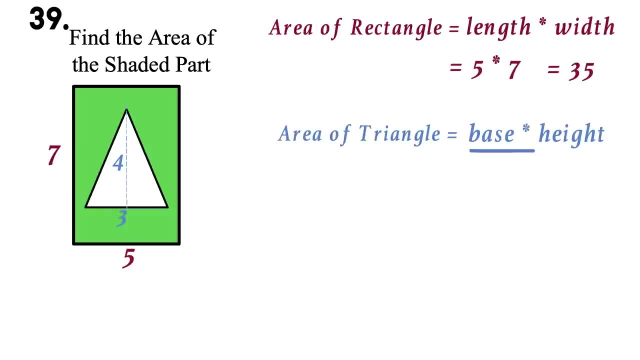 Next we find the area of the triangle. We know that it's the base times the height over 2.. The base is 3 and the height is 4.. We have 3 times 4 divided by 2. This will give us 6.. 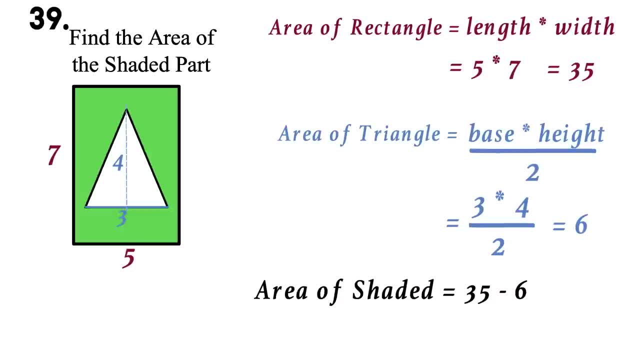 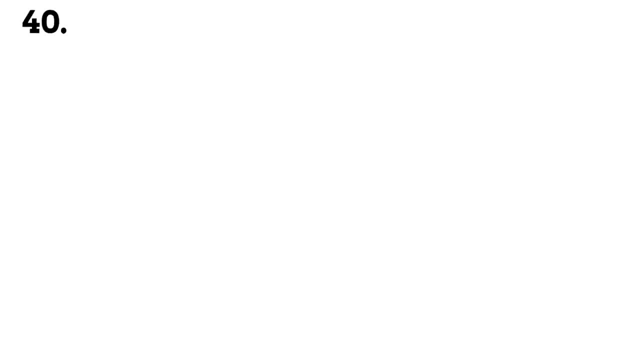 So the area of the shaded portion will be 3 to 5 minus 6. This will be 29.. We are looking at a similar problem. We want to find the area of the green shaded portion. Again. all we have to do is to find the areas of the two shapes and subtract them. 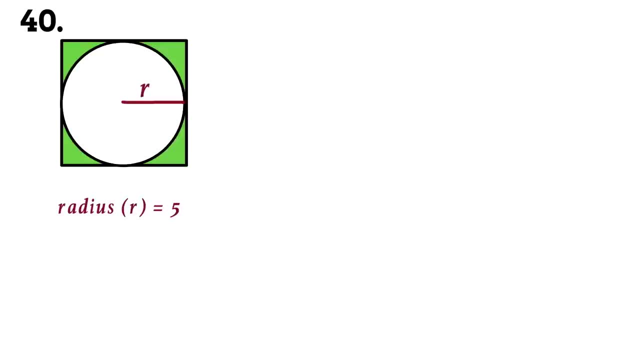 Here we have a circle of radius 5 inscribed in a square. The formula for finding the area of a circle is pi times r squared, Where r is the radius. So we have 5 squared times pi. This will give us 25 pi. 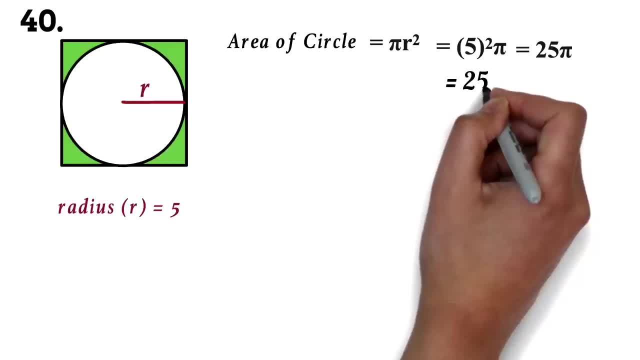 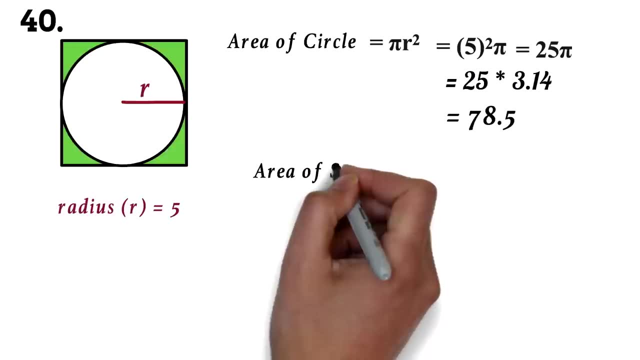 The value of pi is approximately 3.5.. So we have 5 squared times pi. This will give us 3.14.. So we have 25 times 3.14, which is 78.5.. Now we find the area of the square. 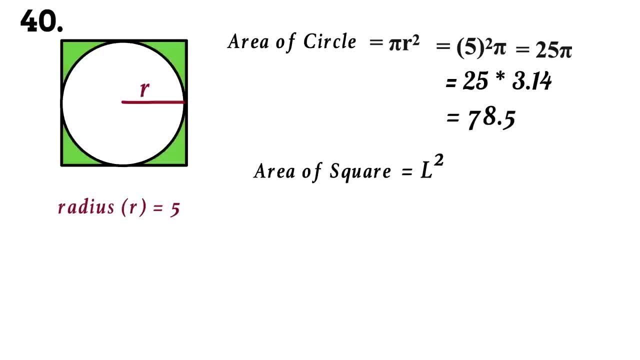 The area of a square is the length squared. We have not been given the length, but we can find it Since this is the radius. if we extend it to touch the other side of the square, we will have the diameter. The length of the diameter will be the same as the length of the square. 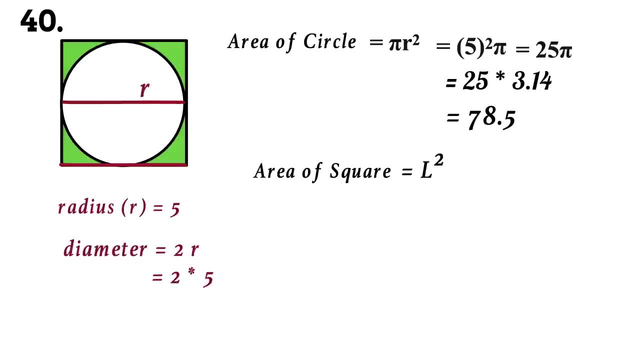 The diameter is 2 times radius, which is 2 times 5.. The diameter is therefore 10.. So the length of the square is also 10.. Now we find the area. The area will be 10 squared. This will give us 100.. 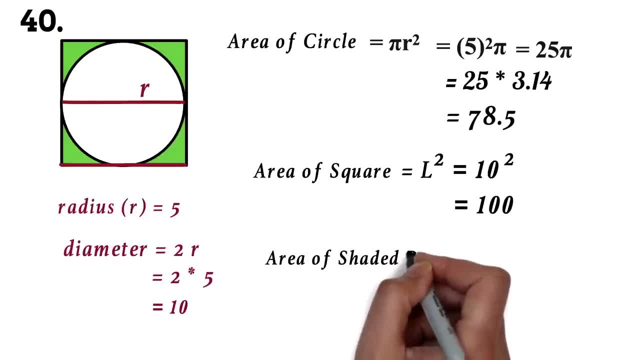 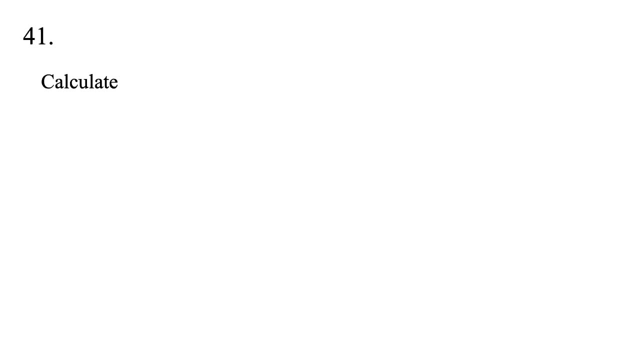 Finally, we subtract the two areas to get the area of the shaded portion, We have 100 minus 78.5.. The area of the shaded portion is therefore 21.5.. Question 41.. Calculate 28.5.. 2 exponent negative 3 times 16.. 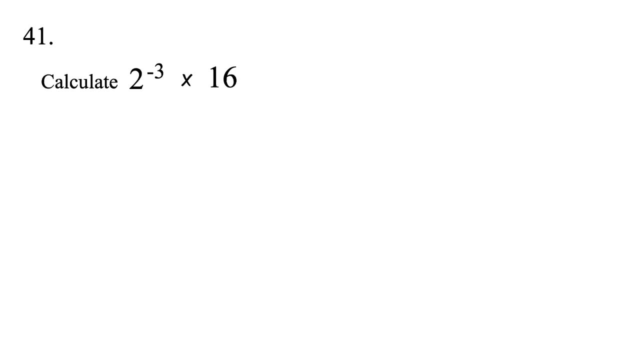 Do not use a calculator. This was the first question on our GED Math 2021 video and most students weren't able to solve it because they were not familiar with negative exponents. so let's look at it here. We'll be solving it two different ways. 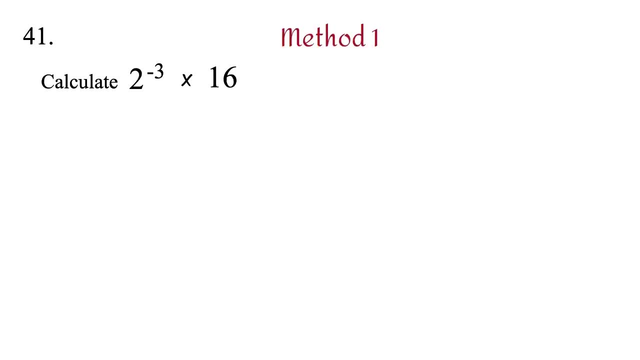 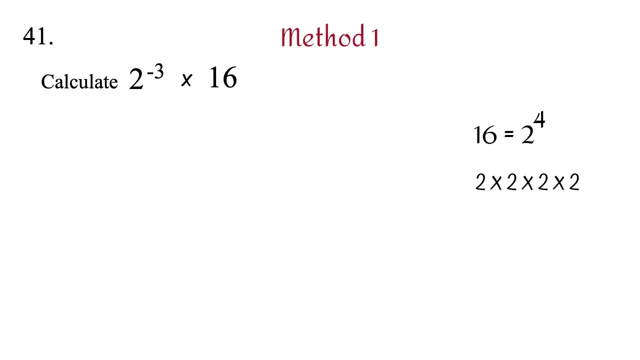 Once you know that, then you can replace the 16 with 2 exponent 4.. Now we have 2 exponent negative 3 times 2 exponent 4.. In math, if you have two numbers multiplying and the bases are the same, you can simply: 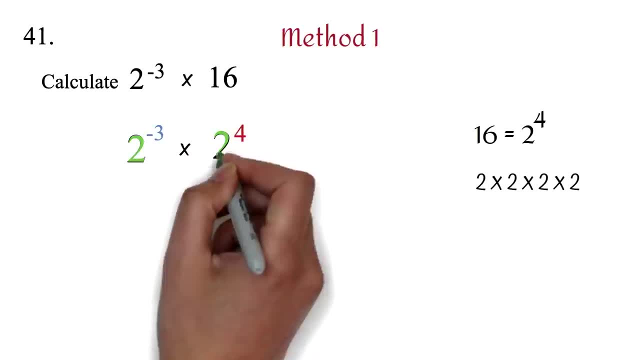 add the exponent. They both have the base of 2, so we can simply add the exponents. So here we will have 2 exponent. negative 3 plus 4.. Negative 3 plus 4.. Negative 3 plus 4 is the same as 4 minus 3, which is 1, so we have 2 exponent 1.. 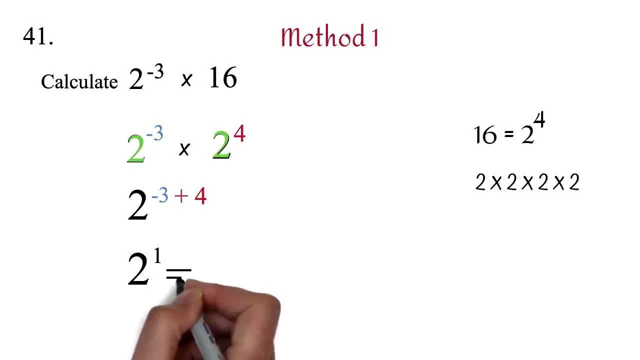 Any number, exponent 1 is the same number. so 2 exponent 1 is simply 2.. This is our answer. Let's look at method 2.. Method 2.. First, we have to know that we can move a number with an exponent from the numerator. 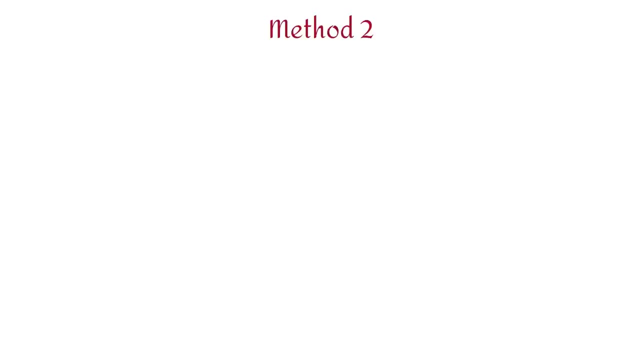 to the denominator or denominator to numerator. We can move a number from the denominator to the denominator by changing the sign of the exponent. Example: if you have 2 times 7 exponent negative, 4 over 3, we can move the 7 exponent negative. 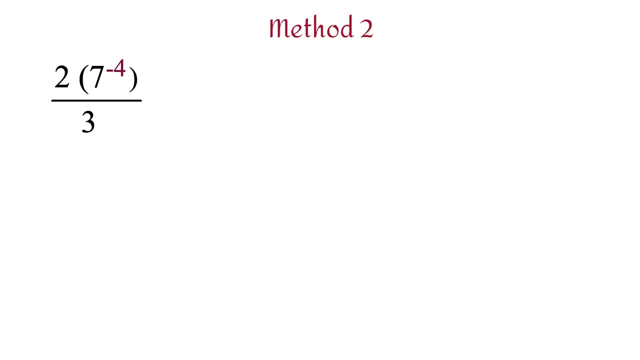 4 from the numerator to the denominator. If we do that we have to change the exponent negative 4 to exponent positive 4.. So we have 2 over 3 times 7 exponent positive 4.. The 7 exponent negative 4 in the numerator became 7 exponent positive 4 in the denominator. 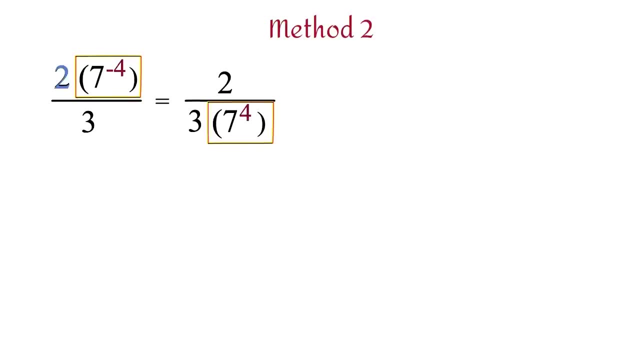 Then we have to move the 2 exponent negative 4 over 3 to the denominator. Notice that there's this 2 in the numerator and 3 in the denominator. If you are not given any values in either one or both, you can use one. 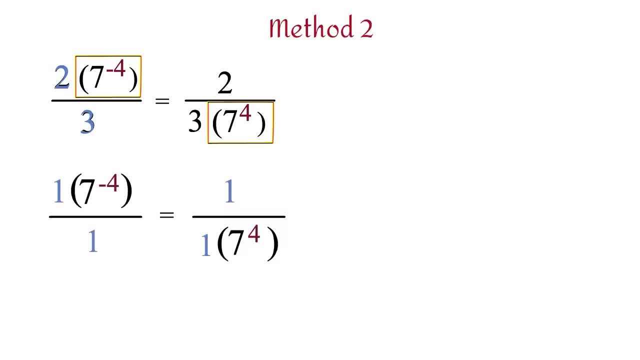 This is not a necessary step, but can serve as a guide. Let's go to our question. We have 2 exponent negative 3 times 16.. Here we do not have a denominator, so we can use 1.. So we'll have 2 exponent negative 3 times 16 over 1.. We know we can move the 2 exponent negative 3 times 16 over 1.. So we'll have 2 exponent negative 3 times 16 over 1.. We know we can move the 2 exponent negative 3 times 16 over 1.. 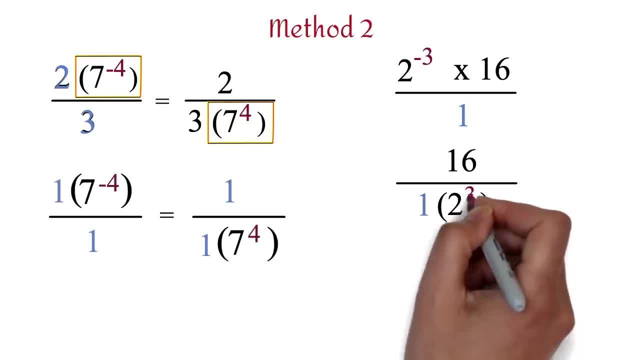 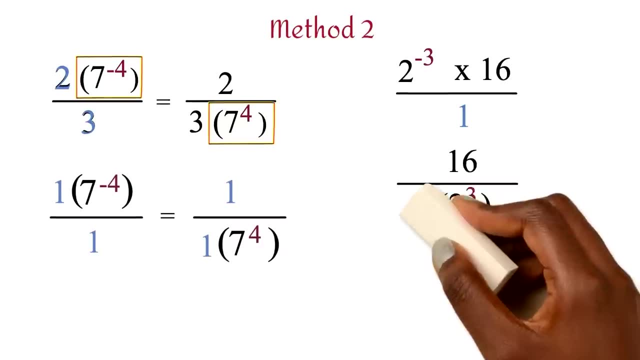 3 to the denominator to become 2 exponent 3.. Notice that the exponent negative 3 became exponent positive 3.. 1 times 2 exponent 3 is simply 2 exponent 3.. So we have 16 over 2 exponent. 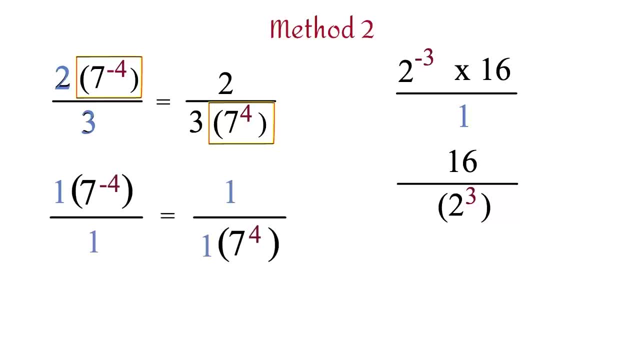 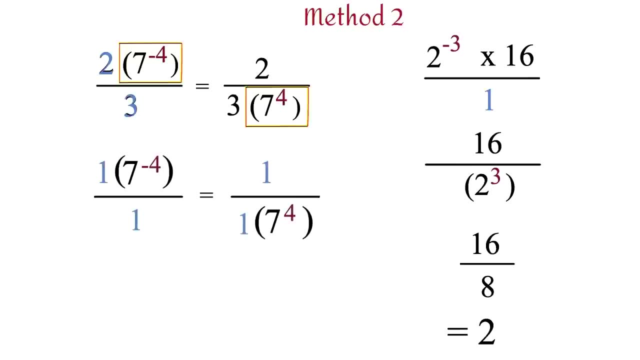 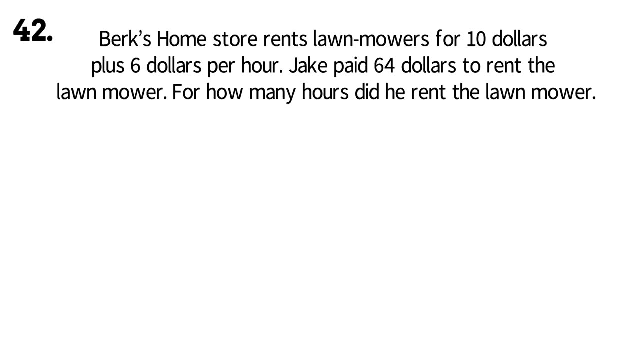 3.. 2 exponent 3 is 2 times 2 times 2,, which is 8.. We have 16 divided by 8.. This will give us 2 as our final answer. Burke's Home Store rents lawnmowers for $10 plus $6 per hour. Jake paid. 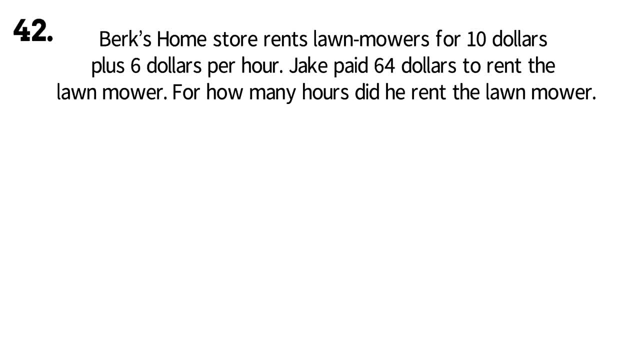 $64 to rent the lawnmower. For how many hours did he rent the lawnmower? This is also another very common kind of two-step GEDs word problem. Here all our three values are in dollars, So you have to find the group in a different way. I call it the revolving. So again we will have our total. 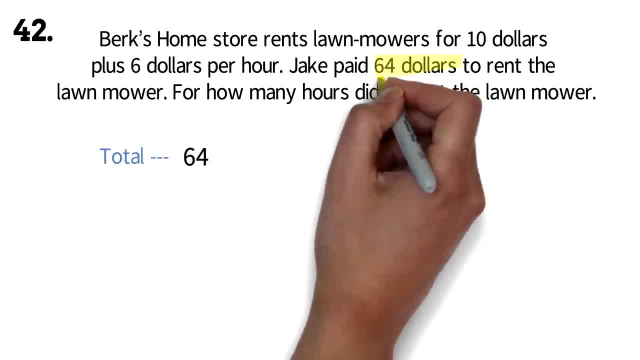 Here the total is $64.. This is the total amount of money Jake paid for the lawnmower. The group, which we are calling the revolving, is the value that keeps happening, usually per day or per hour or each day or something like that is with it. So here, 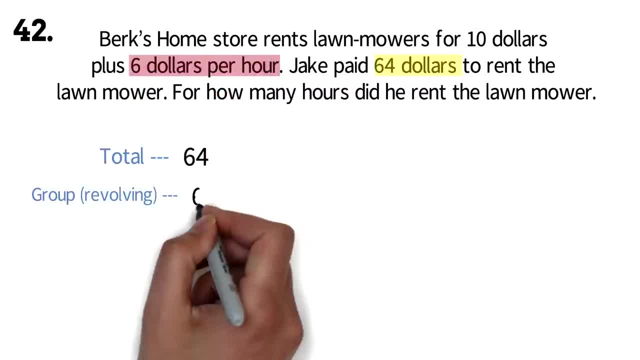 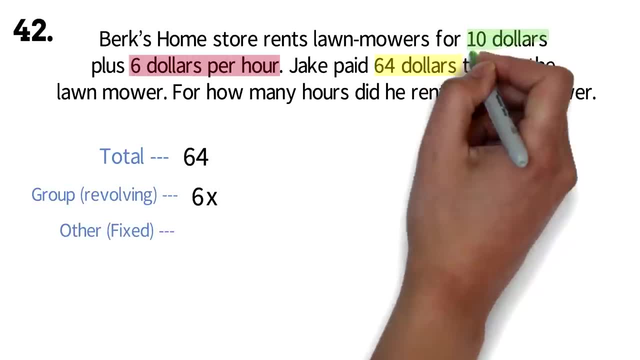 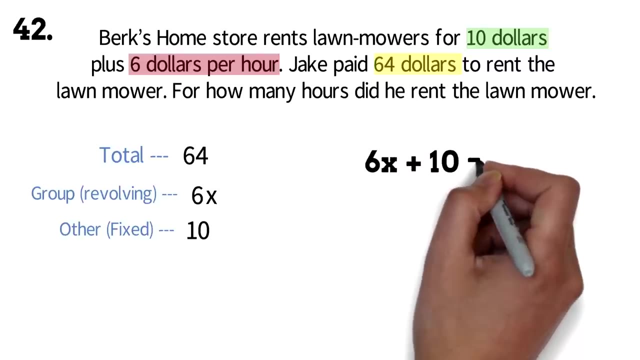 we have $6 per hour, So this will be 6.. We also know the group has the X. Finally, we have what is left, or the fixed value. Here it is $10.. We can write the two-step equation for it. We have: 6X plus 10 equals 64.. 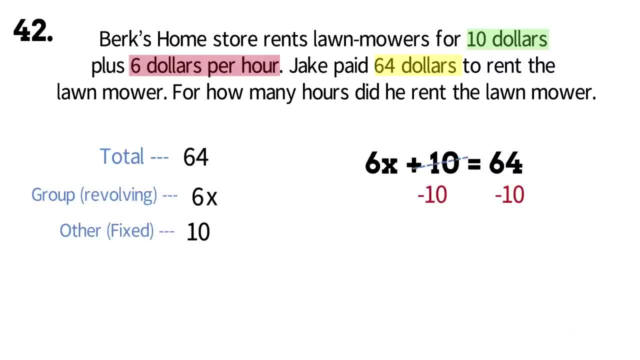 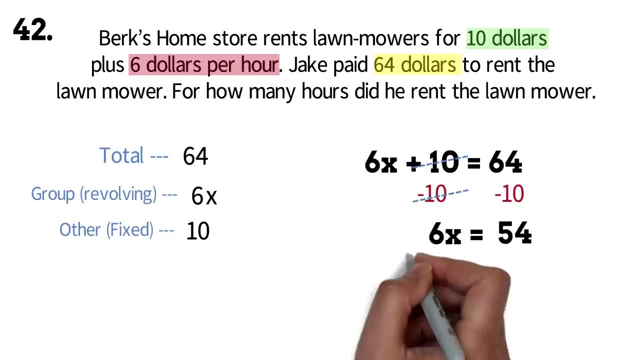 We subtract 10 from both sides, The 10 will cancel out. 64 minus 10 will be 54. So we have 6X equals 54. Next we will divide both sides by 6.. This will cancel out. 54 divided by 6 is 9.. Therefore, 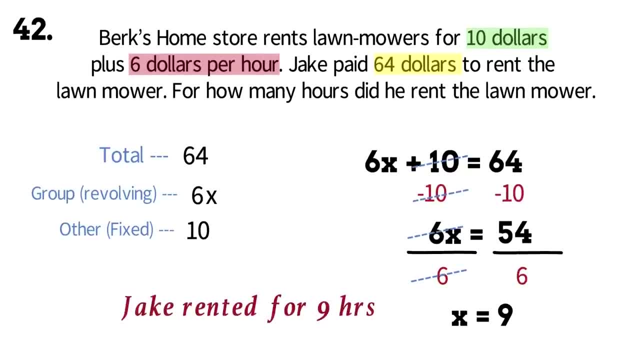 X equals 9.. So Jake rented the lawnmower for 9 hours. Please, you don't have to write all these on the GED test. We are using it for teaching purpose. You can just identify your total, fixed and revolving values and solve the resulting two-step equation. 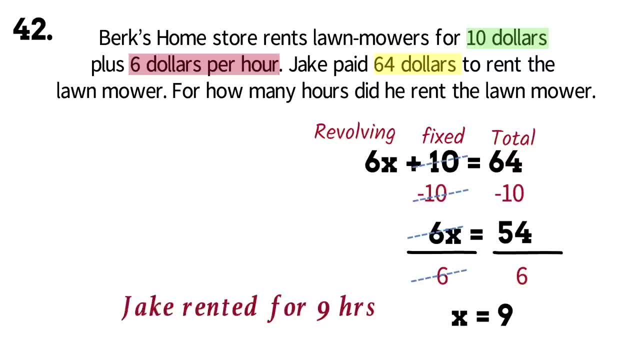 Also, if you know what you're doing, you could have solved this in less than 10 seconds. Input 64 minus 10 divided by 6 on your calculator to get 9 as the answer. What we did was the total: The total minus the fixed divided by the revolving. 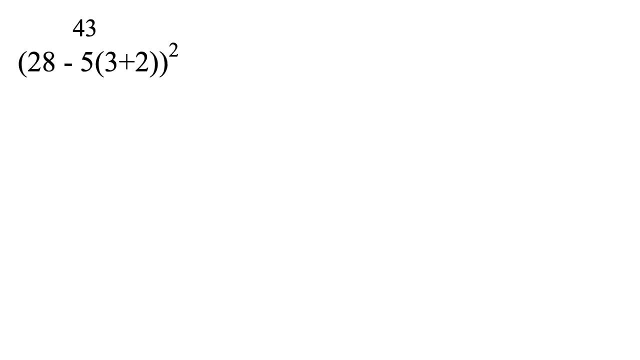 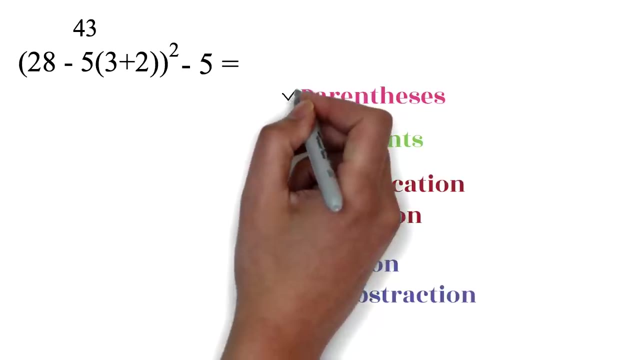 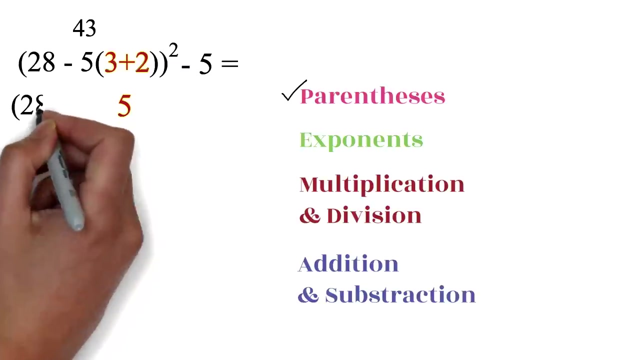 We are supposed to calculate this without using a calculator. Let's bring our order of operations Again. we will perform the operations within the parenthesis first. We notice that there's parenthesis within parenthesis. In this case, we will perform the inner one first. So we have 3 plus 2 to get 5.. We now have parenthesis: 28 minus 5 times 5,. 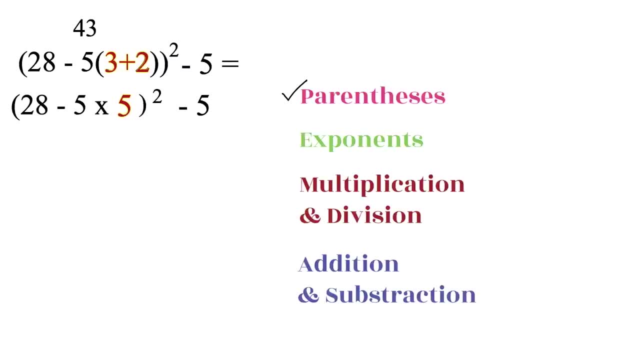 all squared minus 5.. Using the order of operations, we have to perform the operation in parenthesis. We'll notice that the operation in parenthesis also has multiple operations, That's subtraction and multiplication. We will use the order of operation to work that out. 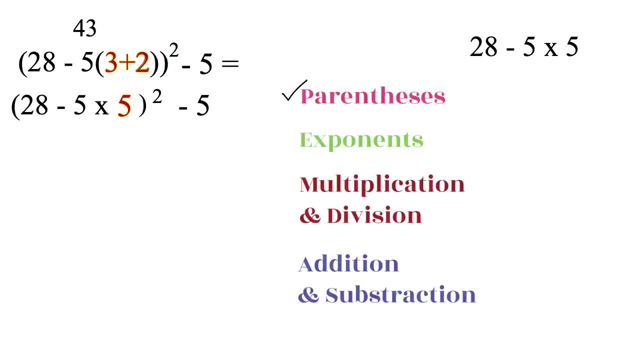 We know we have to do multiplication before subtraction. So we have 5 times 5,, which is 25.. Then we have 28 minus 25,, which is 3.. Now all of these has been simplified to 3. We now have 3 exponent, 2 minus 5.. 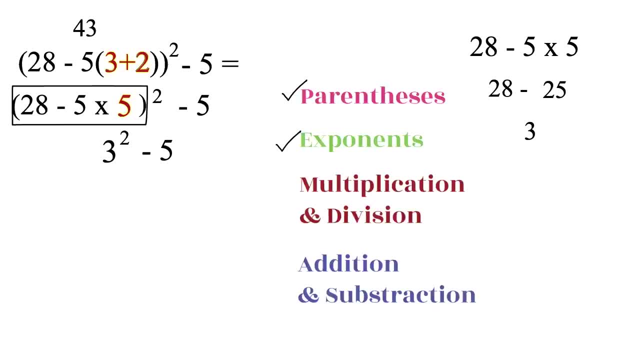 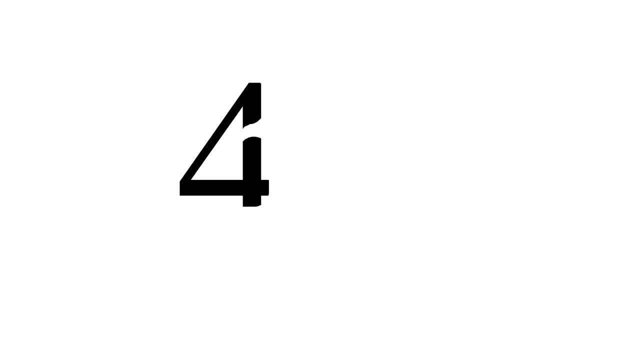 From the order of operations. we will do the exponent next 3. exponent 2 is 9.. We have nine minus five. Finally, we will do the subtraction. Nine minus five is four, so we have four as our final. a car travels at a speed of 60 miles per hour. if it travels at that speed for five hours, what will?